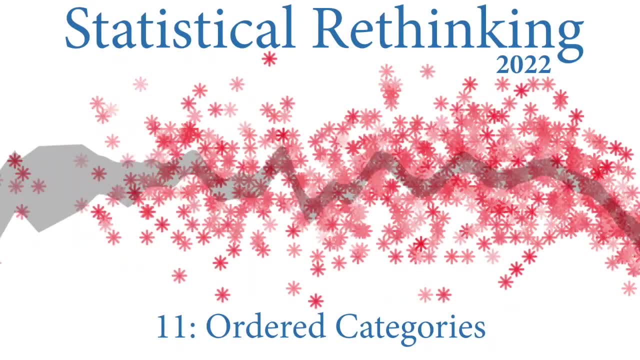 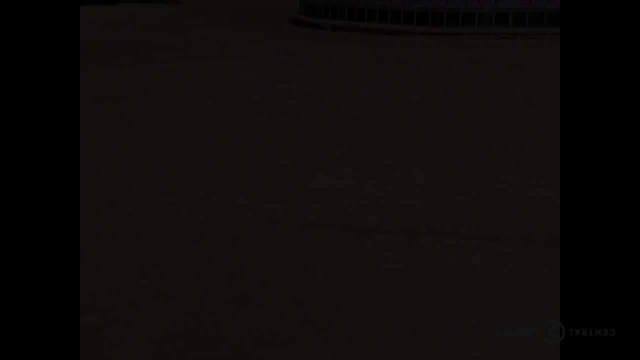 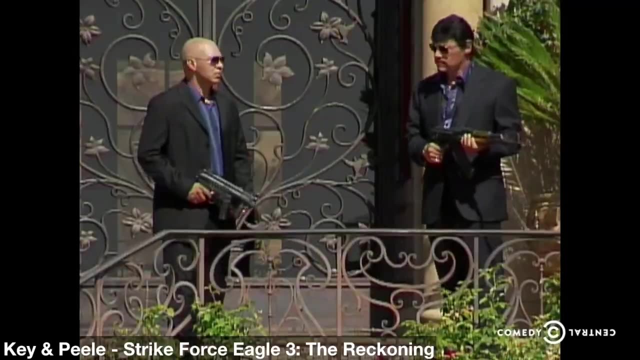 Even though statistics is undoubtedly a difficult subject, the examples in statistics courses often come across as unrealistically simple. It's a bit like those action movies where everything's in exactly the right place. the henchmen and the villains are inconceivably dumb. 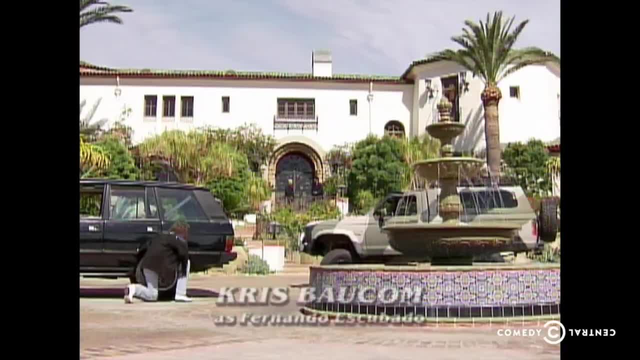 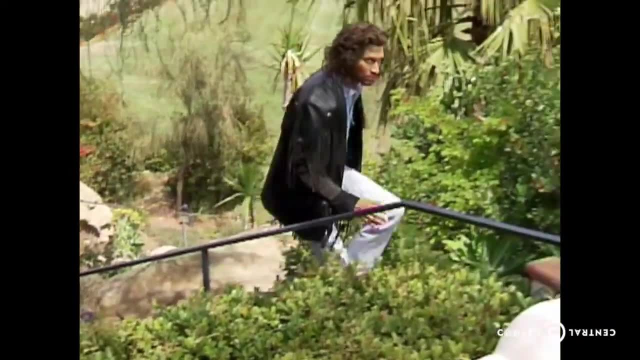 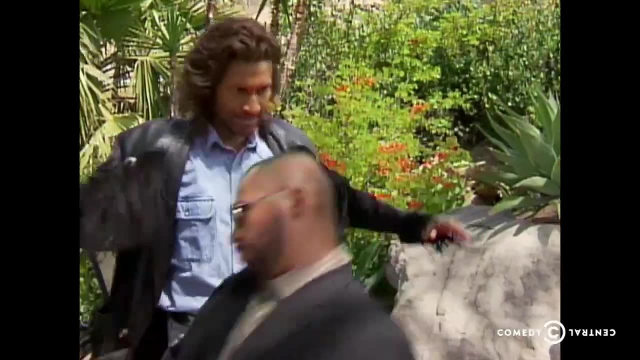 and careless and unskilled. The examples in statistics courses put up simple obstacles which are easily overcome just by the application of simple expedient techniques. It's as if the course is meant to convince you that if you just know the right test or the right commands, 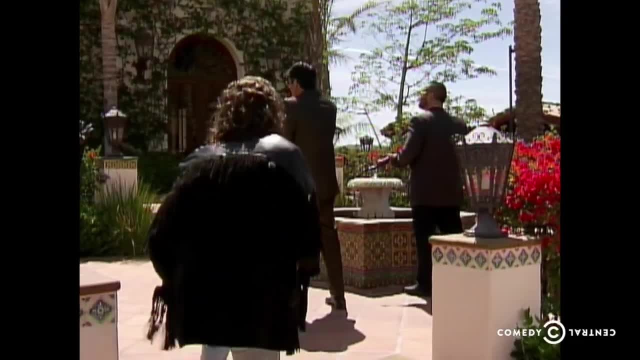 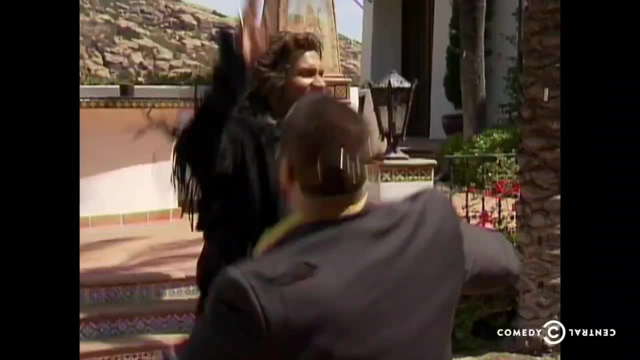 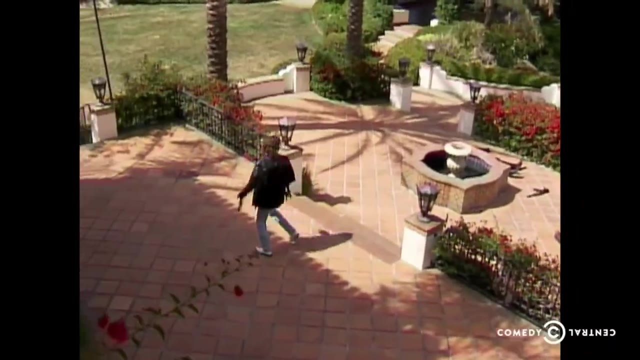 you can always get the answers you want and overcome seemingly deadly scientific obstacles. Of course you know it's not like that. Real research, the real sorts of data sets we contend with, put up a fight. They have more complexity, they have missing values, measurement error and then, of course, 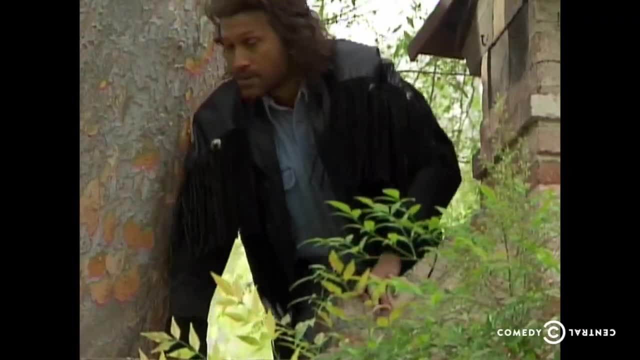 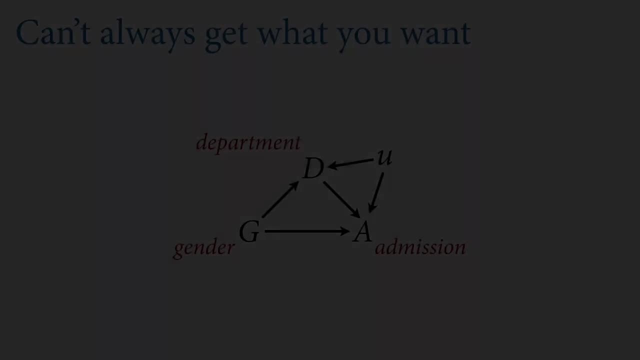 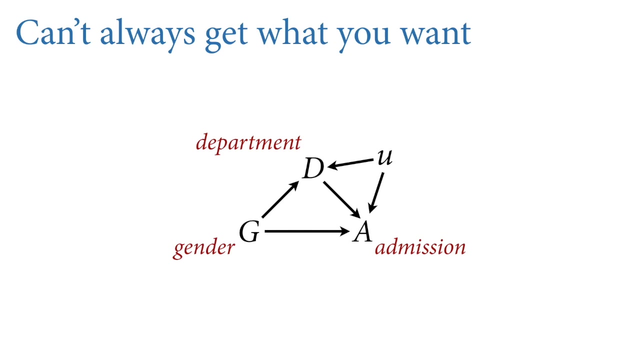 it's the conceptual structure underneath them that's the real challenge. So when we face real data sets, then we meet real terror. In this course I'm trying simultaneously to make the material learnable and also to give you a sense of that complexity. 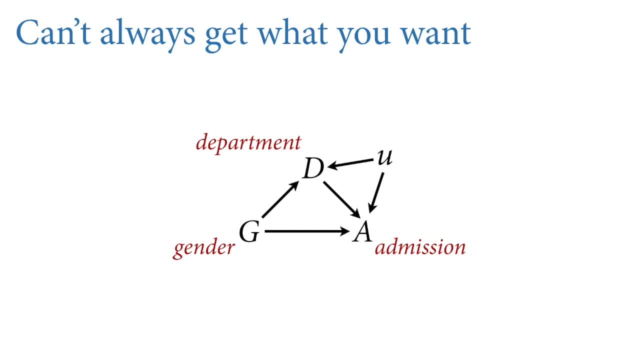 About what real statistical villains are like, not the trivial ones we see in action movies. So the example that motivated last week, this example of gender discrimination in graduate school admissions in the 1970s, is an example where we don't get what we want in the end, But it's a very 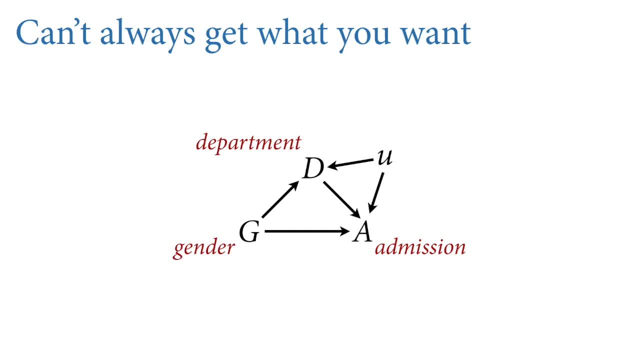 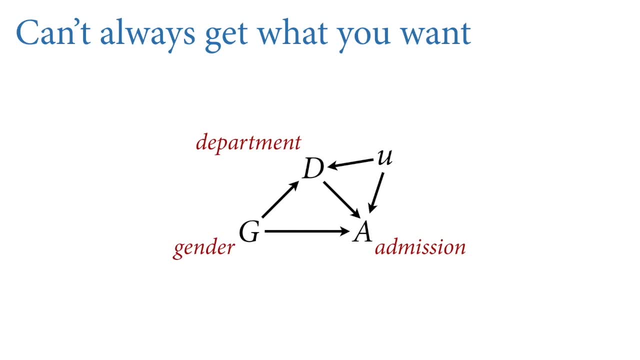 It's not, It's not, It's not, We can't. Um comes together because there are some standard regression tools, uh, but we can't. So let me remind you, Uh, what we can estimate, uh, under the general and reasonable assumptions of the example. 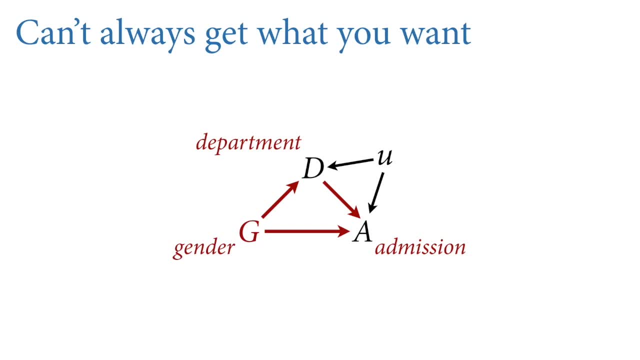 is the total effect of gender on admissions, But this is not what we want to know. What we want to know is the decomposition Uh into direct and indirect effects of gender on graduate school admissions. And this is plausibly and certainly confounded by unobserved 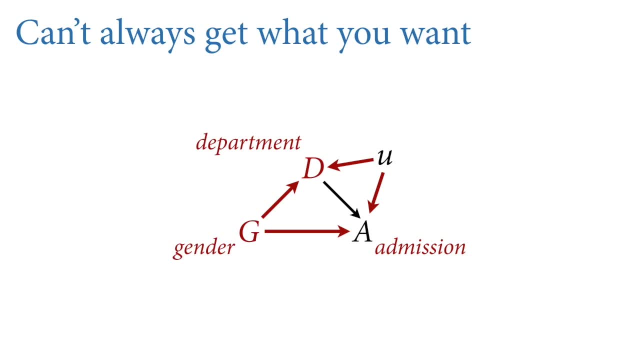 differences in the applications, that in the applicants that drive, both where they apply, whether they apply and affect their chances of admission. and this basic causal structure with a mediating path and a direct effect and plausible, unobserved confounds, is extremely common. lots of data analysis will have a structure like this. the lesson from this example isn't that inference. 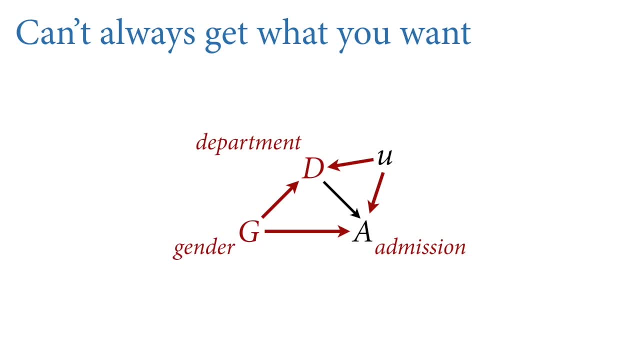 isn't possible. it's that one of the jobs of statistical education is to tell us when we can't get what we want, and that is an answer. it's in a very valuable answer because it stops us from wasting our time, other people's time and misleading policy. so it's a victory, even though we didn't get. 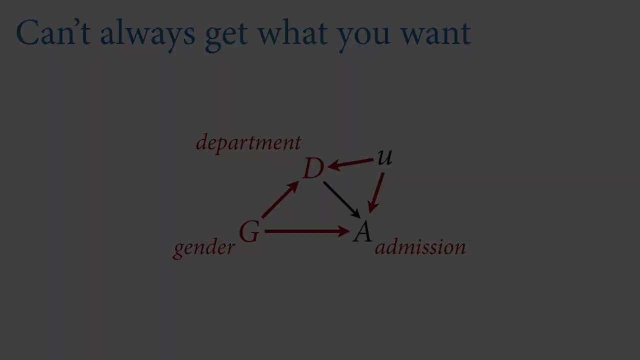 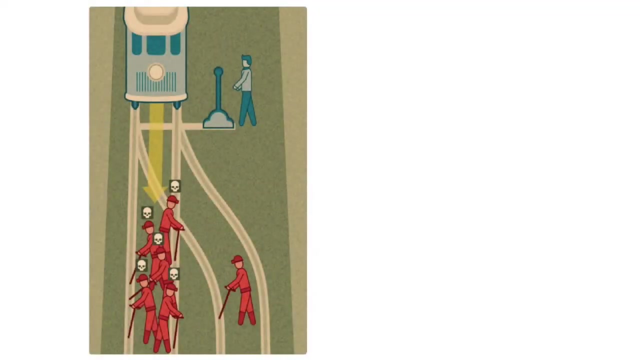 what we thought we wanted when we started. let's look at some other examples, and the example for this lecture is motivated by an interest in moral philosophy and moral psychology. so many of you will have heard of trolley problems, but for those of you who haven't, let me introduce you to them. so 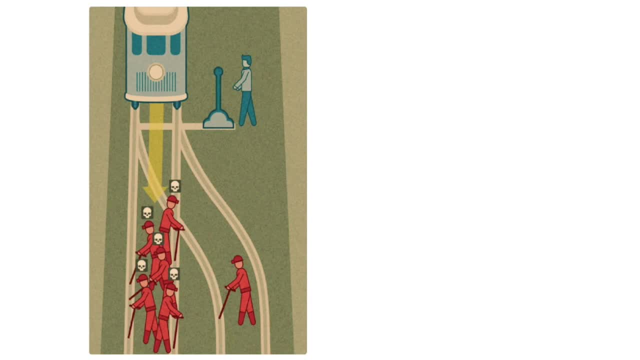 a trolley problem is a toy philosophical story that is meant to elicit moral psychology in those who listen to it. in the quintessential trolley problem the story goes: there's a runaway trolley on a track- seen at the the top of the illustration in this slide, and it's speeding out. 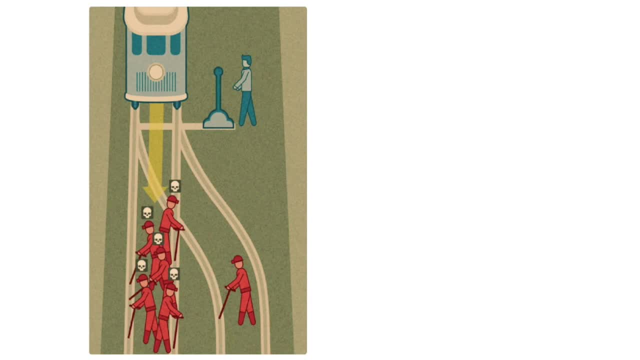 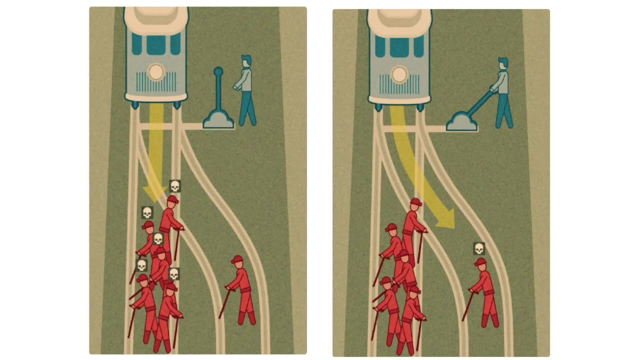 of control and it will strike five people who, for some reason, are on the track and unaware of it. however, you, the protagonists in this story- are standing next to a switch and if you pull the switch, it'll divert the trolley to a side track, where it will strike only one person. 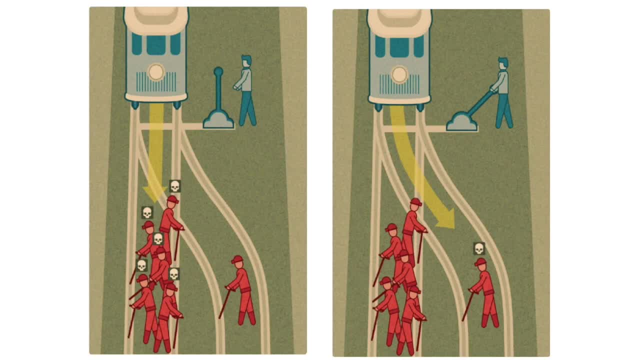 and now the question is, having heard this story, suppose the protagonist in the story pulls the switch- how permissible, morally permissible or appropriate is it to pull the switch? different people have different reactions to this story and there's a big empirical and philosophical and psychological literature trying to understand that variation. what are the intuitions, the moral? 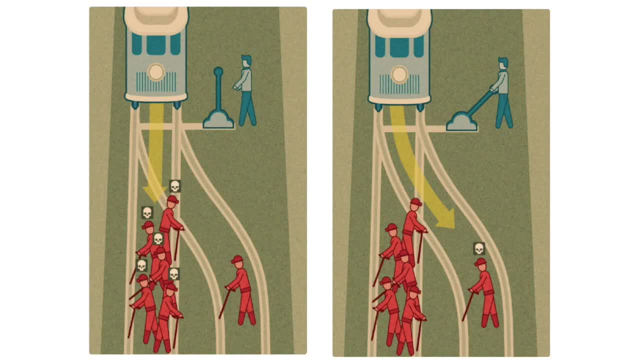 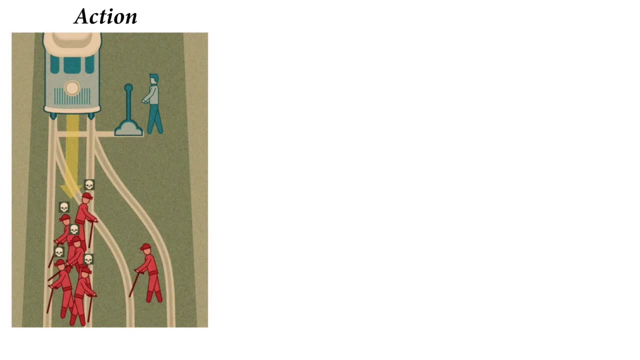 theories that lead people to different responses about these stories. the rest of this lecture we're going to focus on a large empirical data set that investigates three different principles that are hypothetically underlying people's intuitions, to things like trolley problems, to moral situations. these principles are action, intention and contact. 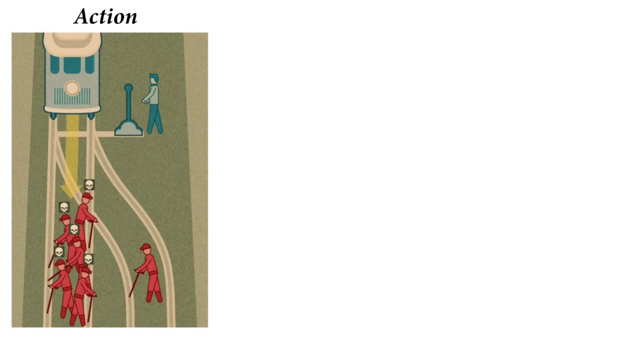 let me introduce each of them with a simple Trolley Story. so the action principle is in play in the Trolley Story. you already met the original Trolley Story. when the blue individual pulls the switch, it is his action that results in the death of the one. 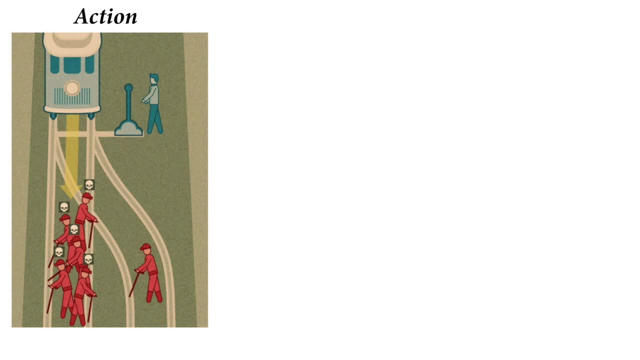 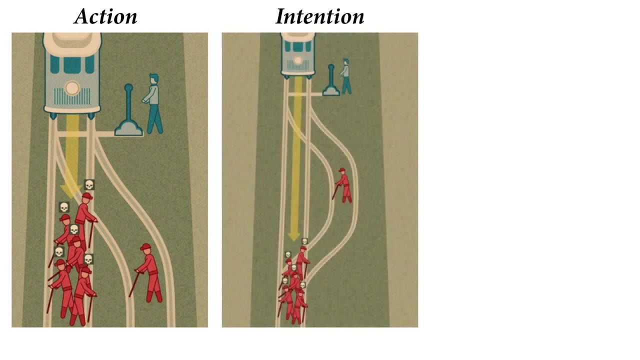 individual on the right, on the side track, and then we're asked to judge whether that action, rather than a lack of action, is morally permissible. the second principle is the intention principle. so now we have a modified trolley story in the middle. here there's a side track but it loops and reconnects to the main track. 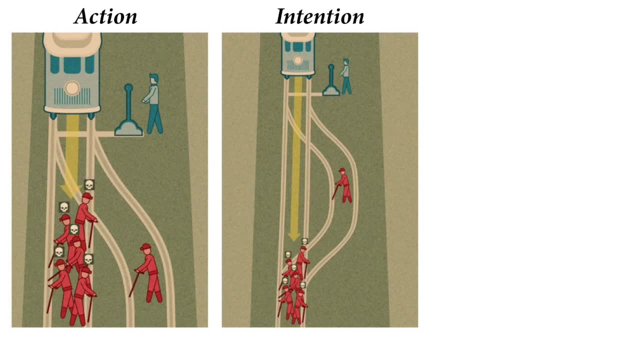 again. if you divert the trolley, it'll go on the side track and in the story, the, when the trolley strikes the one poor soul on the right, it will stop the trolley and save the lives of the five at the bottom again. but this time the death of the one person in the loop is intended. it's not. 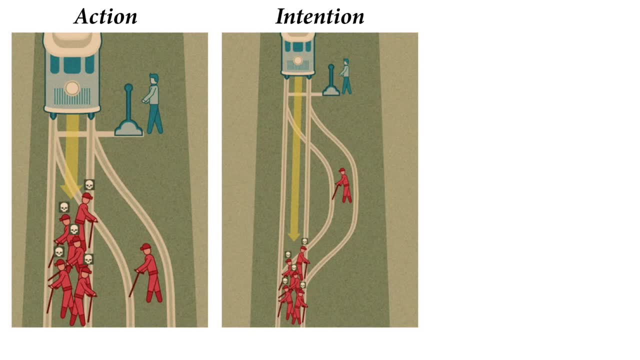 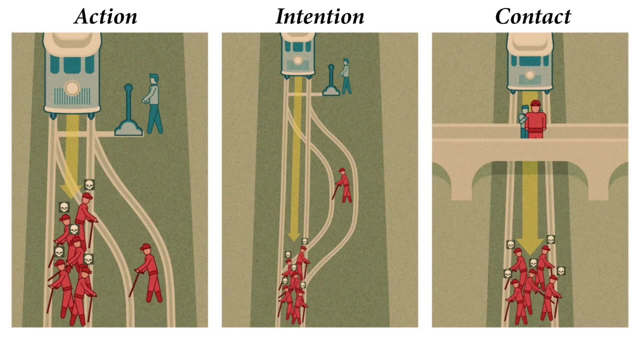 merely a side effect of saving the five lives, it's required to save the five flies, and this is called the intention principle, where a death is intended. and then, in those circumstances, how appropriate is it? and then the third principle is the contact principle. so here's another story. in this story, you are now not standing next to a switch, but you're on a 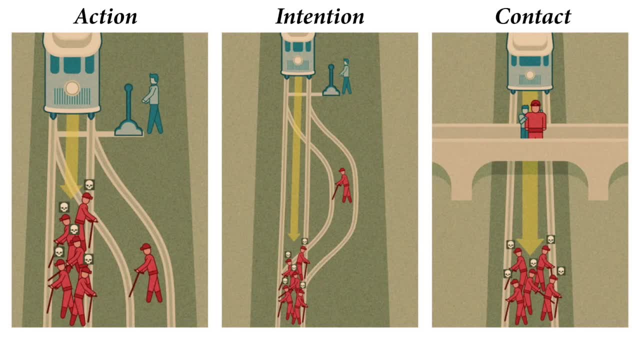 bridge that passes over the track and you're standing for some reason, behind a very large man and as the runaway trolleys speeds towards the five individuals- again, who are these five people and why are they always on the track? you can push the very large man over the railing onto the track and that will stop the 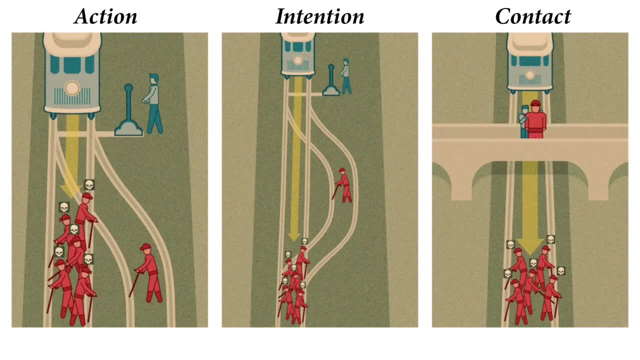 trolley and save their lives. this is a story like the loop in the middle: where there's intention, it's the large man's death as he falls onto the track and stops. the trolley is required to save the five lives of the other, so it's not merely a side effect. 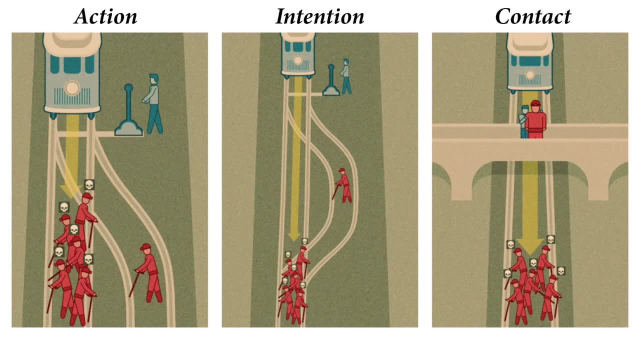 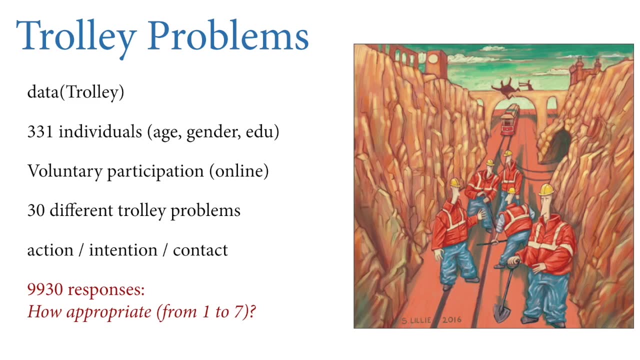 but it also requires physical contact, and this is a principle that seems to bother people a lot. so the data set we're going to work with it comes from an online study. it's a very large sample of 331 individuals, and we also know their age, their self-reported gender and their educational level- their highest. 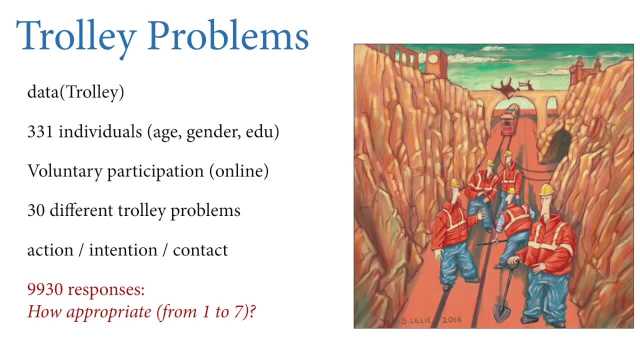 educational level. i said it's an online study and it was voluntary participation. that fact will become a very large part of this later on, and in this study, individuals were introduced to 30 different trolley problems, 30 different stories, and these stories were modified- mutated, if you will- to. 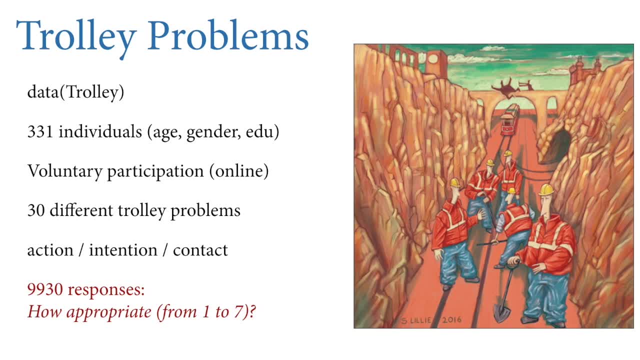 contain or remove each of the three principles in a large factorial design. so action, intention or contact can be added and subtracted to stories by modifying their details. in total, we have at our almost 10 000 responses, 9 930 responses from these 331 individuals, and what they responded to was: 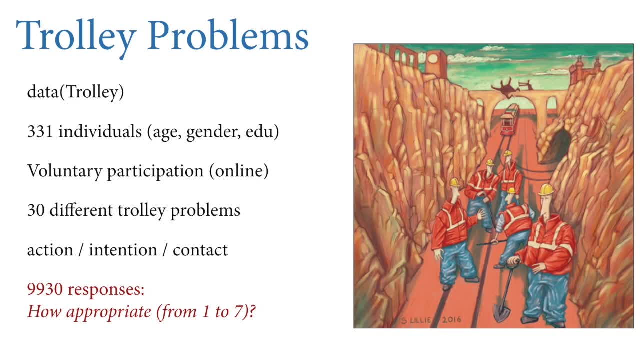 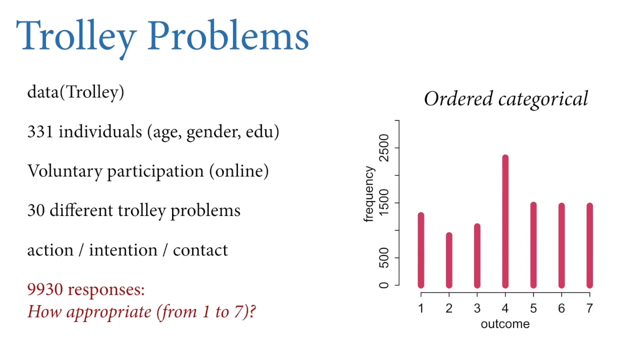 the prompt: how appropriate in any specific story is the action or inaction taken? and they give their response on a scale from one to seven, where one means completely inappropriate and seven means completely appropriate. this is what the frequency distribution of the responses look like, and this response is going to be our outcome. 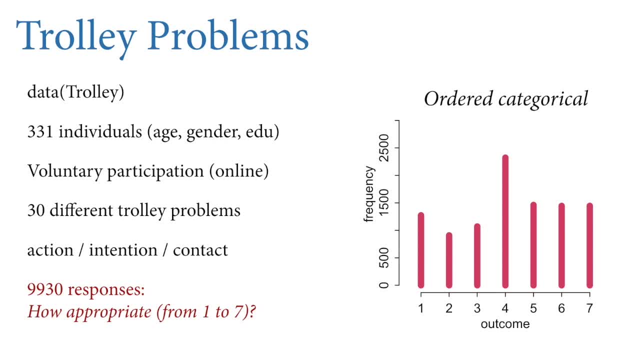 variable and we're going to construct a generalized linear model to analyze these responses as functions of the principles of action, intention and contact. this kind of variable is called an ordered categorical variable, so we need to spend a little bit of time talking about that. but first let's talk about the causal structure and figure out what we're actually going to do here. what's the? 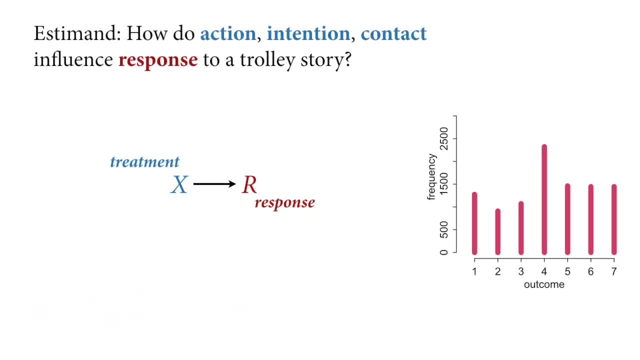 s demand. in this problem, we are interested in the extent to which action, intention and contact, adding or moving them from a particular trolley story, influences the response that individuals tend to give, where the response is defined on this one to seven scale of how morally appropriate it is. so 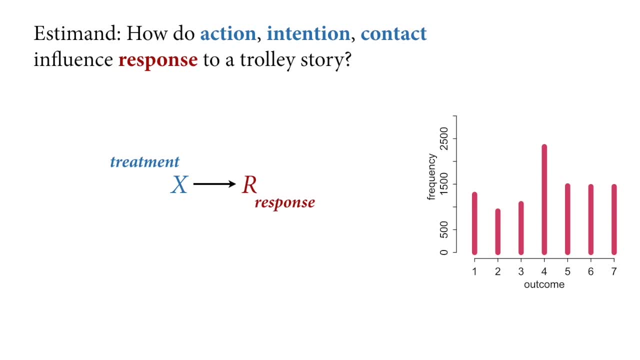 the most basic causal structure here is just: we have some treatment and since this is an experiment, it has- uh, it's under our control- and what is the influence of that treatment- whether it's action, intention or contact or some combination of them- on the responses individuals give? 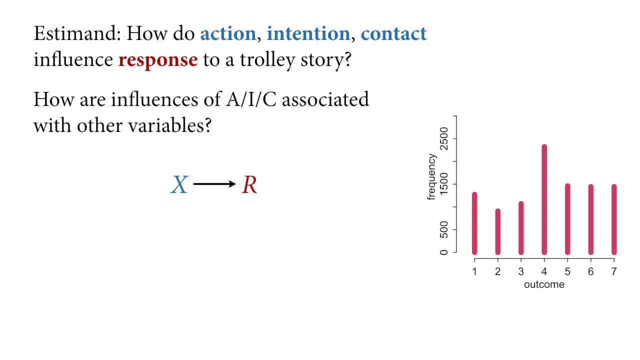 but we're simultaneously interested in how these causal influences of action, intention and contact are associated with other variables. it is not that the other variables confound them, because the the treatments x here are under our control, so they're not confounded, uh. but there are competing causes. for example, there's the story itself. some stories contain: 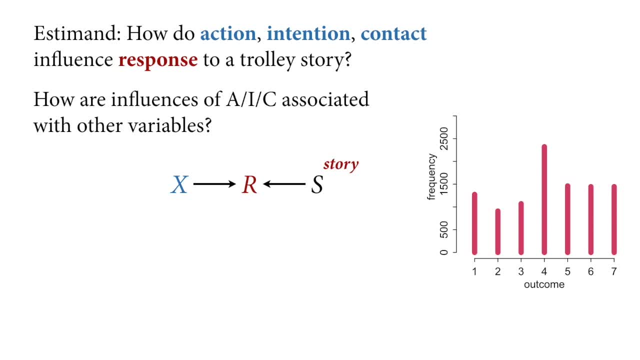 different elements, and those elements may also influence people's moral intuitions, make them more excited or less excited and affect their responses. and then there are the demographic variables about the individuals responding, their educational level, their age, their gender, and these could also moderate the response. these competing causes of action can be extremely important for the 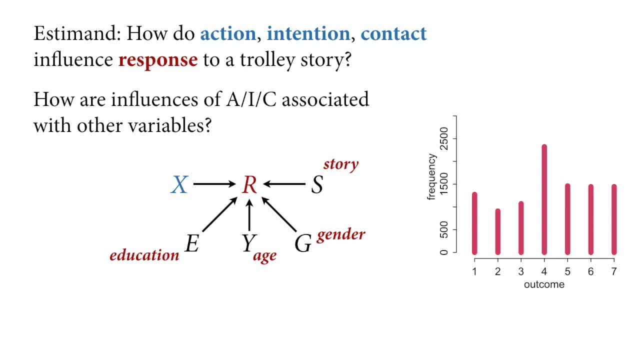 causes, as they're often caused in statistics add a lot of noise, so we often want to include them in models just to reduce the noise, so we get a more precise estimate of the treatments. But in this case they're also a primary research interest because we know that individuals 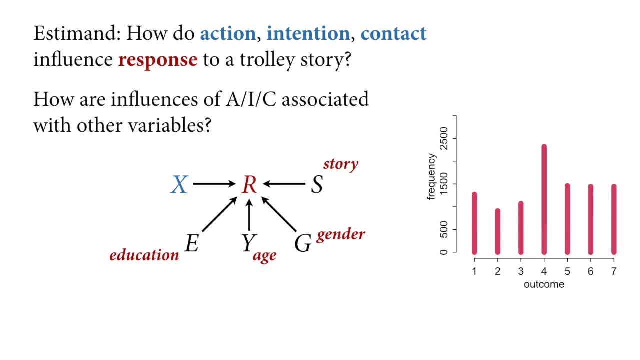 vary very much in their moral intuitions, their reactions to these stories, and we want to understand its patterning so that we can develop theories to explain it. Of course, these variables, like education, age and gender, also have causal relationships with one another. 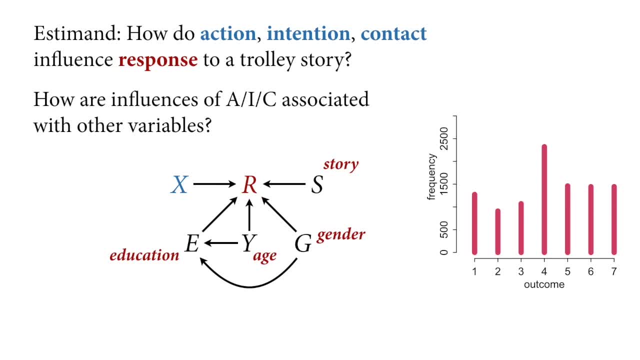 For example, age influences education. Babies have not completed college. Gender also influences education, because gender norms pattern choices in societies and lead to different educational choices, whether it's the subjects or how much education. For example, in Western societies, women seem to consume more education. 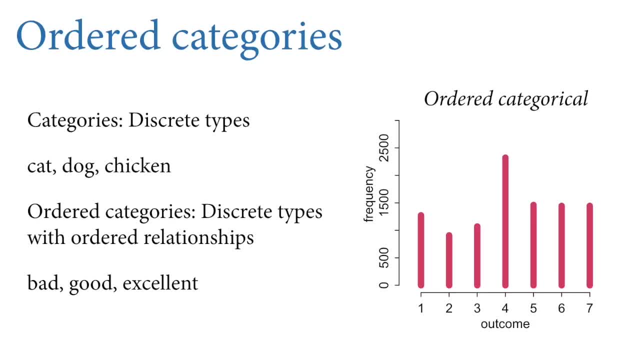 So that's the basic causal structure and we're going to come back to that DAG again and again in this lecture. But for now let's talk about the machinery a little bit. This outcome variable is a very new creature for us and we're going to need a new kind. 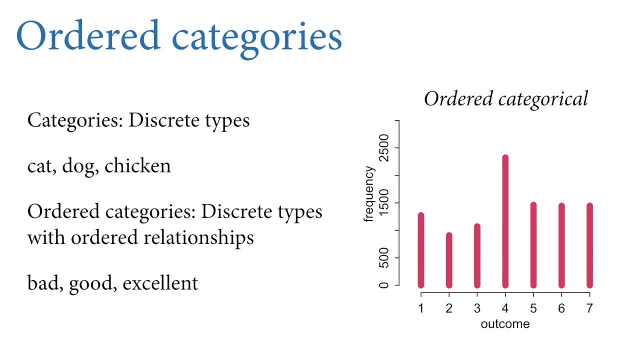 of golem to model it Order. categorical variables require some special treatment, and I want to teach that to you. So what are categories in the first place? Categories are just discrete types, and we've dealt with those sorts of things before events. 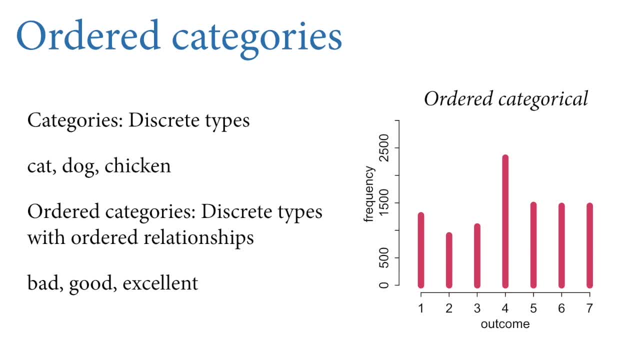 And normally categories don't have any order to them. So, for example, if you had animal categories like cat, dog, chicken, there's no natural ordering to this in the sense that chickens are less than dogs and less than cats, however you may feel. 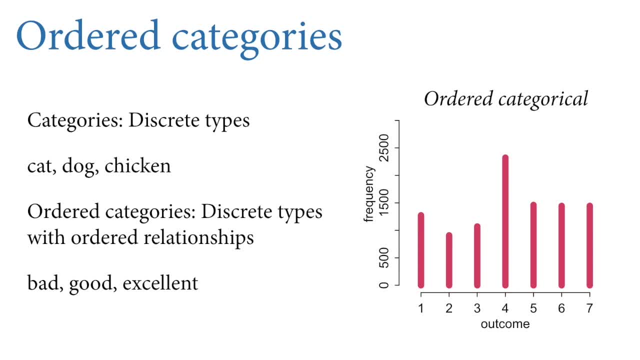 That's a normal category. It's unordered. Ordered categories are also discrete types, But they inherently have ordered relationships with one another along some dimension. So, for example, sentiments like bad, good and excellent have a natural ordering: Bad is always below good and good is below excellent. 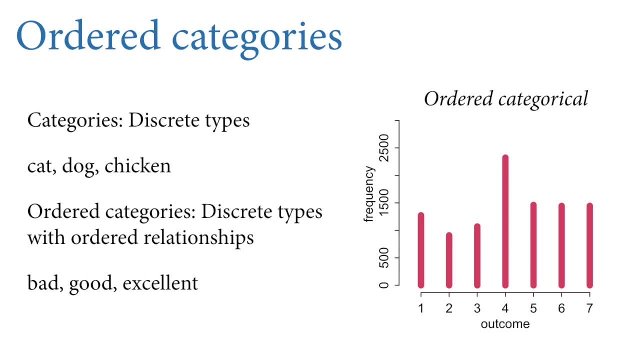 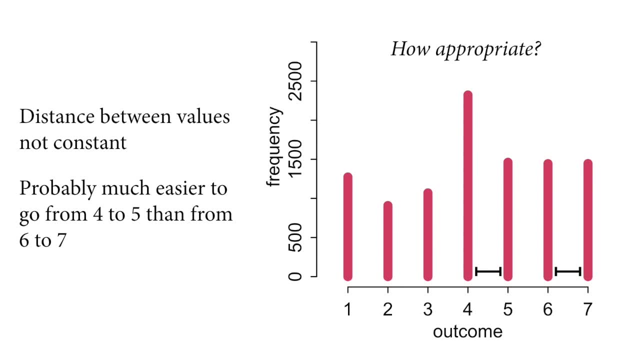 There are some things that arise from this ordering that we need to take account of when we make statistical models. The first is that the distance between neighboring values is not the same across the whole range of the outcome variable. So, for example, in the case that interests us today, if you're asked how appropriate 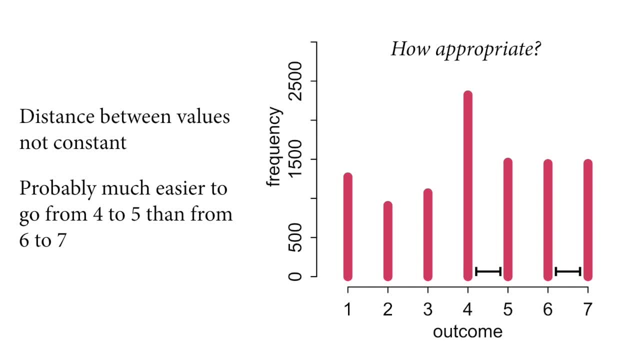 is the action or inaction taken in a story. it's probably much easier for adding or subtracting some feature to a story to move an individual from 4 to 5, that is, from sort of middle meh response to one above it, than it is to go from 6 to 7, where 7 is the maximum. These different increments have different sets of variables. So, for example, in this case we're going to move an individual from 4 to 5, that is, from sort of middle meh response to one above it- than it is to go from 6 to 7, where 7 is the maximum. These different increments have different sets of variables. So, for example, in this case we're going to move an individual from 4 to 5, that is, from sort of middle meh response to one above it- than it is to go from 6 to 7, where 7 is the maximum. These different increments have different sets of variables. So, for example, in this case we're going to move an individual from 4 to 5, that is, from sort of middle meh response to one above it- than it is to go from 6 to 7, where 7 is the maximum. These different increments have different sets of variables. So, for example, in this case we're going to move an individual from 4 to 5, that is, from sort of middle meh response to one above it- than it is to go from 6 to 7, where 7 is the maximum. 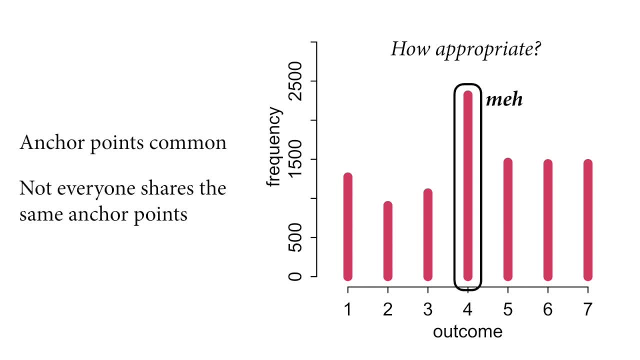 These different increments have different sets of variables. The other thing is they're nearly always anchor points, psychological anchor points. So in this study, for example, four in the middle of the scale is loved by a large number of people. They don't have a strong reaction to the story, condemning it or approving it. 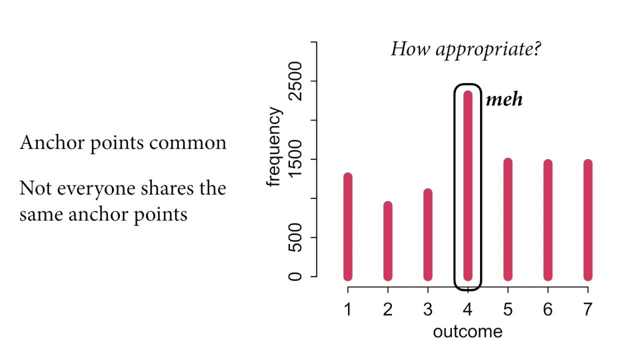 They will often choose four. This is the kind of meh response And interestingly not everybody shares the same anchor points. Sometimes they're culture-specific, individual-specific: If you have favorite numbers or unlucky numbers, you may avoid them, and so on. 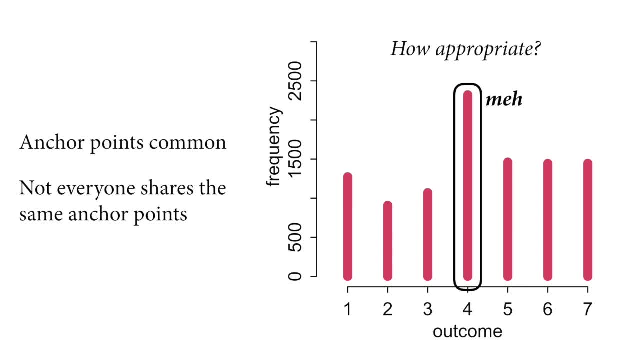 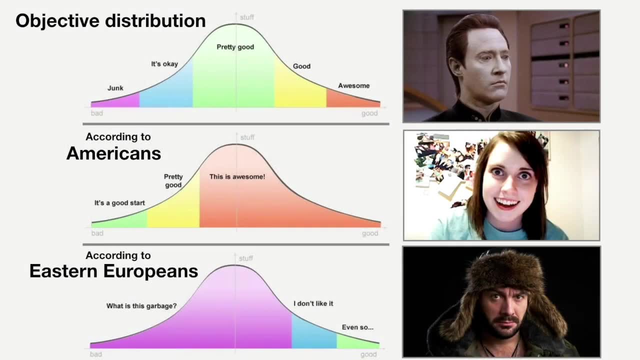 But quite often people use the middle and the ends of these scales more than the values in between. This is a bit like this Internet meme, which I am personally very fond of, where we think about different, culturally patterned ways to cut up some objective distribution. 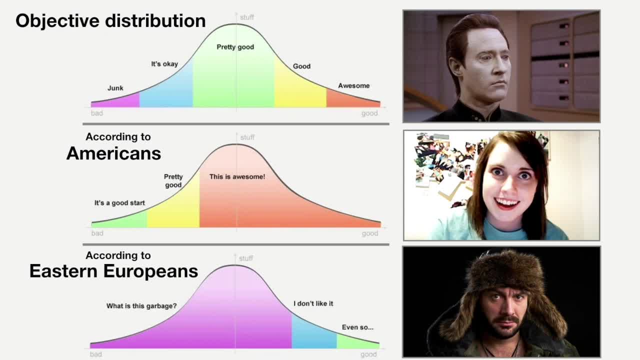 So suppose there's some distribution. There's a distribution of things and they have a normal distribution, as at the top of this slide. Most of them within plus or minus one standard deviation are pretty good And then fewer are good going up and only in the tail are they awesome. 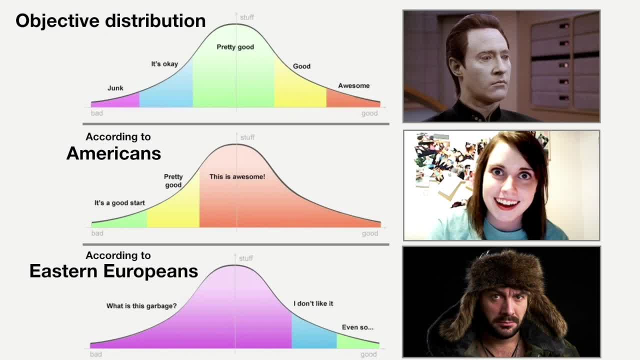 And then going the other way, it's okay. And then a very small number are junk, And some passionless android like Lieutenant Data would rate them exactly as they're distributed. But people don't do things that way. Okay, Okay, Okay. 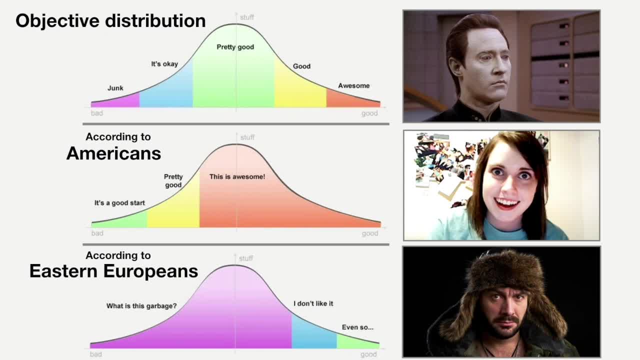 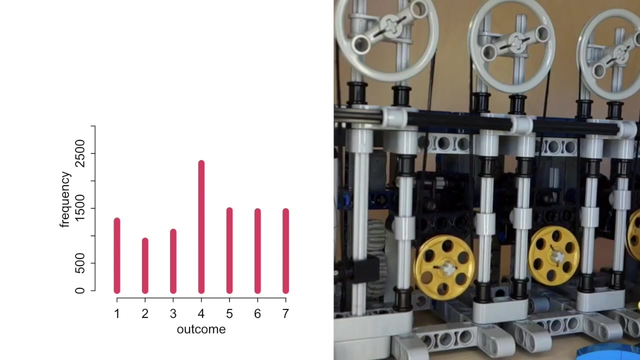 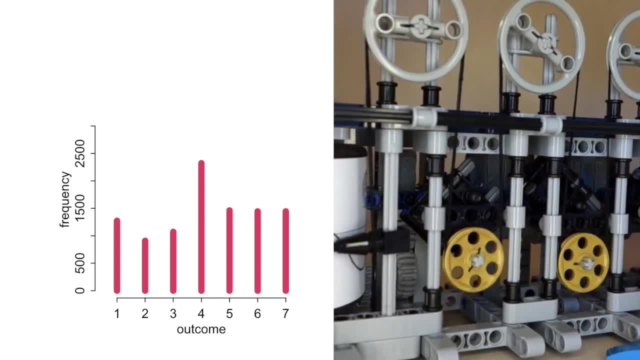 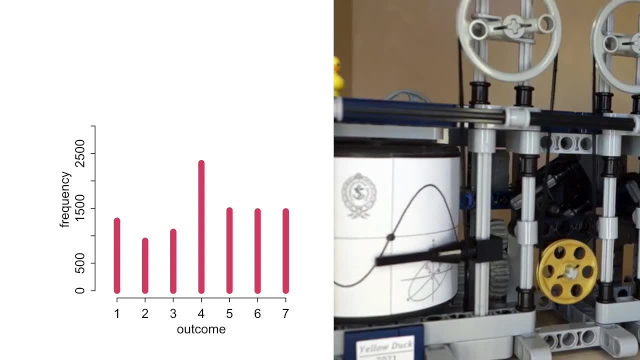 distribution. this doesn't look like any ordinary probability distribution, because it isn't it's. it's something that emerges from a bunch of idiosyncratic psychological features of the task and the people taking the task, but we still need to transform this into a probability distribution. 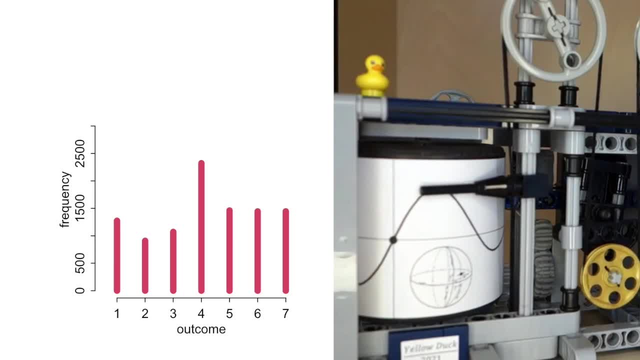 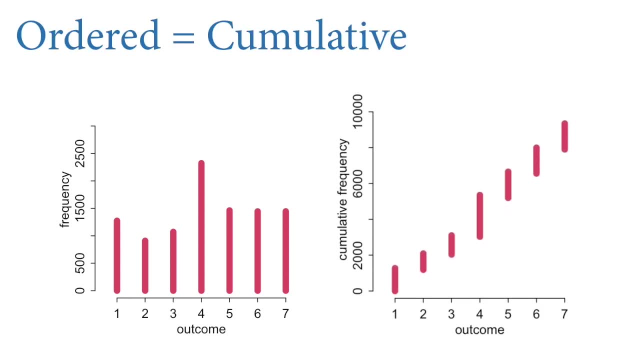 so that we can do statistical inference with it. and that's what we're going to do: we're going to make a tide prediction engine for this kind of well tide. the trick that's going to get us to where we want to go is to realize that when something is ordered, it's cumulative, and so 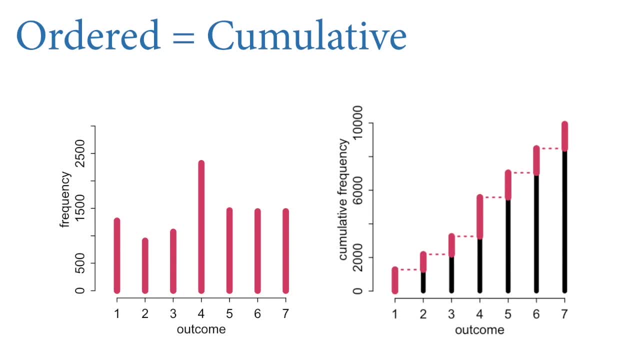 the frequency distribution on the left. the height of those individual red bars doesn't seem to have any ordering to it at all. in fact, the, the middle value, is the tallest. but if we stack them on one another, like i've done on the right hand side of this slide, 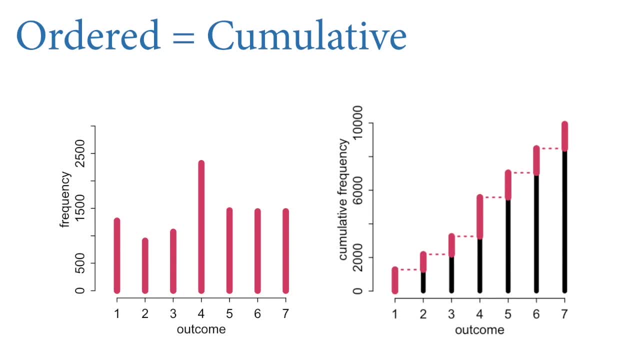 to transform an ordinary frequency distribution into a cumulative frequency distribution. and you can see what i've done. i just take, starting on the left at number one, i take number one and i stack it on top of number two, and then take number one and two and stack them on top of number three, and numbers one, two and three and stack them. 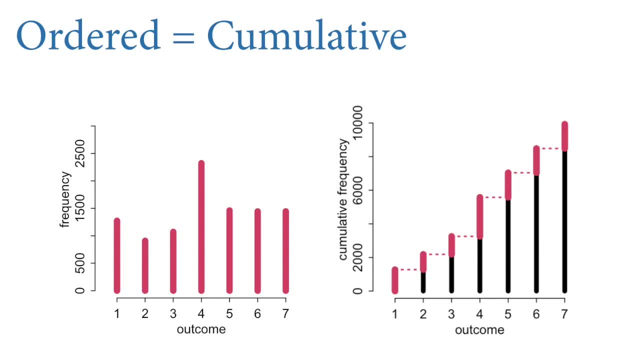 on top of number four and so on, and this makes a cumulative frequency distribution which has a natural ordering, because now each subsequent value is always bigger than the previous one, even though the distances change, and those distances are just the original frequency distribution on the left. so there's no damage that's been done here. no information has been. 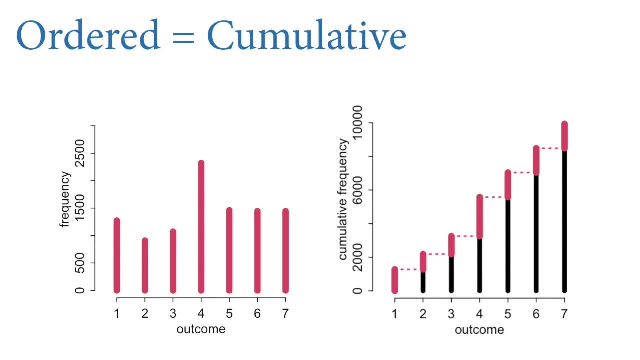 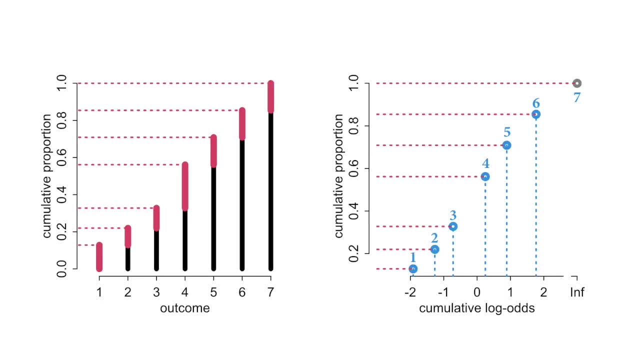 lost. but now we have represented the data in a way that has a natural ordering, and that's why these models always work with cumulative distributions. i appreciate this is a bit weird, so i'm going to spend the next few slides stepping through it carefully. usually when you 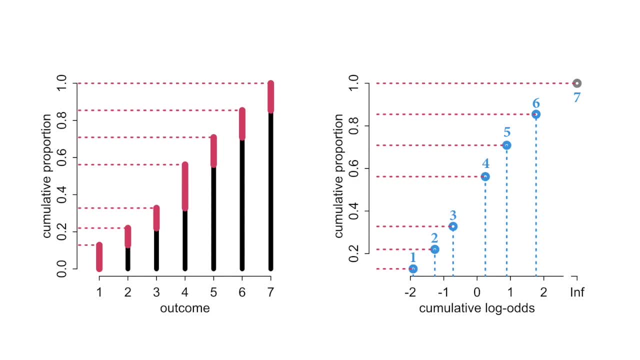 work with models like this. you can put this detail in the background. the machine always takes care of information you can use to do a lot of work using an array ofوم Democracy, and then you can use an array of arguments and you can use an array of Liege equations to figure out how far you've. 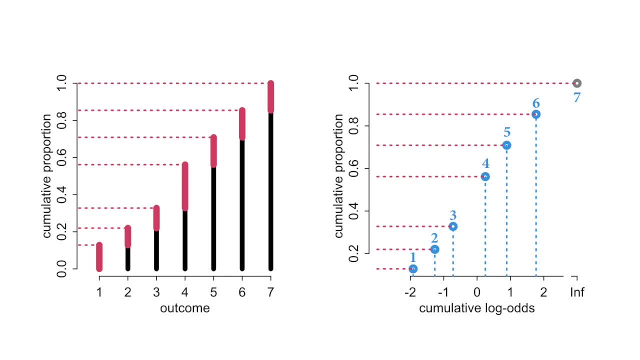 gone in terms of how many rows have you ever even done? so you can use this to figure out what you could do. and then there is a number of other ways that we can try to do that as well, and i've given you that package- a lot of information on the site here- and it's very easy and easy to. 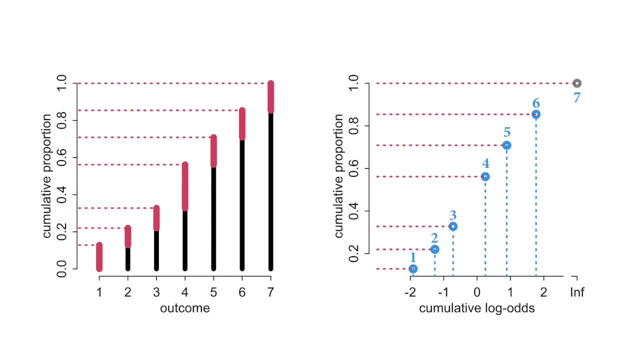 kind of get into the detail of what you could do, and i think the best way you can do is to work with a model like this one. of course, we could use the mathematical logic in relation to this model, but i, that's the entire sample. it has to be that way, and then the others are some fraction of the total. 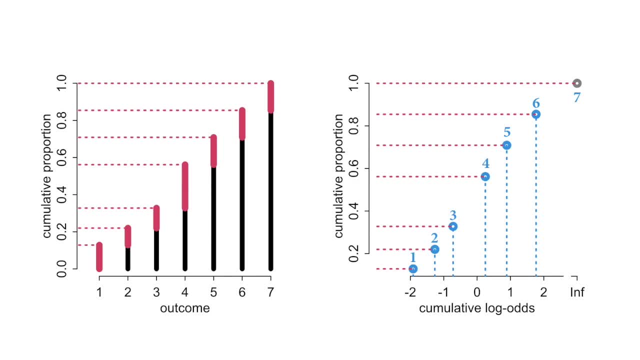 sample on the right represented the same thing. but now what i've done, the horizontal axis is not the outcome values, but it's just the vertical axis on the log odds scale. so i've taken the cumulative proportion, or probability, and i've done a logit transform on it, just like we did for the binomial. 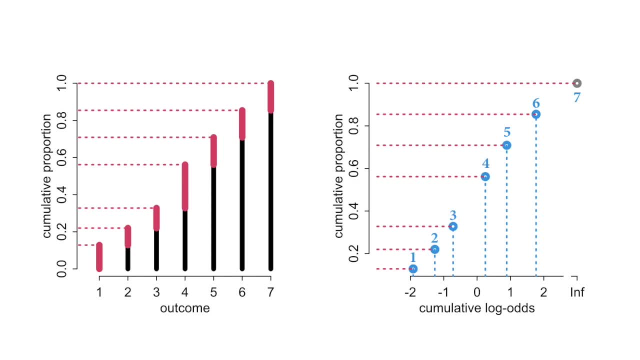 and logistic regression models last week and this has converted them onto the log odd scale. but now it's not ordinary log odds, it's cumulative log odds, but it has the same scale, the same properties. you learned last week about log odd scales, about logit scales. that is zero means fifty percent. 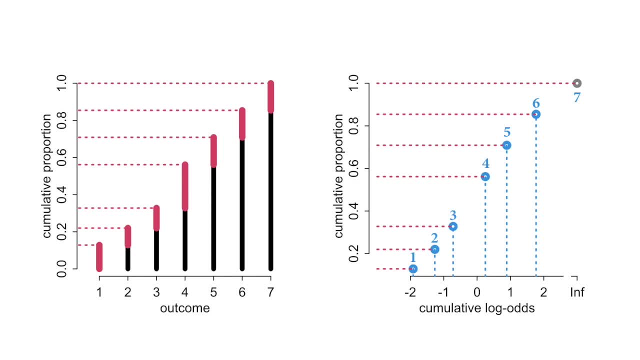 positive numbers push you closer to a hundred percent and negative numbers closer to zero percent. and now, for each of these outcomes values, we've got a cumulative log odds value that corresponds to it, and this is going to turn out to do everything for us. now i'll walk through the next bit slowly. 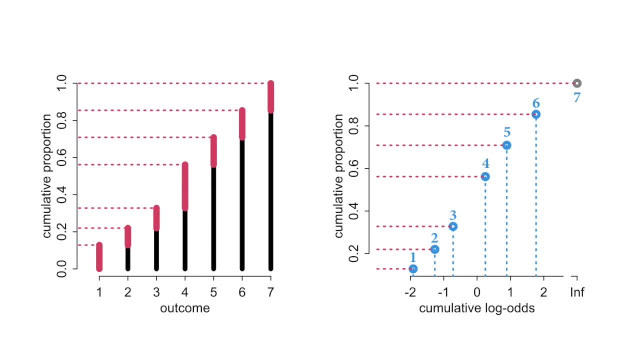 before i do, though, i want you to notice that number seven- there is cumulative log odds- is infinity, and that's because the log odds of one is infinity, because it's one divided by zero. so these um log odds values of each of these points are usually called the. 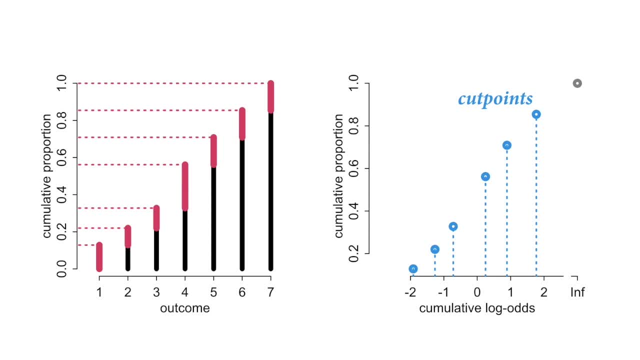 cut points and that is, their locations on the horizontal axis on this slide. and these cut points are going to be things that we're going to estimate, they will become parameters. so let me step through this piece by piece. so first realize that it's the spaces between these cut points that are 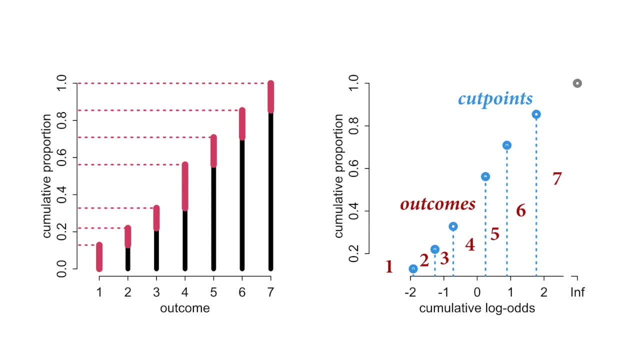 the probabilities or stand for the probabilities, the relative proportions of the different values that are observable. so, for example, all the values that are observable are observable. so, for example, all of the cumulative log odds below about minus two on this are assigned number one, which is the minimum. and then it's between the cut points, uh, the first and second cut points. 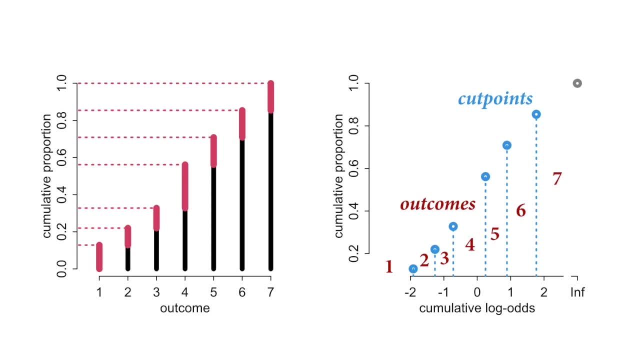 that we get values two, and then, between the second and third, that we get values three, and so on, up until value seven, which is after the highest cut point and before infinity, because it's the rest of the real number line. this lets us define the probability or the likelihood of each. 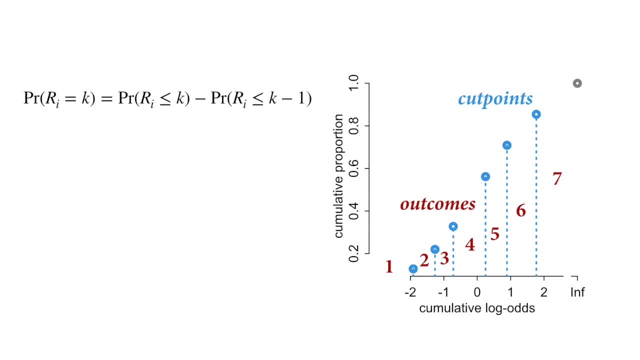 observation. so in this example, let r sub i be the response of individual i and uh, it takes some value, k, which is a number between one and seven. that's been observed and it doesn't matter which number. i'm just defining this in general and so the the probability of that response observing. 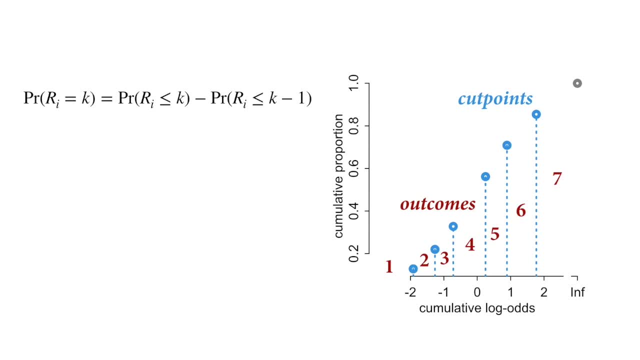 that response. uh is equal to the difference between the cumulative probabilities. uh, that that r sub i is uh less than or equal to k. right, that's the probability that it's k or anything smaller, minus the probability that it's one less than k or anything smaller. 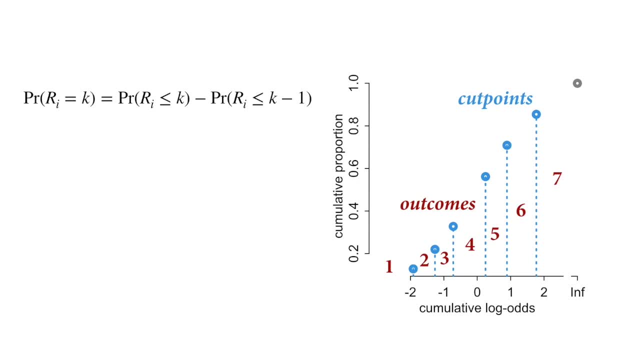 and so how does this make any sense? well, this is where the, the cut points, give us those probabilities. that's what we've got, because the we have a cumulative distribution now, and so it's these less than or equal to probabilities that we have in our, in our machine now, and not the 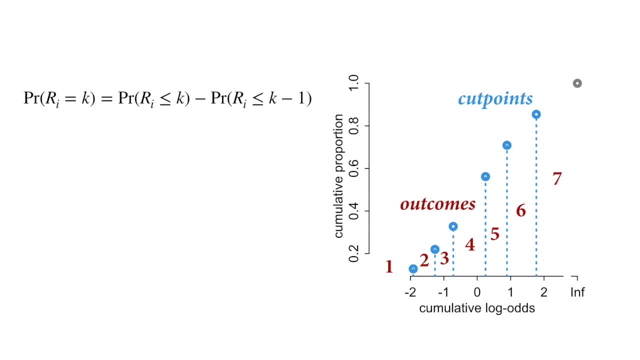 discrete ones. but we can get the discrete ones back. the probability r i equals any specific value k, just by subtracting one from the one right below it, and that's what these cut points are going to do. they represent those probabilities of less than or equal to. let's say: 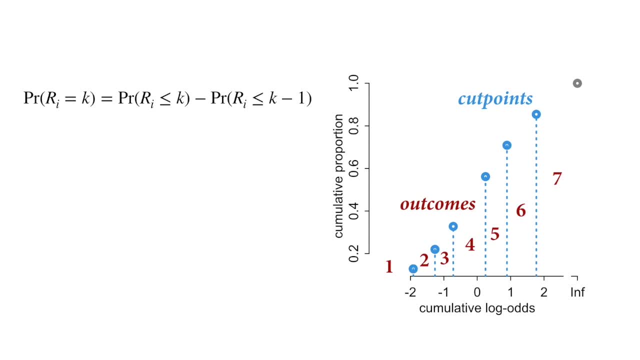 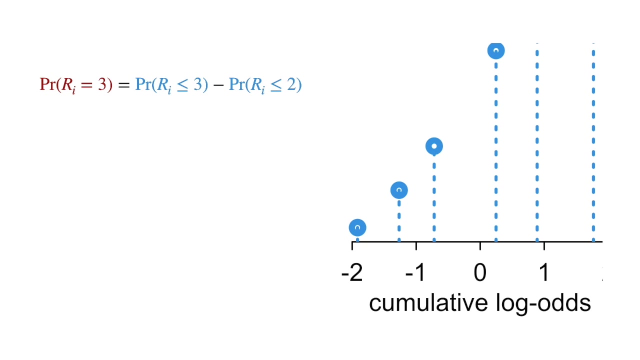 the first cut point is the probability that any observation is less than or equal to one, and the second the probability that it's less than or equal to two, and the third the probability it's less than or equal to three, and so on. an example: i appreciate this is weird. 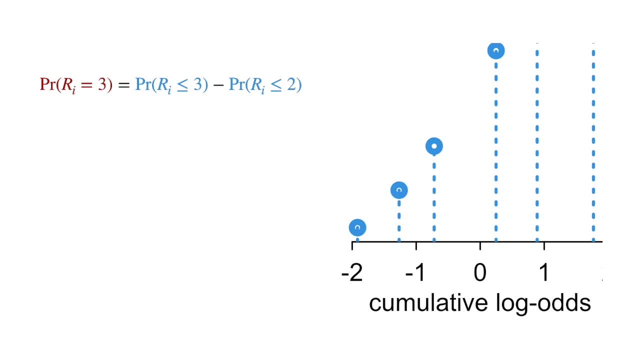 it's weird every time i teach it, and i've been doing these models for, uh, almost two decades. so let's suppose that the observed outcome value is three, so that we want the probability that r sub i equals three according to our model. well, this is necessarily the difference between the cumulative 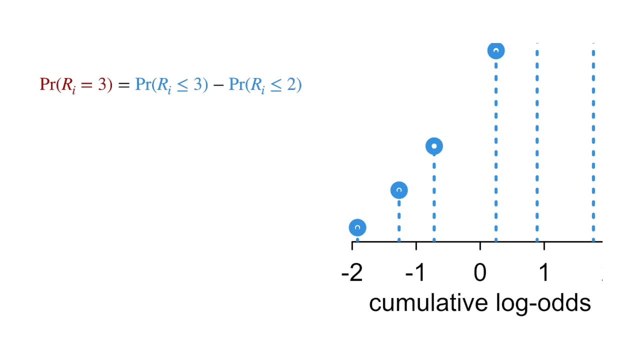 probability that it's three or less, minus the cumulative probability that it's two or less. so where are these on this graph? well, this cut point right here. the second one is the probability that the response is less than or equal to k, or anything smaller than or equal to one, and so on. and 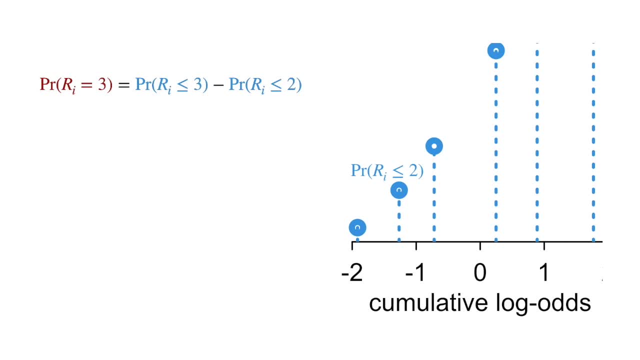 the third one is the probability that the response is less than or equal to two on the log odds scale. right, but its height on the graph here is the probability scale. so the horizontal axis is cumulative log odds, the vertical axis is um is cumulative probability, and so the height. 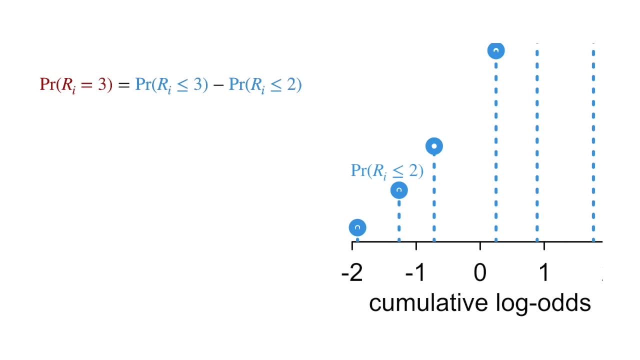 where that blue dot is. that's the cumulative probability that the response is less than or equal to two. and then the third one is the cumulative probability that the response is less than or equal to 3, and 3 is the value we're interested in, so we just take the difference. 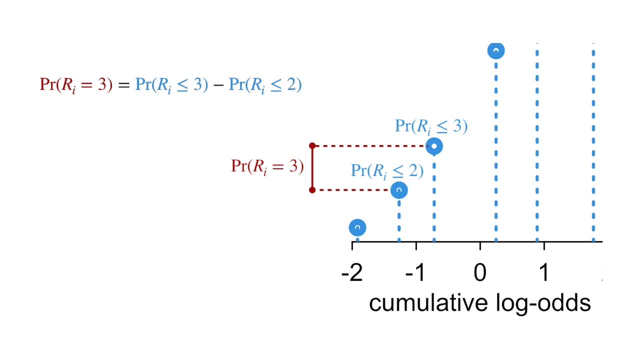 between these two. the difference between the height of these two points is the probability. r sub i equals 3 according to the model, and that's also all the machine needs to calculate. we're going to build a model that does this, that does all these little incremental calculations with. 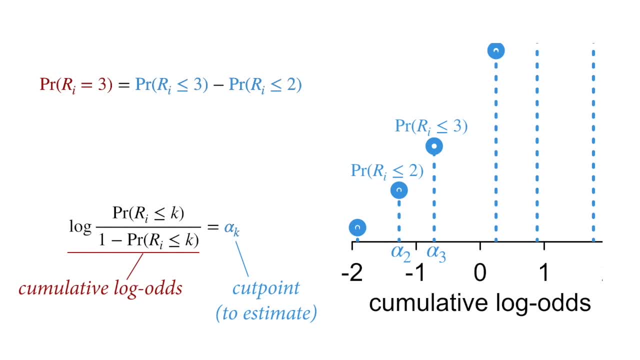 cumulative log odds. what we end up with is a link function. this will be a generalized linear model, a very weird one, but it will be a generalized linear model where the link function is something called the cumulative log odds or or cumulative logit link, and i'm showing it to you on the slide. 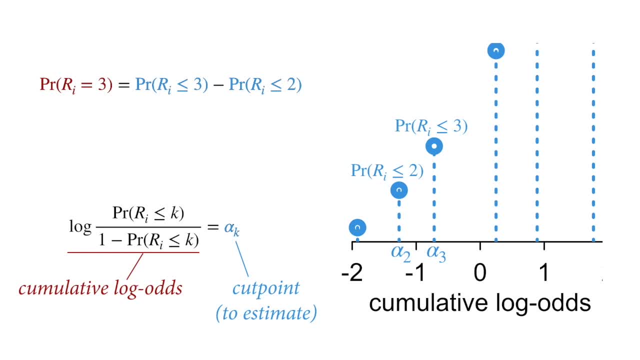 here, and we set that as always, so that the cumulative probability transformed by the cumulative logit is equal to our linear model. but in this case we have one cut point for every, or sorry, we have one intercept alpha for every cut point, and that is we're going to have. if there are seven possible responses, we're going to have. 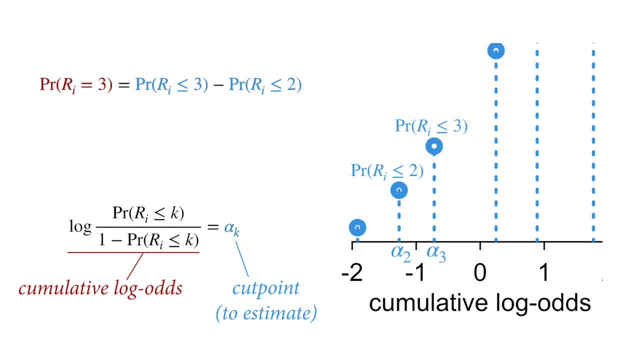 six alphas to estimate, because those are the six cut points and every unique value k has its own intercept that we're going to estimate. and then we're going to stick other things on this linear model, but we can wait a bit to do that. but in essence, the locations of where those vertical dash 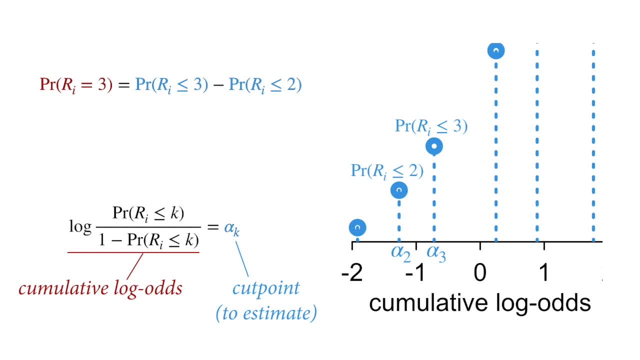 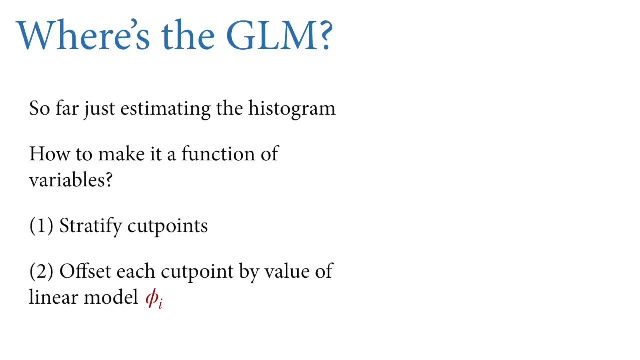 blue lines on the slide, hit the horizontal axis. those are the parameters we need to estimate. there'll be one alpha for each of those locations and we learn them from the data. okay, what that does effectively is learn the frequency distribution of the sample, with the uncertainty that it is it deserves, given its sample size. that's already. 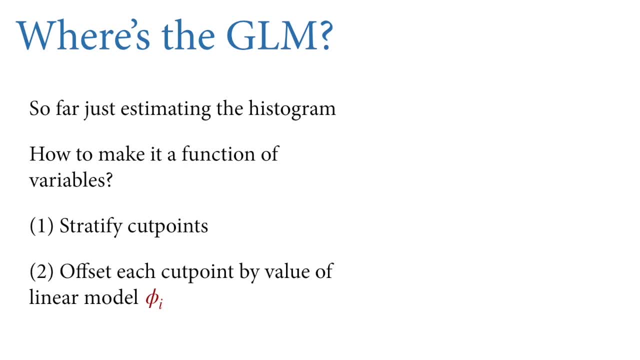 something right. this is a bayesian version of of frequency estimation that that respects the uncertainty in its structure. but we often want to have more variables in here to explain the differences and difference between individuals and the treatment effects. so how do we make something like this a function of variables? well, the first thing you could do is you could. 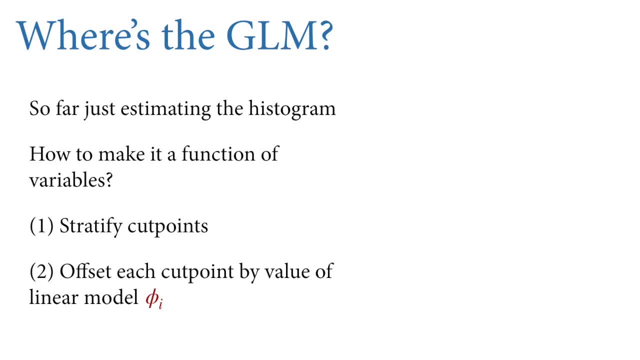 simply stratify the cut points by your explanatory variables. for example, you could have one set of cut points for the young and one set of cut points for the old, if you're willing to binarize age in that way. the second thing you can do is use the classic linear model strategy. 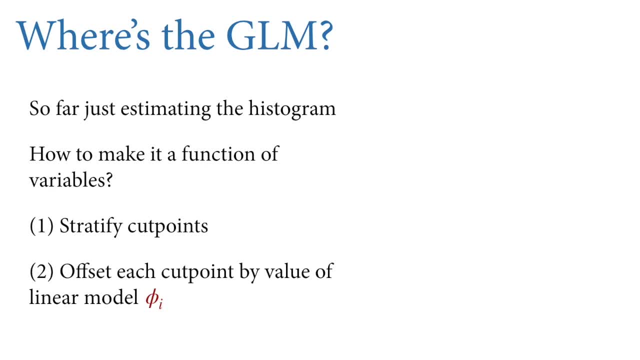 so in this case, what we do is we offset each cut point by the value of some common linear model common to all the cut points, and we're going to call that phi sub i. so what this looks like is: well it it looks like a linear model. so phi sub i will equal some set of slopes times their. 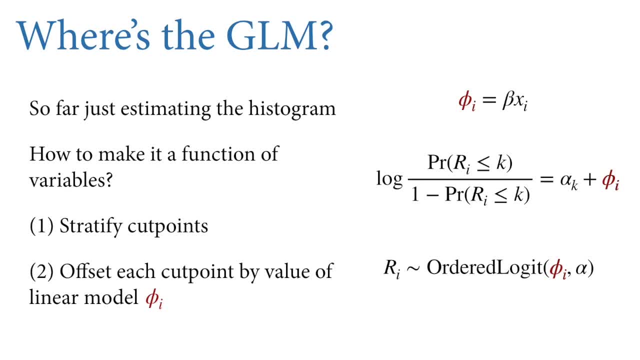 predictor variables. so looking at the top on the right of this slide, phi sub i equals beta times x sub i. there's no intercept in this because the cut points are the intercepts. so if you look at the middle on the right of this slide, we have the cumulative log. odds is equal to. 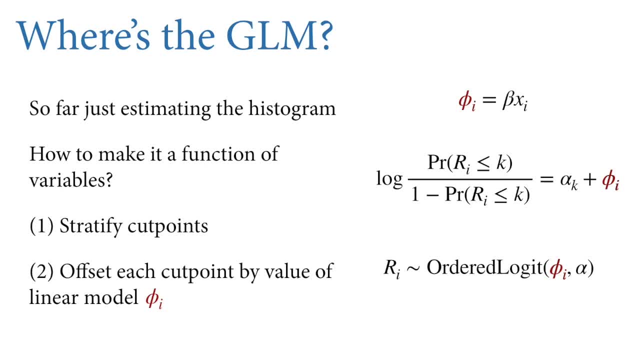 alpha sub k plus phi sub i, and that alpha sub k is the intercept that's specific to each observed value, k. so the intercepts are free in this model and if you stick them in phi it won't destroy things, but you will get confused and it'll make the chains run inefficiently. 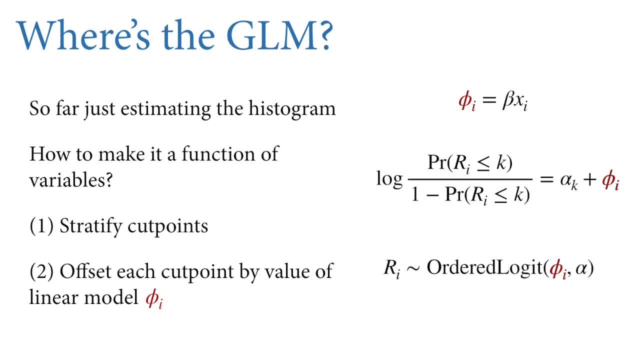 they're not, it's not necessary to have extra intercepts. and then usually the way we denote these sorts of models, these cumulative log odds models in a in a statistical definition, is we have a distribution we call the ordered logit distribution. it's really a type of categorical 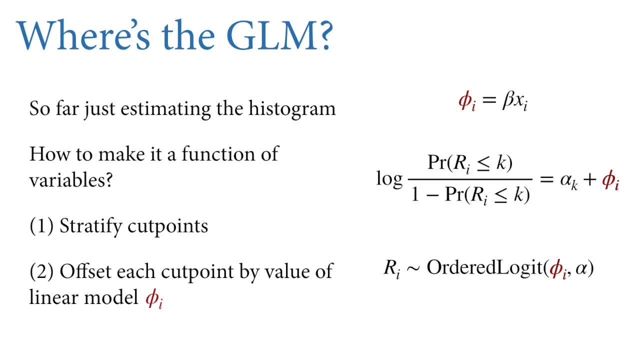 distribution, and if you look at the section of the textbook where that explains this material, i show you how to write out this model as if it were just a categorical model. but it's very messy, so but take a look. if you're interested, i'm going to use this ordered logit notation in the 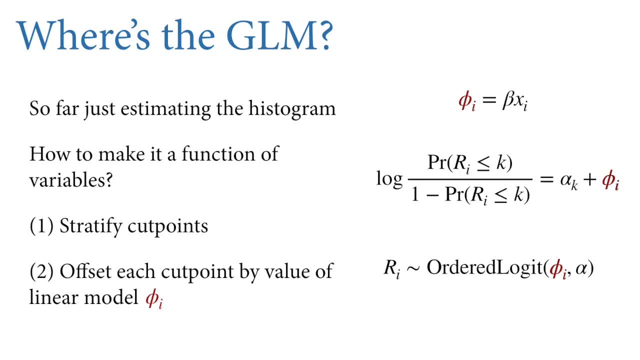 lecture, just to make things simple. and the shape of the ordered logic comes from its linear model, phi, sub i and the whole vector of alphas. so when i write alpha without a subscript, i mean all of them, and in this case it's all six of them. right? so only six, because the seventh one is free. 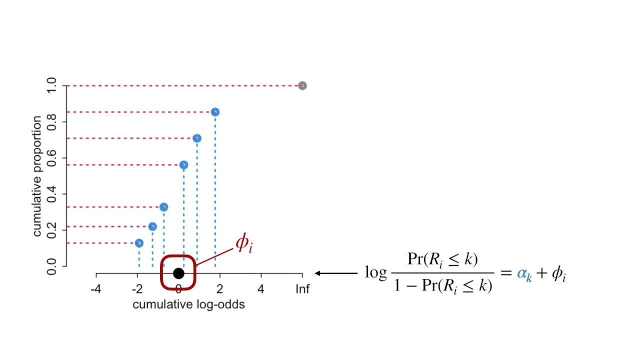 we know it's infinity. okay, that was a lot, but let me make one more attempt to give you an intuition for how this works. what you're looking at now is on the left. here is a graph you've seen before. we've got the cumulative log odds along the bottom. 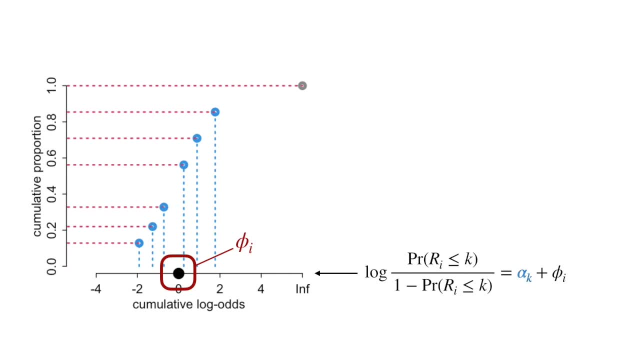 and we've got each cut point represented by the blue dash lines. and then the blue points are at the height of where the cumulative log odds have been transformed to the cumulative proportion to probability. yeah, so the vertical axis is just, is just probability, right? the inverse, uh logit, of the 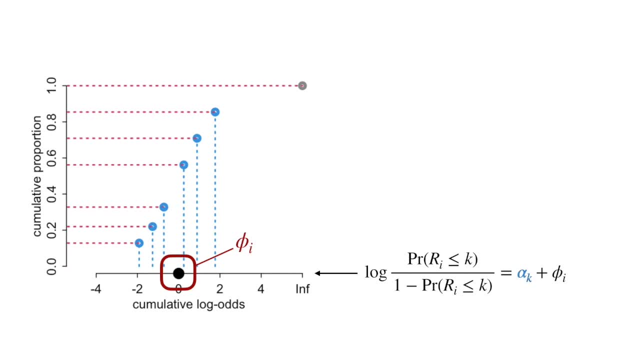 log odds and i've placed this um black mark, uh, on the on the horizontal axis, which is going to represent the value of phi, and i'm going to move this mark and slide it along the horizontal axis so you can see what this does to the implied distribution. 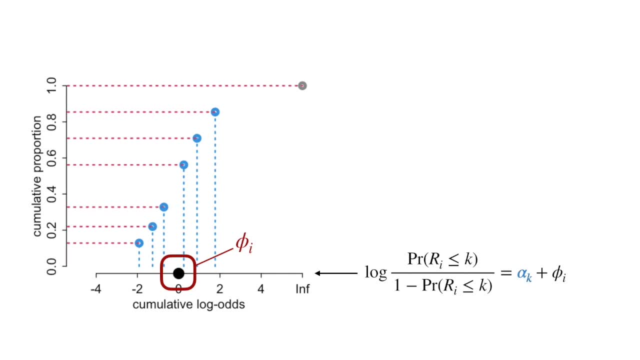 frequency distribution from the model. one way to think about this, as i've tried to indicate on the right of the slide, is that the horizontal axis is the value of the linear model in the ordered logit glm. so it's, it's a set of specific alphas, each alpha sub k. 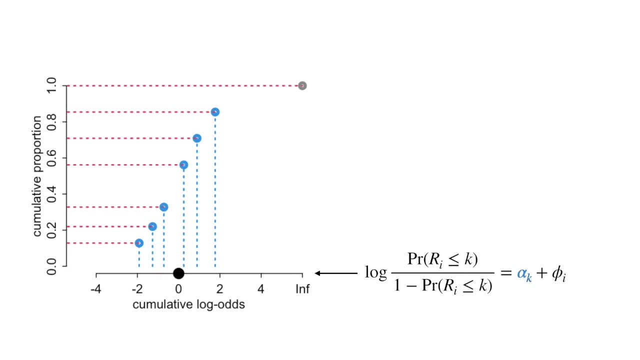 plus the value of phi. so now let's modify phi. so what i'm showing you here is when phi equals zero. in this particular example, this is the frequency distribution that's expected. that is, the height of the red lines on the right are the distances between the vertical distances between the red. 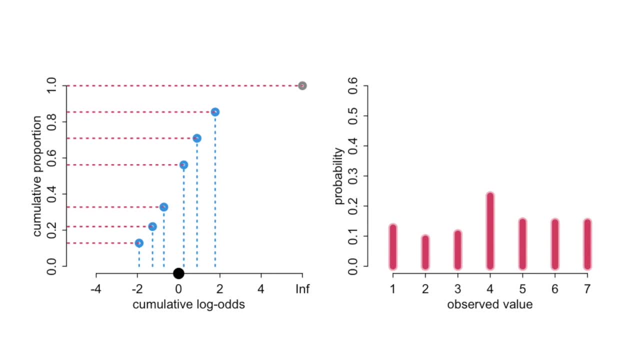 lines on the left. those are the probabilities of each of the specific outcomes and you can see right if you. if you look at four, four is the tallest bar on the right and four is the tallest gap on the left between the red dashed lines. do you see that? okay, good, because now i'm going to 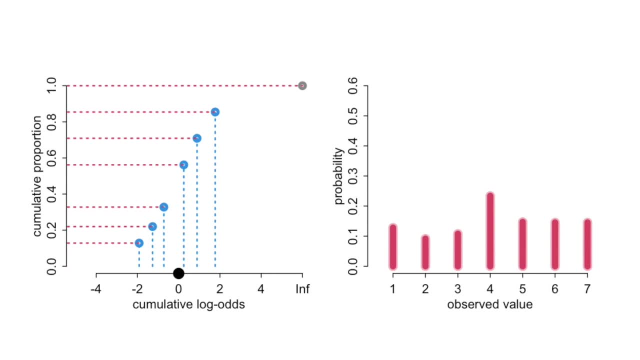 start this whole thing in motion and i'm going to let v move. let's increase it up to two, and what happens is you notice that the, the blue vertical lines, maintain their distances with respect to one another on the cumulative log odd scale, and we've just added v to all of them. 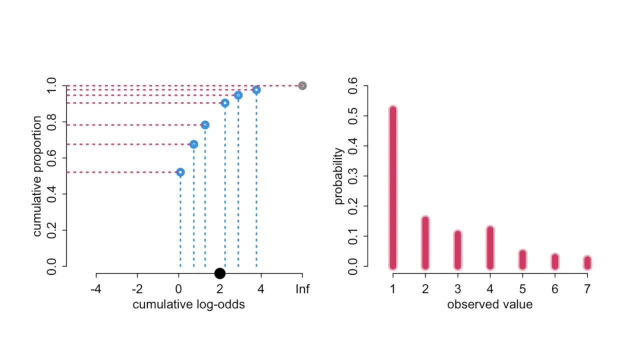 so they don't change relative to one another. but on the probability scale, the vertical axis, they definitely change their relationships to one another, because you can't go above one, and so as the probabilities get pushed up, uh, on the log, as the log odds get pushed up, the 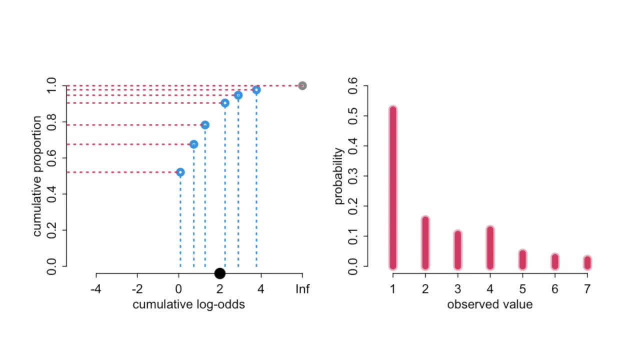 probabilities, uh, distances get smaller and smaller, and this transforms, it mutates or morphs the whole histogram. and so now what you see is what this does is if you make phi bigger, it makes the lower values more likely. i'll say that again: if you make phi bigger, it makes the 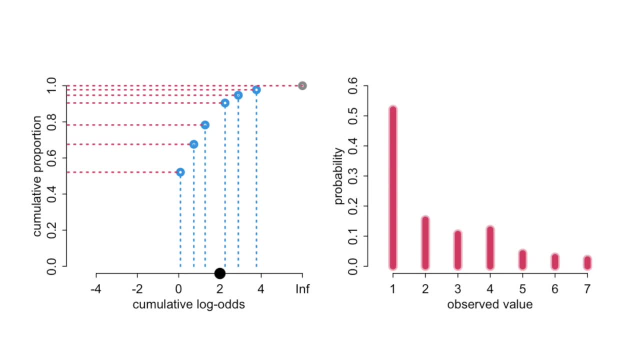 lower values more likely. and so you can see what that's done to the frequency distribution here is it's made one have a very high value, and now let's slide it the other way. i'm going to slide it all the way down to minus 2 and you 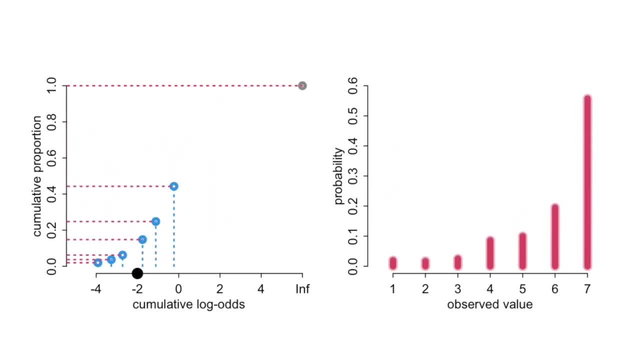 can watch it do the reverse, and now everything gets squished along the bottom and now 7 is the value of phi, because we've created this big empty space overhead where the outcome is going to be 7.. so we can keep alternating this back and forth between 2 and minus 2 to prime your intuition. 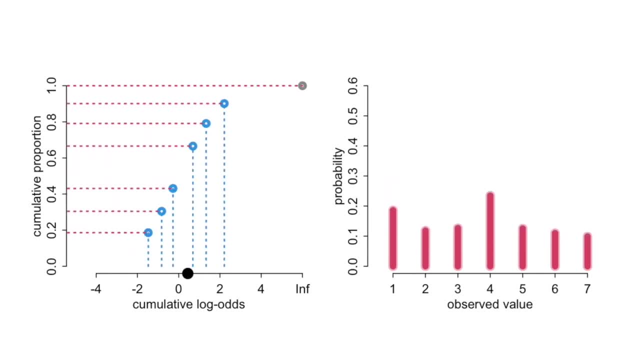 about this thing. this is how these models are built. you add terms to phi that distort the graph and help you understand how the predictor variables result in changes in the frequency distribution, and that's an ordered logit model. so here's an example of a problem that we're going to be looking at in the next slide. 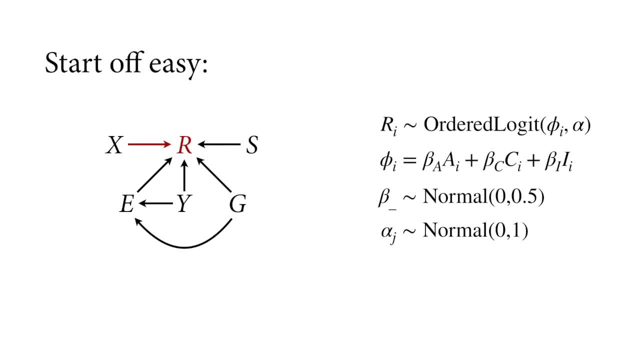 so let's start off with a simple problem and then gradually layer in our estimands in this example. so to remind you, we're interested in understanding the effects of treatments x on the responses are, and we're going to focus only on that simple causal relationship. for the moment, the average 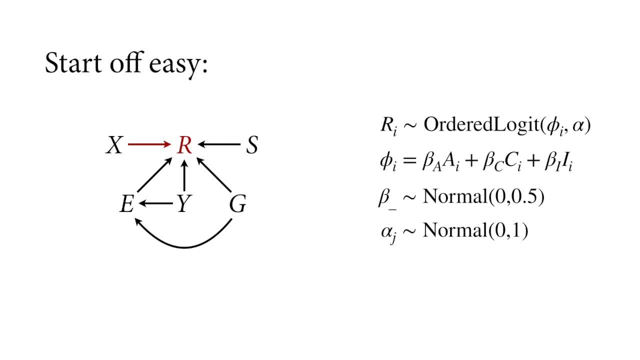 causal effects of each of the three principles: action, intention and content, and so on the right of this slide i've showed you the simplest or sort of ordered logic model that contains these three factors and i've made a sub i the presence or absence of the action principle in a story. it's a 0, 1 variable and c. sub i is the presence or absence of contact. 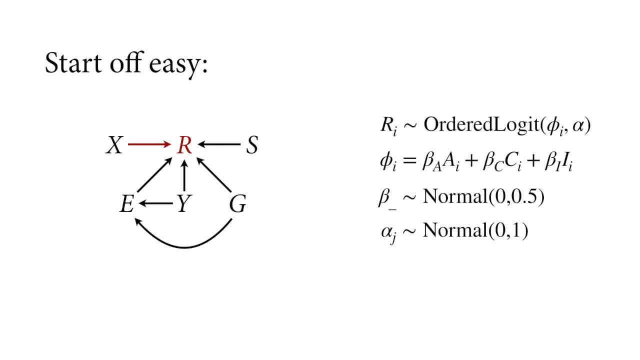 in the story and capital i, sub i, is the presence or absence of intention in the story, and we add each of these to phi with its own coefficient: uh, beta sub a, beta sub c or beta to the z wave of i respectively, and then for the priors beta with that flat line in the subscript. there i'm. 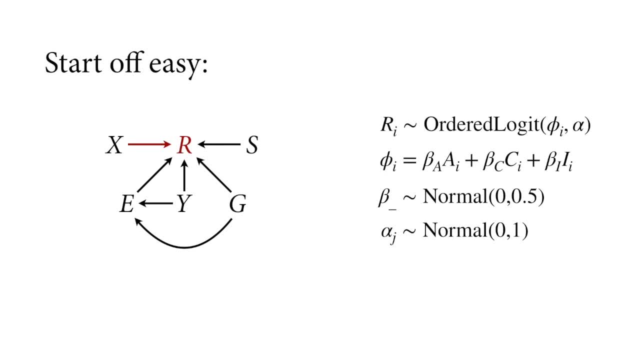 going to use that in this lecture to mean any beta, so that flat line could be any letter, a, c or i, and we're going to give them all the same prior normal with a mean of zero and a standard deviation of one half of 0.5. and then for each of the alphas- remember there are six of them for each of the- 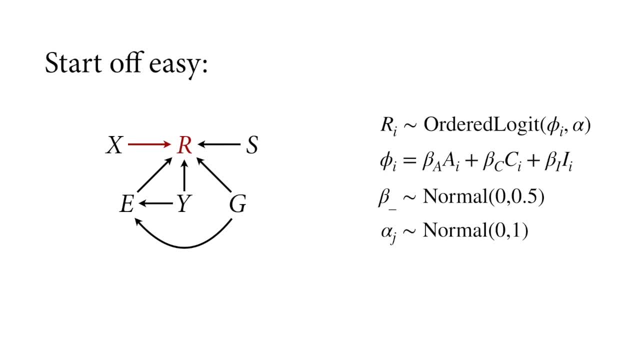 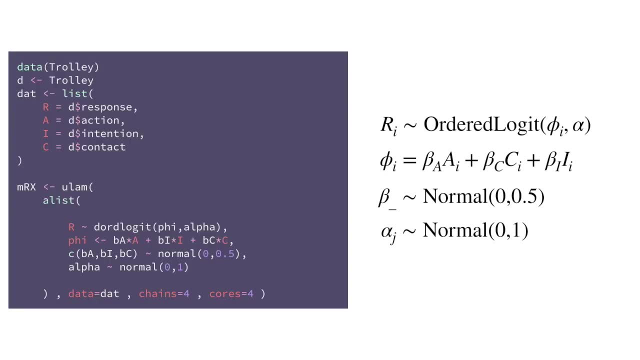 alphas. i'm going to give it a normal 0- 1.. remember these are on log odds, so this is like the log odds intercepts we talked about last week in code form. there's no big uh struggles here. there's a distribution in the rethinking package called d or logit. you can say it doored logit if you like. 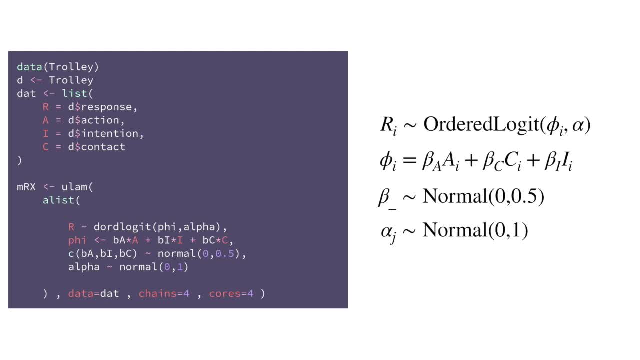 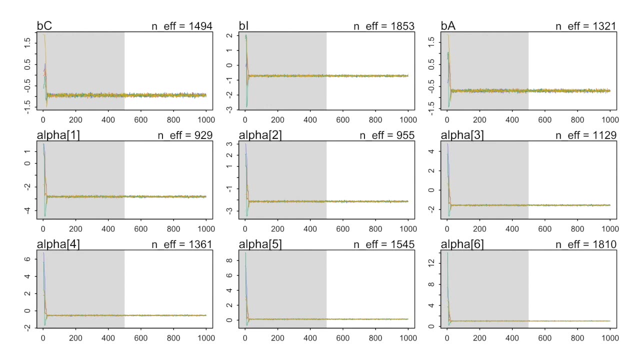 and this is the ordered logit distribution and it takes v and a vector alpha and you define things as you'd expect and uh, ulam will happily run this. let's look at the chains. uh, i want to look at the trace plots here, because they're- they're, the chains are fine, but these. 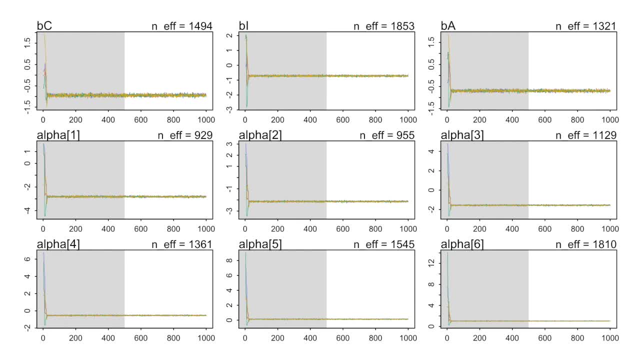 trace plots are very hard to read because the chains start from such highly dispersed places in the probability distribution- which is good- that by the time they've converged it looks like a thin little line and it's hard to see if there are any anomalies or anything bad going on the tranq plots. 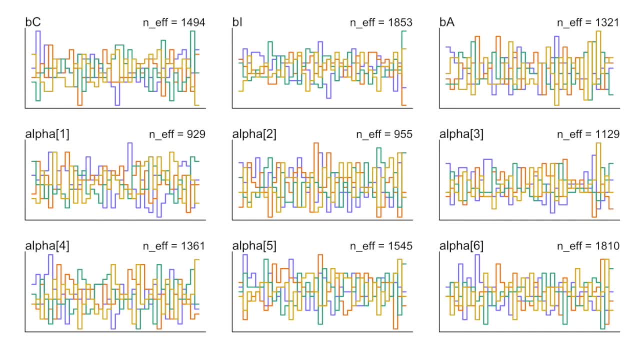 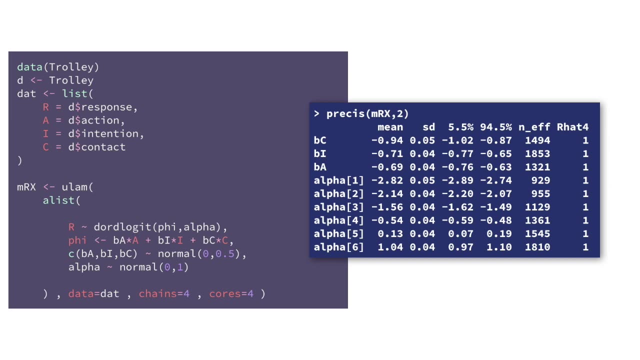 always don't have that problem. they're much clearer and you can see that these chains show lots of evidence of having converged and of good mixing. okay, if you look at the marginal posterior distributions from this model, as in the pricey output on the right of the slide, it's pretty hard to see what's going on. 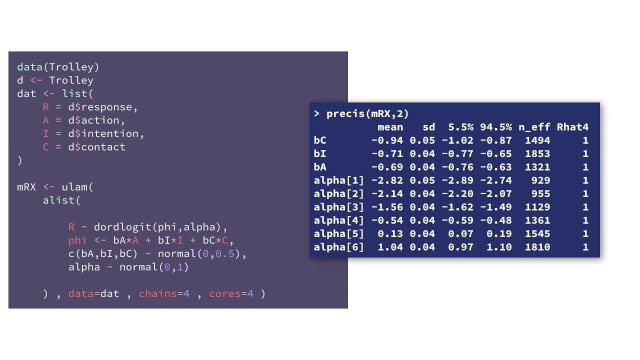 all of these things are on the cumulative log odds scale, and i don't know about you, but i have a hard time thinking in cumulative log odds. it's a bit difficult to figure out what's going on. the alphas are locations on the horizontal axis, and so, of course, 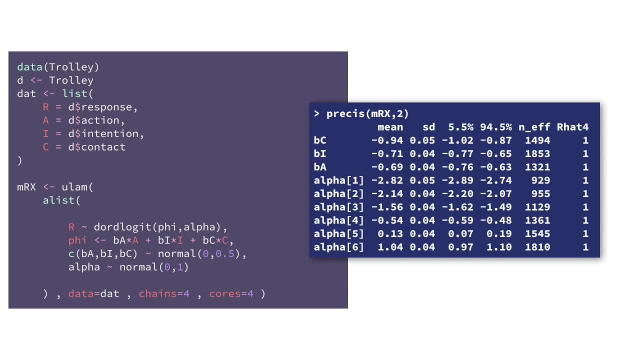 the smaller ones have smaller values. they have to be. it's ordered and it'll always be ordered that way. but it's hard to read these things directly, and the same goes for coefficients. you can kind of look at them and see: oh, a negative value that's going to decrease things and a positive value will. 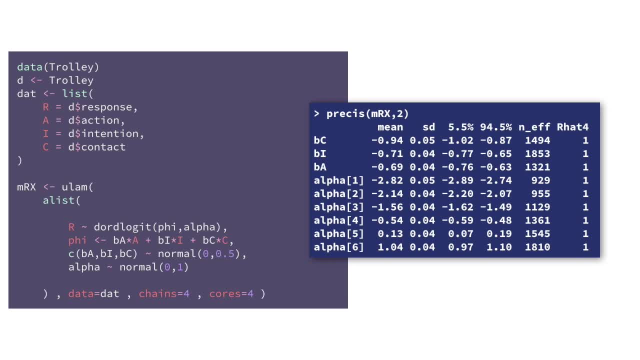 increase them. but it's hard to figure out what's going on in the derivative log, so it's hard to know by how much. so you know what's coming next. we're going to simulate from the posterior distribution, pushing it back out of the model, treating it as a generative model so that we can 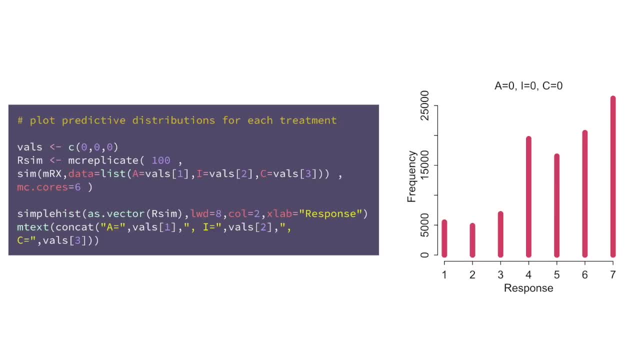 see what the implications of of the machine are. it doesn't take much code. i'll show you. and there are different ways to do this. here's the way i did it. for this example, i set up a vector called vowels that contains the the values of the a, i and c variables, and i set up this little vector so that 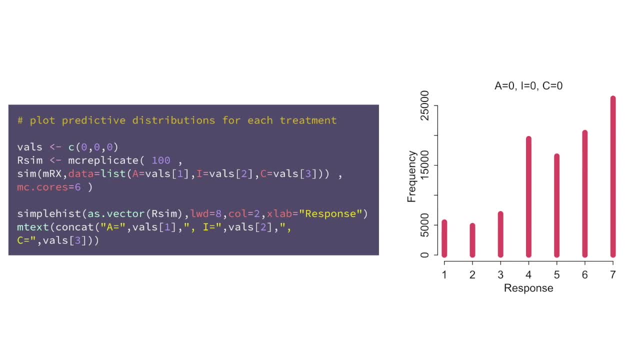 i can change it easily and then i simply use the rethinking package's sim function to simulate from the model with those values. but i do it a hundred times because we're simulating observations and i want the expectations, and sim can only simulate as many observations as there are samples in the posterior, and so we got 2000 samples from the posterior. but 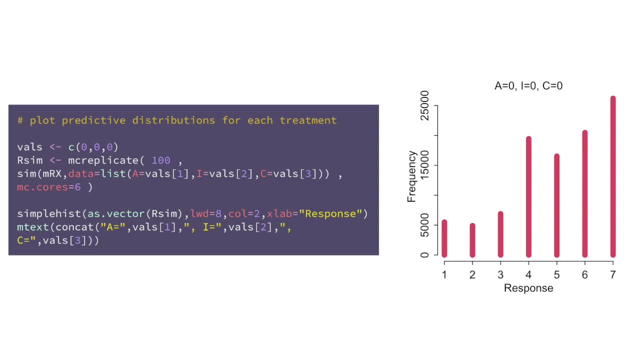 i want more simulations than that, so i'm going to use mc replicate to loop through those 2000, 100 small objects and simulate different observations. remember there's a different contribution of the stochasticity when you push observations out of sim. so we want to average over that. 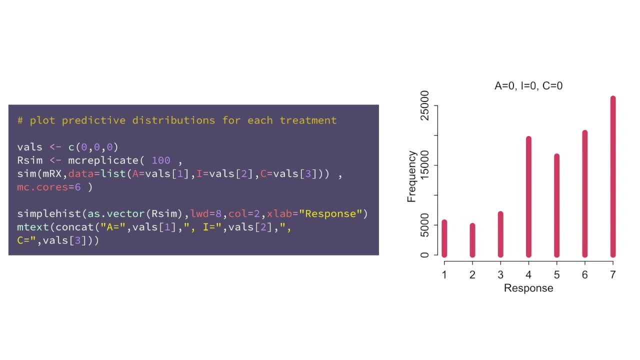 and i use mc replicate to use all the cores. so i use six cores here. so this finishes pretty quickly and then i just draw the histogram and that's what you see on the right. so i'm going to draw this type of histogram for different combinations now of the treatment variables a, i and c. 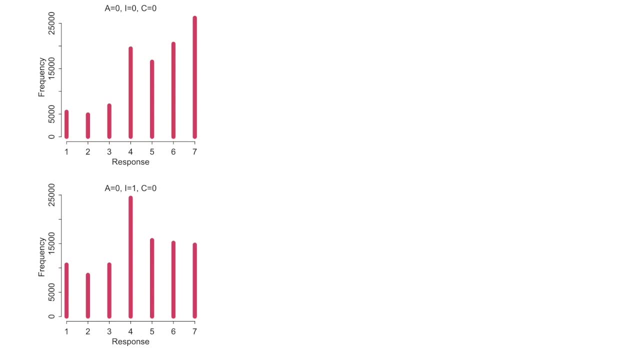 So let's take this first one where they're all off: There's no action, there's no intention and there's no contact in the story. There are trolley stories like that, And let's compare that to one where we just turn on intention. 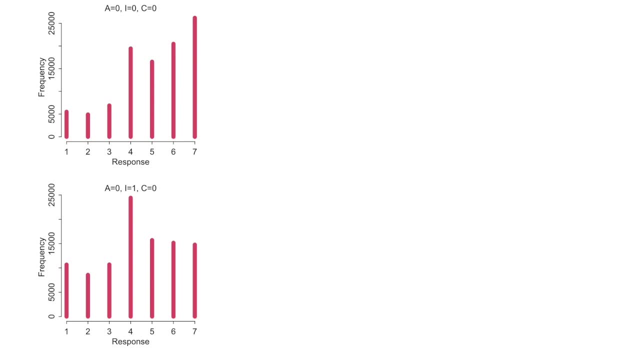 So we take the same story and we add intention to it. What you see is that now it's less appropriate. right, Intention tends to make things less appropriate. That is the average comes down. There's many fewer sevens Now in the middle column here. in both of these I've turned on action, added action. 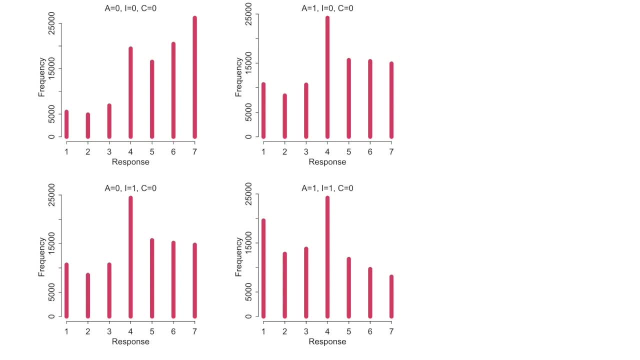 to both stories. So the top still has intention off and the bottom has intention on and you can see what adding action does is it makes things smaller again. Adding action makes people less approving, makes the responses smaller on average, But notice, it's not that it does it to all of them. 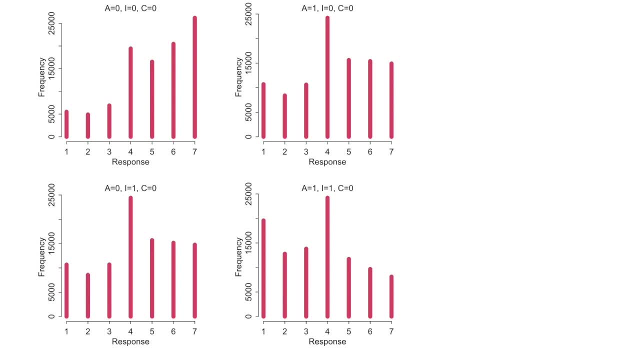 It's because there's this spikiness to the distribution, right where the focal points, like on the end, on number one, are more important and four still dominates a lot. And then, finally, if we add contact instead of action, where contact is a special kind. 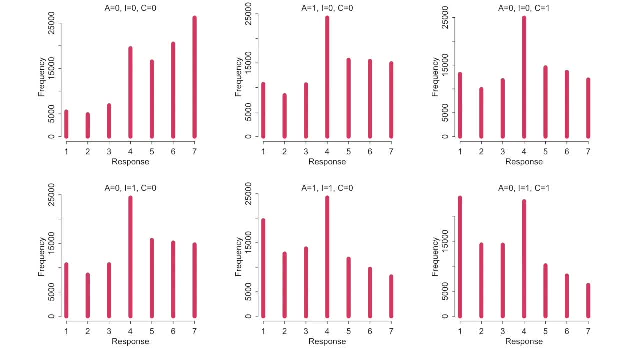 of action. So the way these data are coded, it's mutually exclusive from action, And you'll see that this is the worst of all If you've got intent and contact in the lower right. this is the lowest average of all types of stories in the data set. 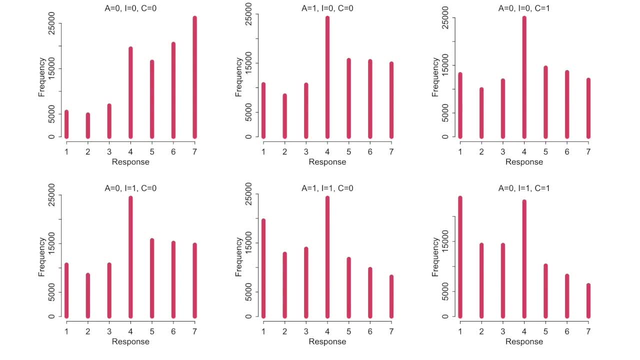 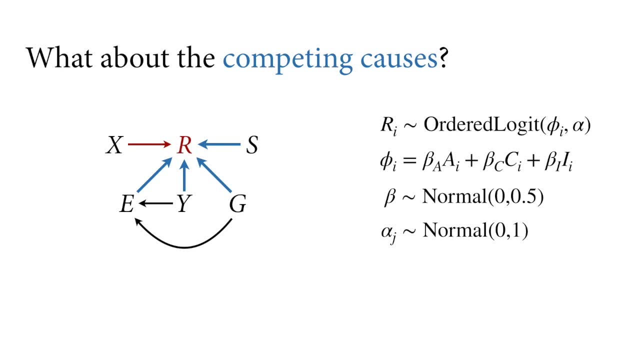 And you get lots of ones. In fact, ones are the most common response. Okay, So we've learned average treatment effects, ignoring all the other stuff in the data. But there's room for improvement. and we've got a second set of estimates. of course, 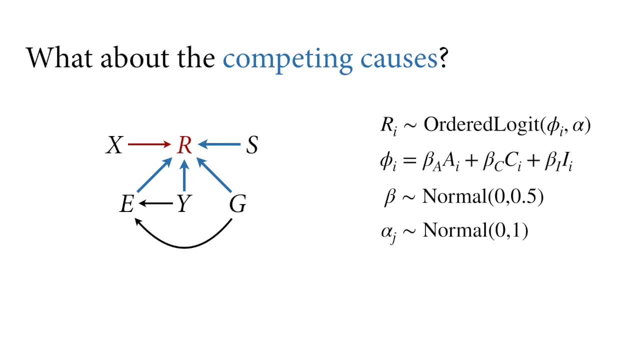 We want to know about how differences between individuals moderate those treatment effects, And so we can take this basic structure and put in some Competing causes, as they're often called. Let's think about a simple one, for example, like the effect of gender. 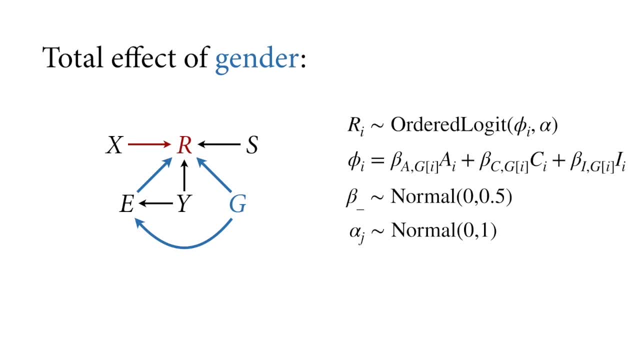 So gender has a direct effect, according to the DAG that I've asserted here, where individuals of different gender may have different average responses to the same story, or maybe just average different responses to the scale or the task, And there's also an indirect effect through education as well. 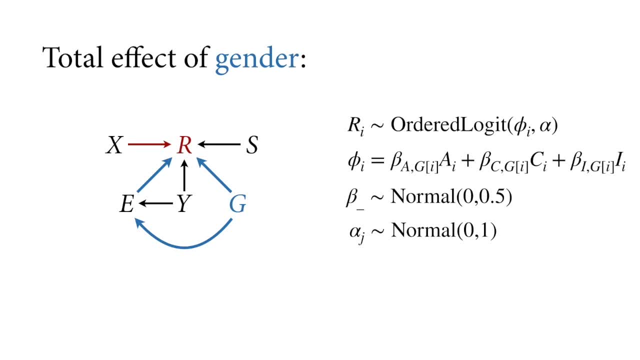 Okay, That is, if members of different genders tend to have different average levels of education and education has a direct effect on the response, then that will also be part of the total effect of gender. So we can add that to the model simply by stratifying each of the beta coefficients. 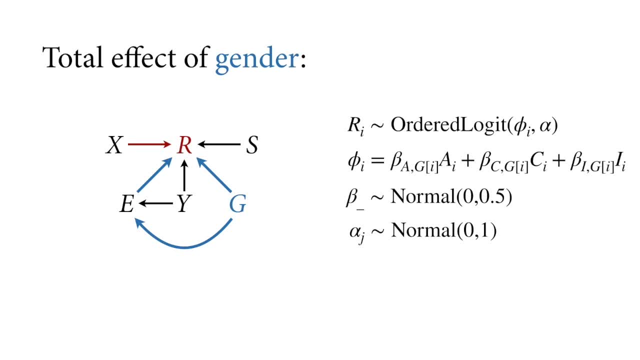 by gender, That is, having two beta sub a's and two beta sub c's and two beta sub i's in this case. So you'll see that I've modified phi. So now there's a subscript in each beta, which is g of i. 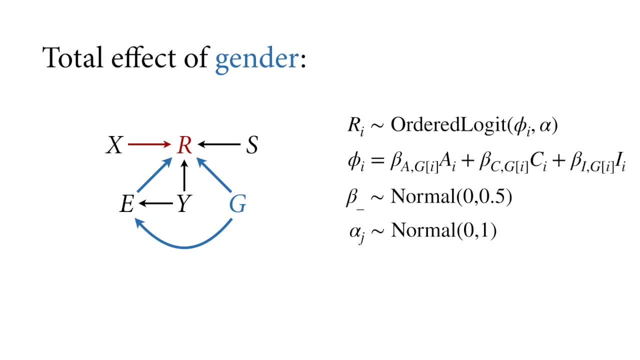 So there's a one and a two there for each of them, And again, every beta in this- this is beta with the line under it. every beta, no matter what its special identity, gets the same normal zero one half prior, and we go back to the. 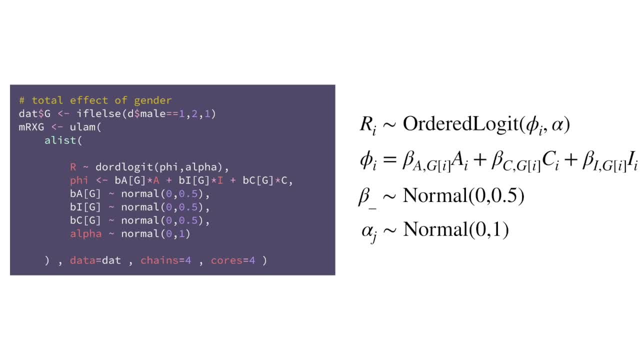 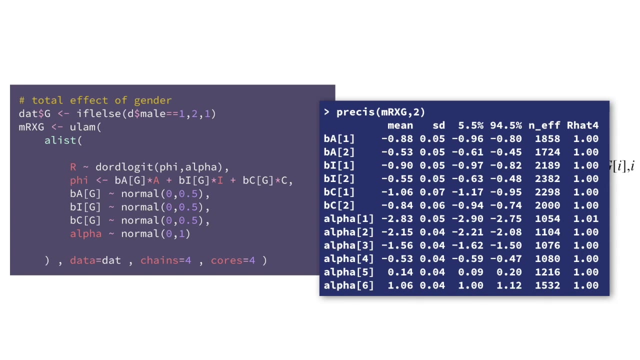 code In Oolam. this is easy. You just bracket each of the coefficients and then you get a vector of them of the length of the unique values in g, And we can run the model again. Okay, And now we look at the pricey output and we have six of these coefficients because 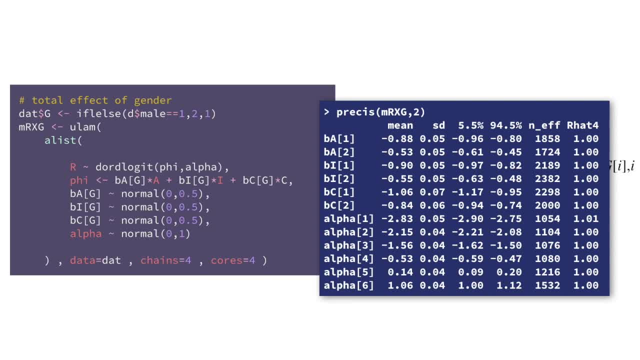 there are three treatments, a, i and c, and then two genders in this data set. So we end up with six coefficients in total And again you can kind of peer at these coefficients and maybe get an idea of what the relative 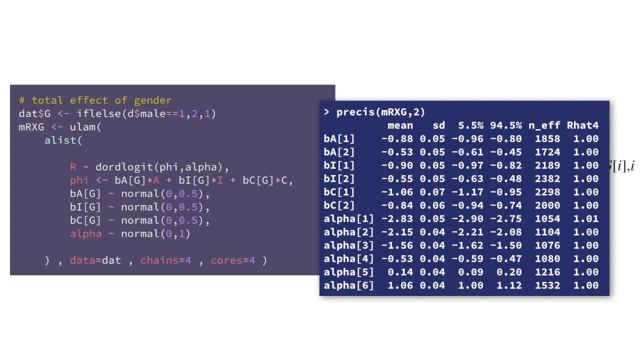 effects are and in which direction. That is basically. all of these things make ratings lower. yeah, They make people disapprove more when you add action, intention and contact, But some things are much worse than others, right? So like, the coefficients for contact are the lowest. 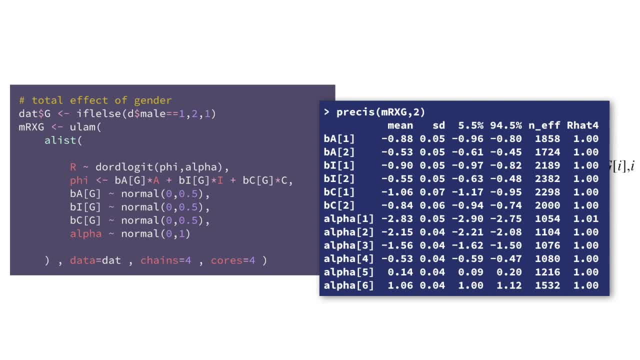 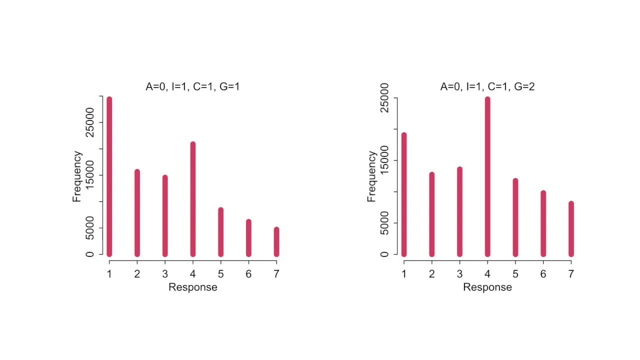 That's because people disapprove of those things the most. But again, it's useful to use the same sort of code as before to push these out on the frequency distribution scale, because it isn't only the average that matters in this kind of model, because you've got spikiness in the histograms right. 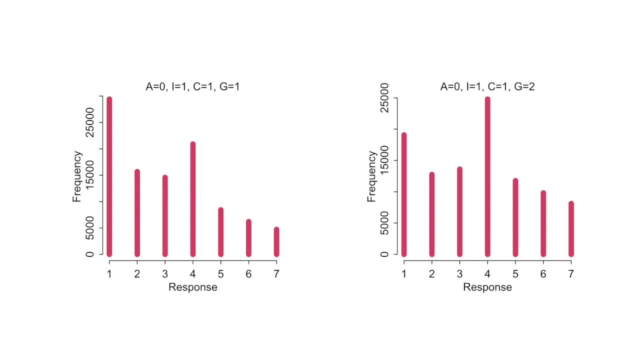 The anchor points matter a lot, But in this case, what I'm showing you. Okay, So for stories which contain contact and intent, which is the kind of story that upsets people the most in these experiments for gender, one on the left which is women, the way I've 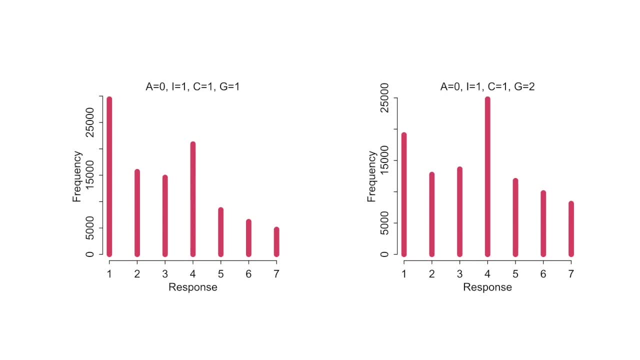 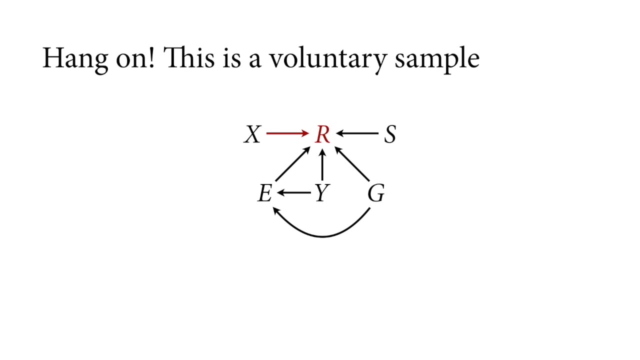 coded it, the average is lower than on the right, for gender equals two, which is men in this, the way I've coded it, Okay, So it seems like by that That Okay, Women in this sample tended to disapprove more than men, or to say it the other way, 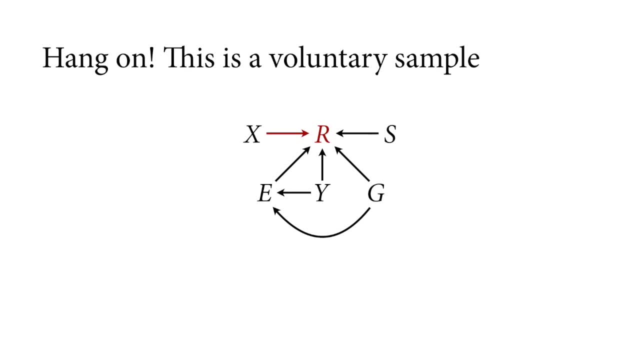 men tended to be more approving of the same stories than women in this sample. But hang on, What is that estimate actually? Let's remember that this sample is a voluntary sample. There were advertisements posted online and people voluntarily in their free time went. 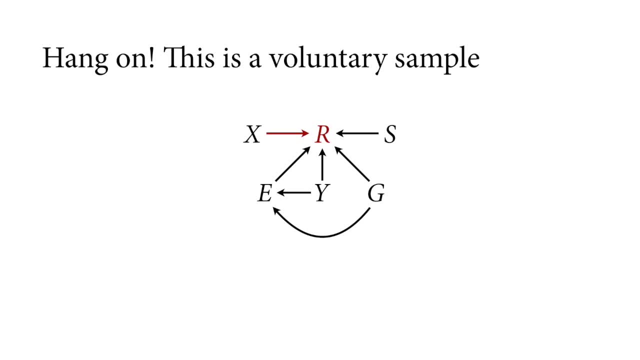 to a website and read through trolley problems, So Okay, So let's try adding that to the DAG. This is something we haven't done before, but you can do this, So it's very plausible in this case, in fact, almost certain, that the demographic features. 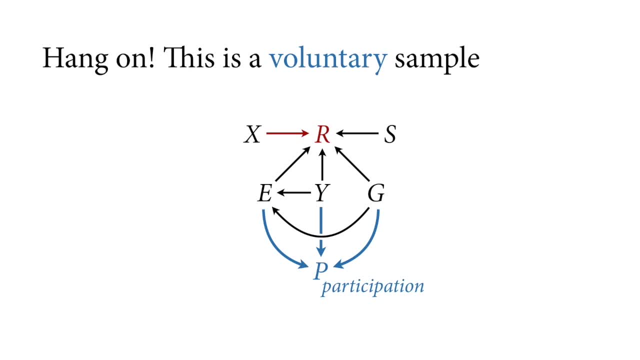 of people, that is, their education, their age, their gender and other things we don't have measured about them. influence, participation- And I've added participation as a node in the DAG. That is the P at the bottom And you'll see that it has causes from E, Y and G. 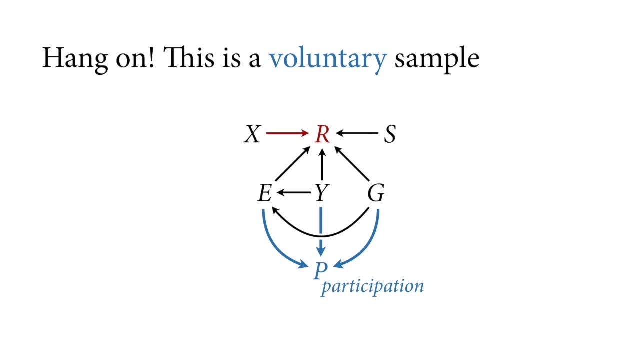 Now here's the cool thing. Well, it depends upon your definition of cool. The sample is automatically conditioned on participation, right? Because we don't have data from people who didn't participate, And P is a collider of E, Y and G, And so, since the sample is conditioned on that collider, 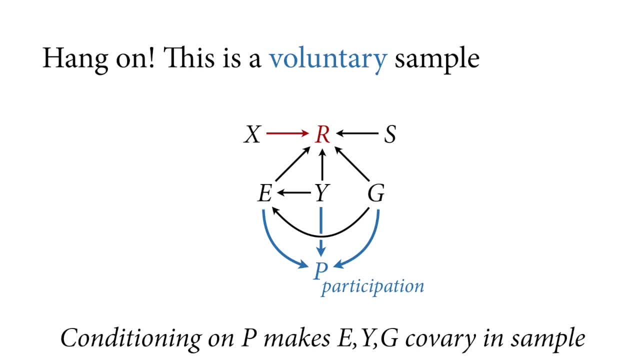 this induces collider bias and, as a result of this, even if e, y and g don't co-vary in meaningful ways in the general population- so, for example, gender and age do not cause one another in any sense- and yet they can co-vary because of recruitment, because they influence participation in the study. 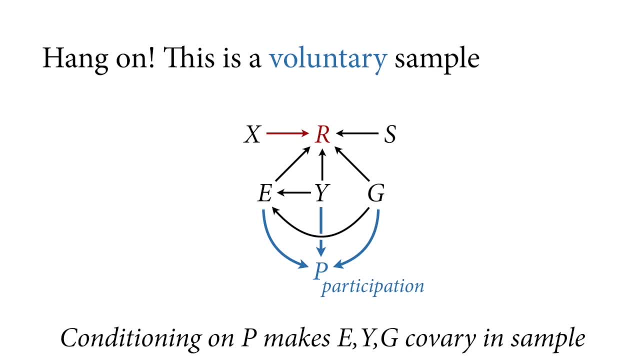 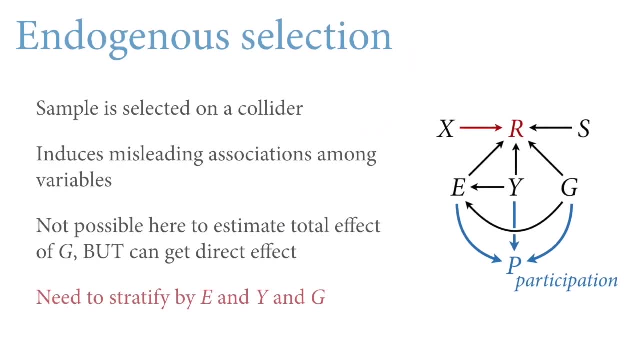 and so our sample can have additional associations among the explanatory variables that will mimic causes, and this is just another way of talking about collider bias. sometimes you'll hear people call this endogenous selection, because it means your sample is already selected. in this case, it's selected on a collider which induces associations non-causal. 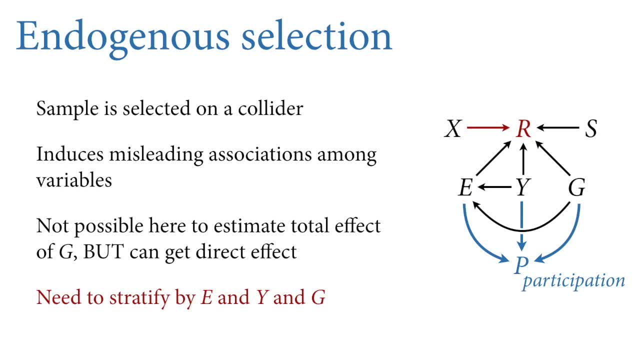 associations among your explanatory variables and these can mislead you. they can be contradictory in the general sense of the term. the consequence of this is that it's not possible from this sample to estimate the total effect of gender. the reason is because it's got confounding paths. 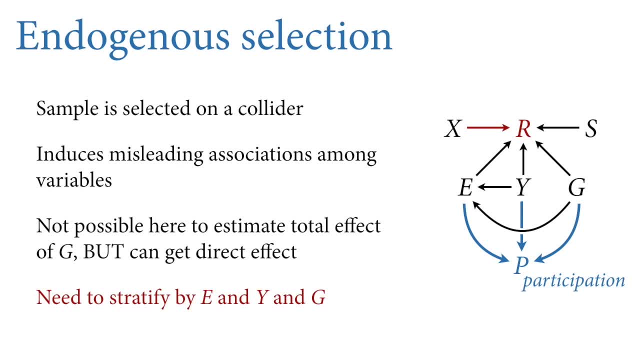 through the collider that connects it to education and age, and so whatever we just measured about the gender effects in those coefficients is not the effect of gender. it's some confounded effect of gender. almost certainly that is a result of the fact that gender and age and 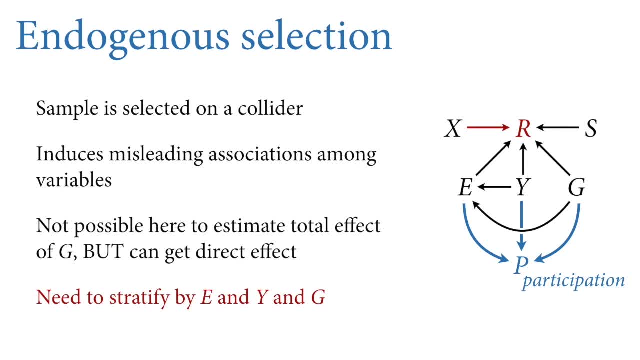 education are all influencing participation in some way, so it's not really interpretable as a total causal effect. but we can get the direct effect of gender in this case, because we can stratify by education and age and block the collider contamination. and if you analyze the graph with your eyes, i i hope you can see that by now you've gotten practice at this. 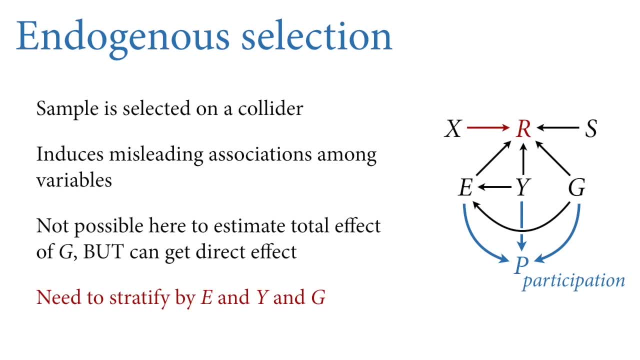 but if you're not at that level yet, that's fine. i encourage you to fire up a little bit more of a tool like daggety at daggetynet, or use the the daggety r package. put this dag on this, slide into it and then ask it for adjustment sets for different queries and it'll tell you that it is. 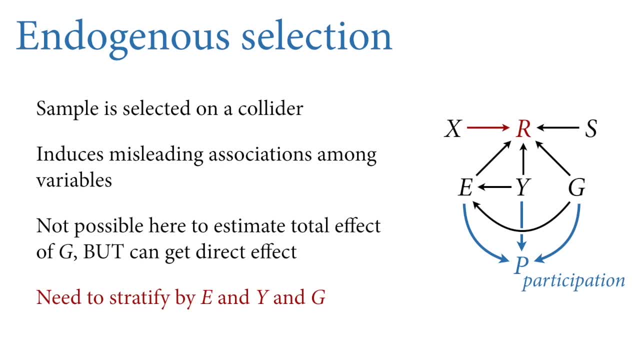 possible to get the direct effect of g but not the total effect of g, and the reason is because of participation. we've already conditioned on participation, so we're going to stratify also by education and age and gender simultaneously. that's what we have to do to answer our s demands, but there are things we can't get. we can't get the total. 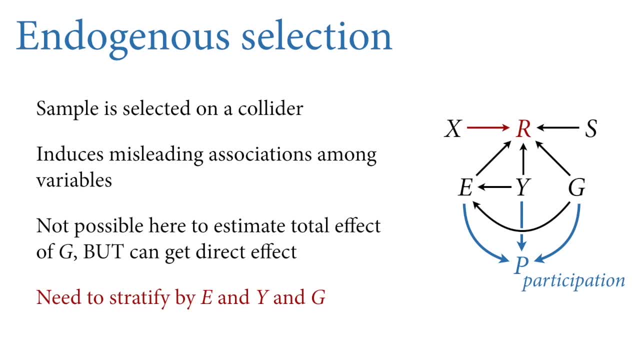 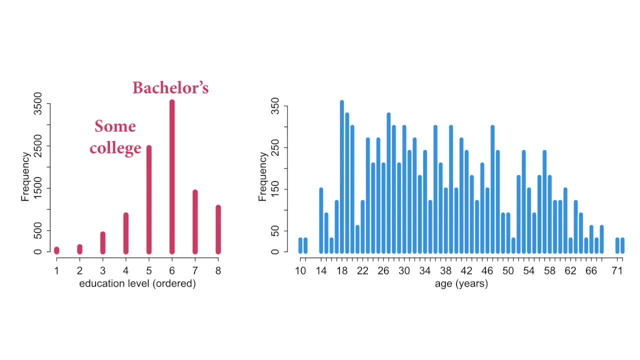 causal effect of gender and we also, by analogy, cannot get the total causal effect of age, because it is also similar, for the same reason, contaminated by the collider bias. let's look at these variables- education and age- now, and their and their distributions in the sample. it's pretty obvious. 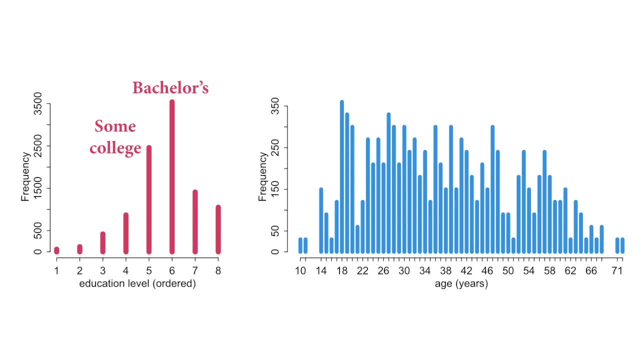 that this is not a random sample of the population and very plausible that these variables are partly driving participation. so on the left in the red i'm showing you educational level. this is an ordered variable. it's like the outcome, it's ordered, but it's it's educational level. one is: 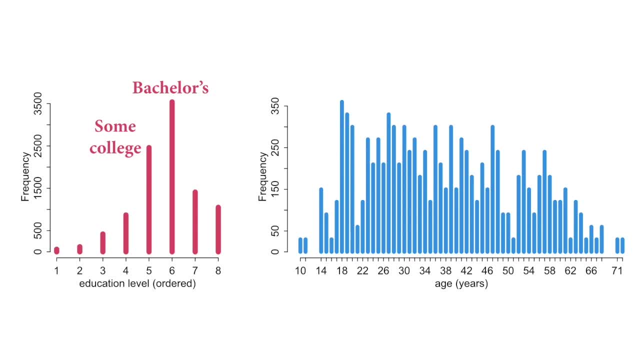 elementary school and eight is having a doctorate, a phd. the most common values in this sample are some college five, uh and the and having a bachelor's degree, and that's because college students are the main participants of this experiment. it was advertised at universities and then on the right you look at the age distribution. this is not the distribution. 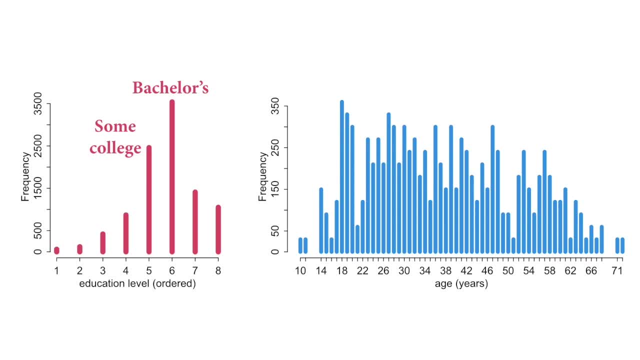 of uh, of of any country this experiment had had significant participation from. in fact, it's not the age distribution of any human population, right? uh, it doesn't look anything like this, but that's okay, you can still make inferences with non-random samples. you just have to. 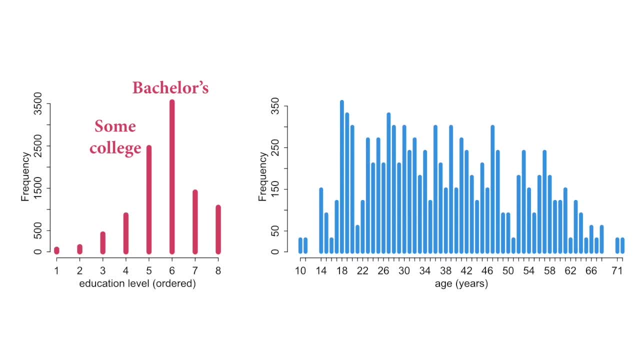 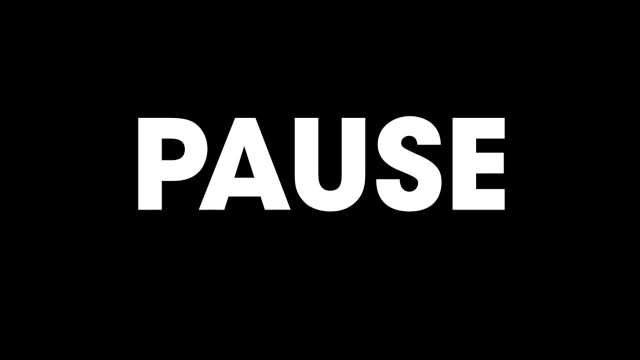 think carefully about whether which particular s demands are confounded by the possibility that these features are driving recruitment in particular ways. okay, that's a lot. we've learned some basic machinery of the ordered logit model and thought hard about what is actually a fairly complicated causal structure. 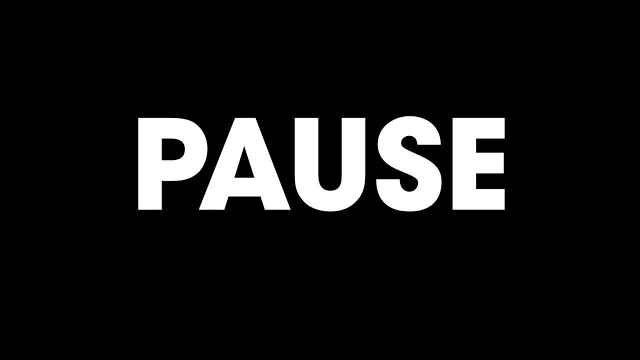 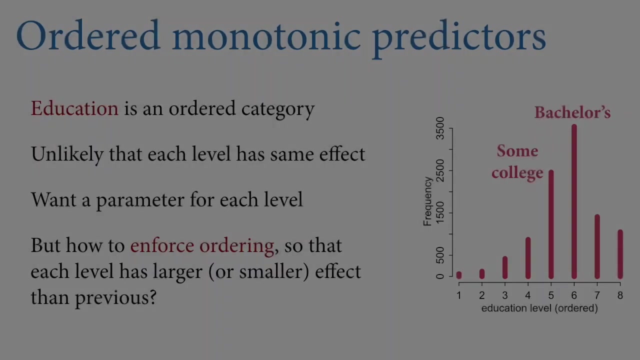 even though it's an experiment. so i think you've earned a break. why don't you take a walk, have a cold or hot beverage as you prefer, and when you come back i'll be here. all right, welcome back. let's pick up where we left off. before the break we were talking about 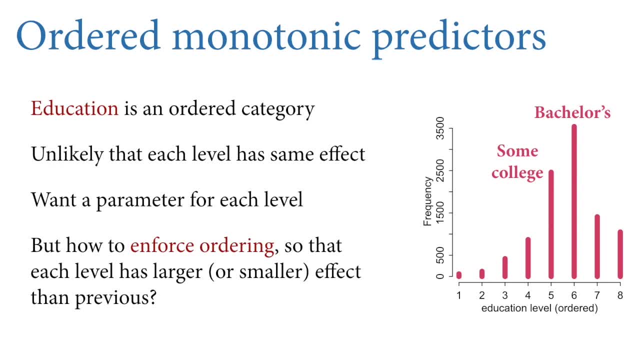 two of the predictor variables, education and age, and adding them to the ordered logistic regression. let's talk about education for a while, because there's an interesting feature about the education variable, as i mentioned before the break, is that it's also an ordered variable, like the outcome. 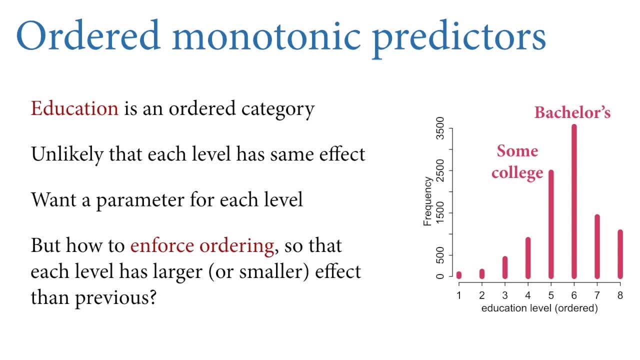 but it's not a subjective response. it's an objective measurement of how far each person has gone in their education. well, it's self-reported. it's a self-reported measure of how far each person has gone in their education, but it's ordered because of course there's a progression from. 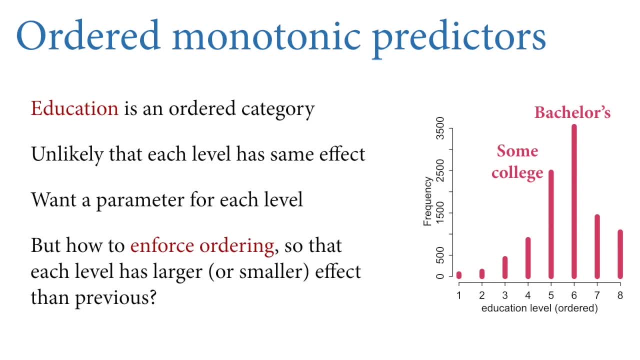 elementary school to middle school, to secondary school, to college, to master's degree, to PhD and so on- hd- and that it creates an ordering that we want to pay attention to and like the outcome it's. it's unlikely that each level has the same effect, in the sense that there's no constant distance. 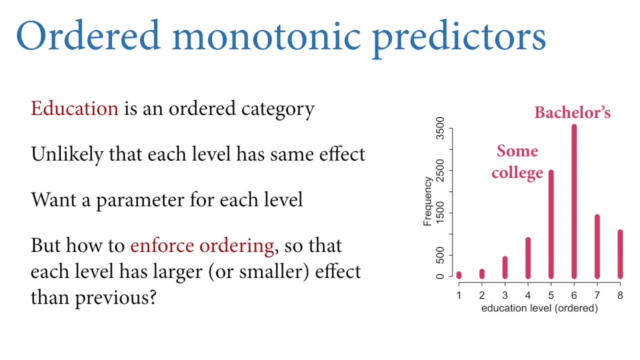 in, in effect, in this case, between one and two, and two and three in the education variable. so there's an obvious and extremely useful solution to this problem. for predictor variables, i remember our goal is to stratify the outcome by the levels of the education, and so we can. 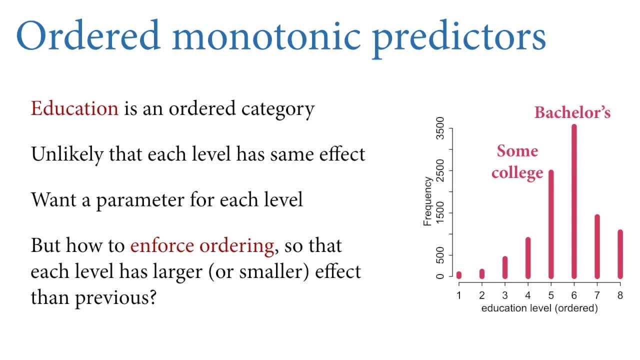 easily do that. we can just have a different parameter for each level of education and estimate it, and in principle that's no problem. we have a lot of data here. it'd be no problem to have seven parameters for education. we only need seven, even though there are eight levels of the 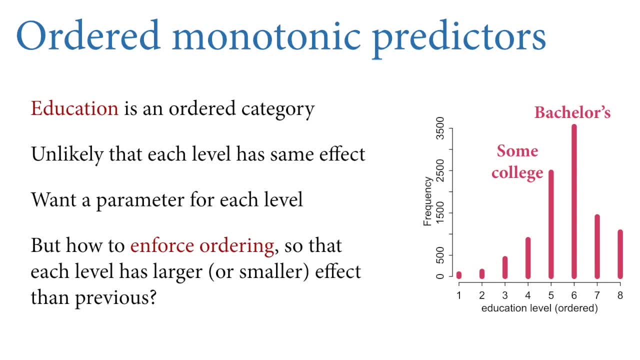 education variable, as you see on the right, because one of them is already- is in a sense free. it's already accounted for by the cut points, by the alpha parameters, but we'd also like to enforce an ordering, that is, we'd like the effect of education to be monotonic. 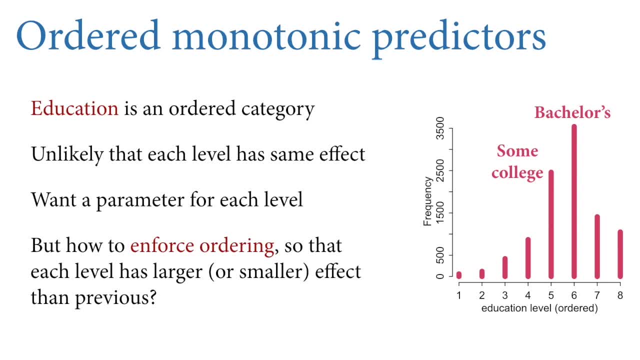 and that means either always increasing with increasing education or decreasing with increasing education, that is, its causal effect on the outcome should be monotonic, and this is nice because it'll make estimation more accurate and it's the kind of functional assumption that often gives us a way to identify causal effects when it's accurate. so what we mean to do here, to enforce 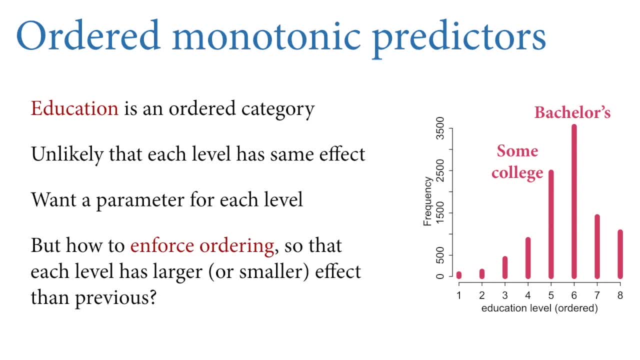 some ordering to this is make it so that each level adds an increment. let me break that down in the next several slides and show you what what i mean, but before i do that, i want to tell you that this is a very industry standard, if you will. way to treat ordered. 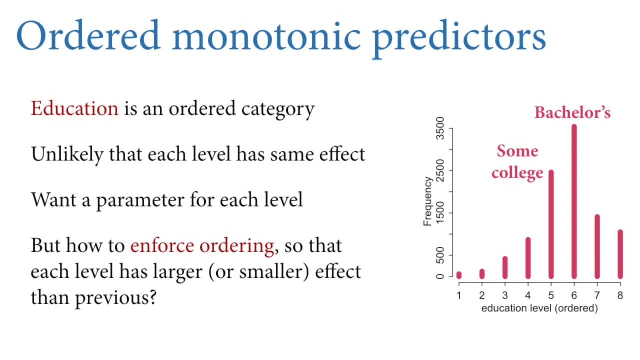 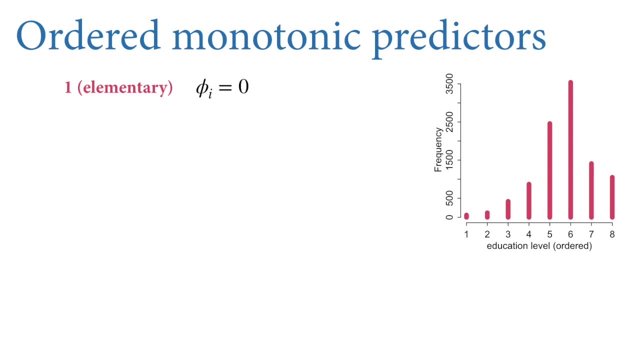 predictors, that is, if you have an ordered variable, an order categorical variable, on the right hand side of your regression. this is an extremely common and useful way to include it in your model. so let's consider the first level of education, which, in this data set, is elementary school. having completed elementary school, 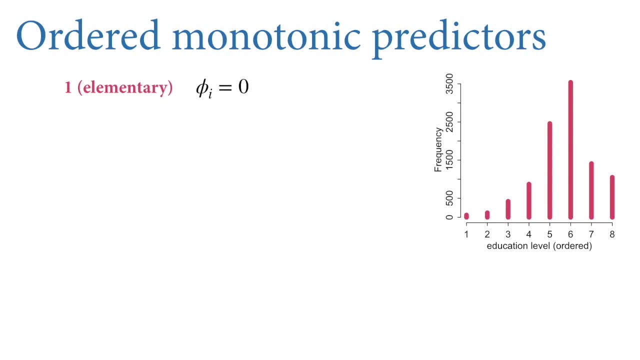 and we're going to consider, we're going to construct this example thinking of there being no other predictors in phi, the linear model of our ordered logit. and so phi sub i equals zero in this case because, as i said, the first level of education is in a sense free because its distribution is. 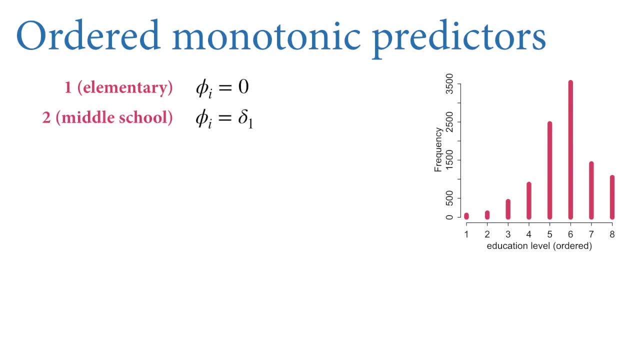 taken account of by the intercepts, by the alphas. but what about the second one? well, for the second one, which is middle school, in this data set, we're going to add a special parameter for it, which i'm going to call delta, and it's delta sub 1. 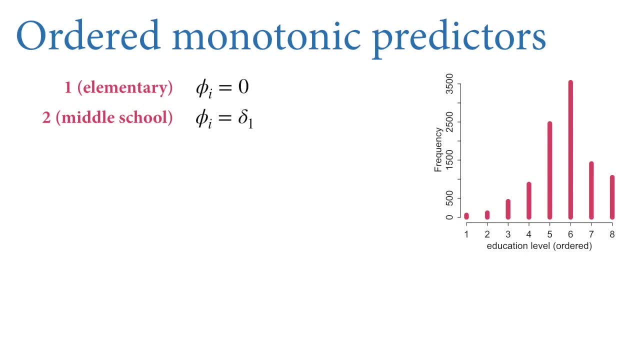 there will be a series of deltas, one for each level of education above the first, and so we we move the cumulative log odds of uh, the outcome variable, by delta sub 1, and the model needs to learn if delta is positive or negative. and then for some high school, which is level three, 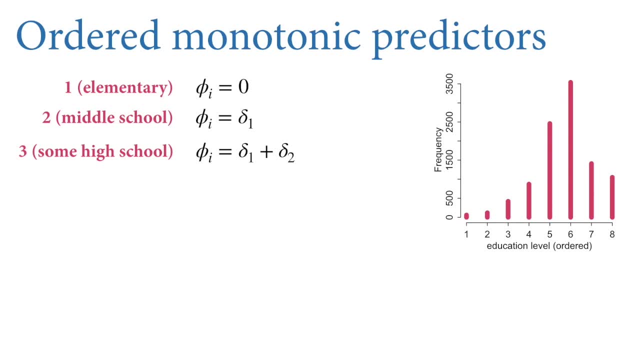 delta 2 is a new parameter that's specific to the increment of some high school, and so this is what establishes the monotonic ordering of the causal effect of education is that we're going to keep piling up these deltas, and so for high school, which is level four, it's delta sub one plus. 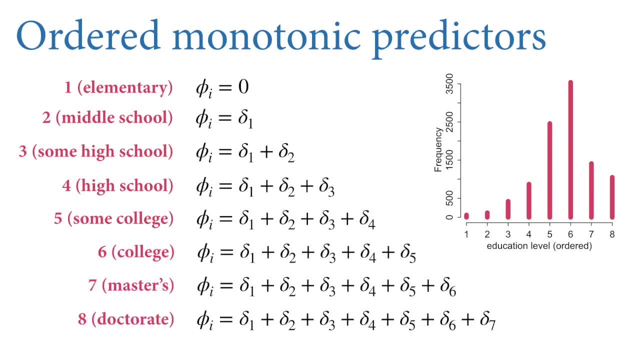 delta sub two plus delta sub three, and so on. for level five, there will be four deltas and for level six, there will be five deltas, and for level seven, there will be six deltas. and uh level eight, the doctor at the highest level, there will be seven. for this last uh level, the doctorate, it's very 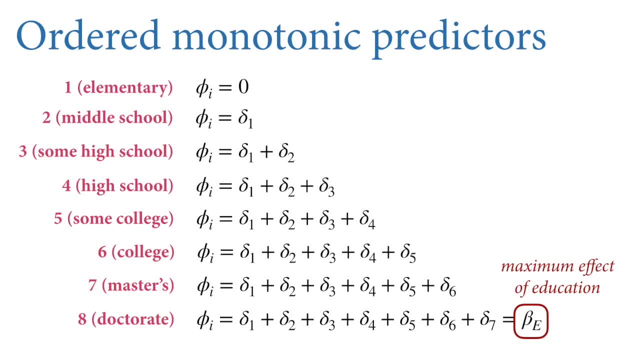 useful to transform these deltas by first saying that if you sum them all up, they equal a parameter, beta sub e, which is the maximum effect of education. remember, this could be positive or negative, you know, because education could increase the acceptability of stories to people or it could decrease it. 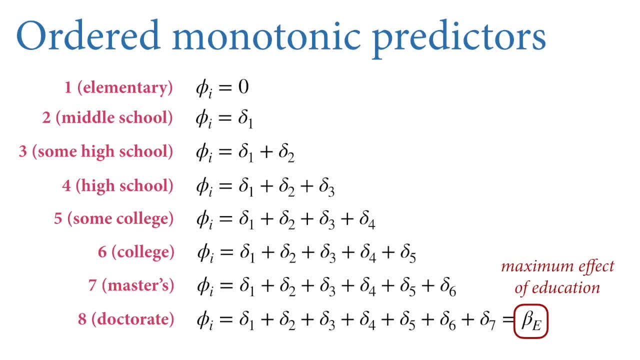 and then what we're going to do next is we're going to transform the deltas so that there's something called a simplex. i'll say this again, so hang on if you haven't gotten it on the first pass. so we're going to say that there's a little imaginary parameter: delta sub. 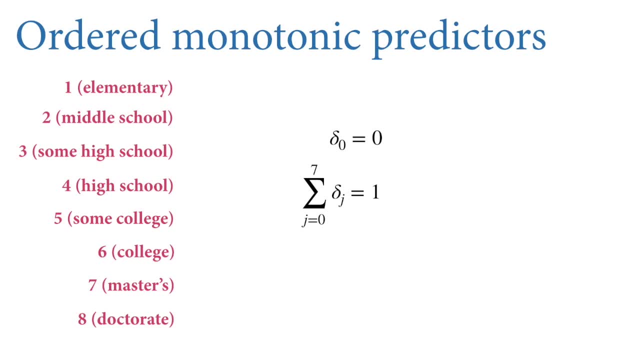 zero, which equals zero, which is the effect of the first level of education, elementary. and this is just a placeholder to help us remember that the first level of education is taken care of by the intercepts, by the alphas, and then for all the others, uh, we're going to say that they sum to. 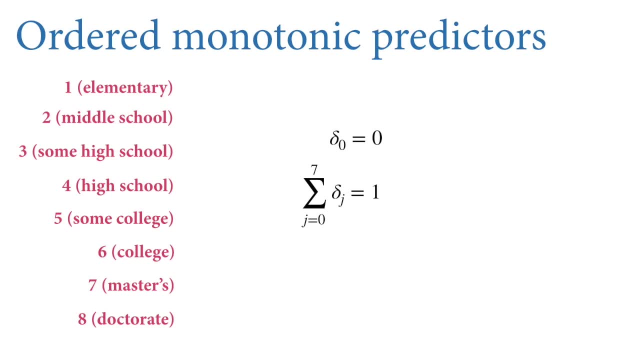 one. we're going to enforce this actually. so if we sum from zero to seven, all the delta sub j's, from j equals zero to seven. we make them equal one. why are we doing this? well, because it lets us set phi, our linear model, with a simple linear model, so we can get the sum from zero to one, and then we can. 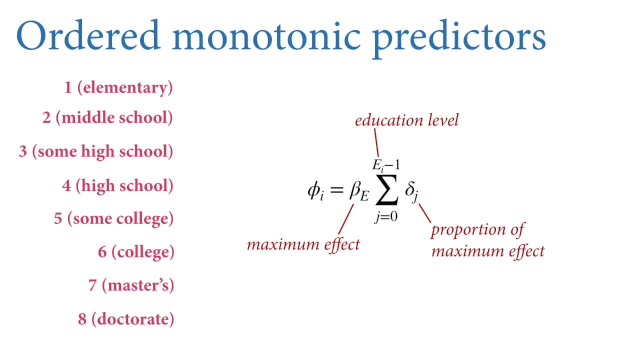 kills, Tôi vẫn sẽ tr? yay. rồi đềm realize, Goodness, if you didn't focus that I have five minutes left, not a second, over the Shar nok menα, and this is what we're going to do. let me explain this to you so, phi. 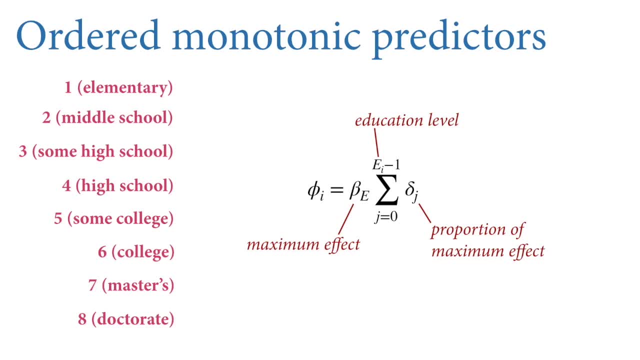 will equal now, data sub e, which is the maximum effect of education multiplied by the sum of all the deltas up to the educational level of the individual on row i. I'll canulous cries say that again. so phi sub i, which is the adjustment to the cumulative log odds for k psi. 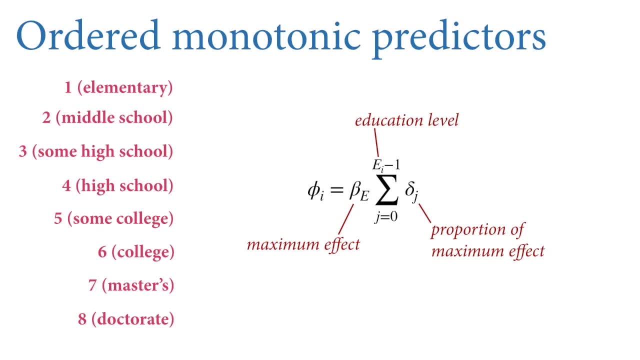 will be equal to beta sub e, which is the maximum effect of education, and this we estimate. this, remember, times the sum of all the deltas, where the deltas are these proportional increments from each educational level, but only up to the educational level of the individual, and you'll notice it's, it's e. 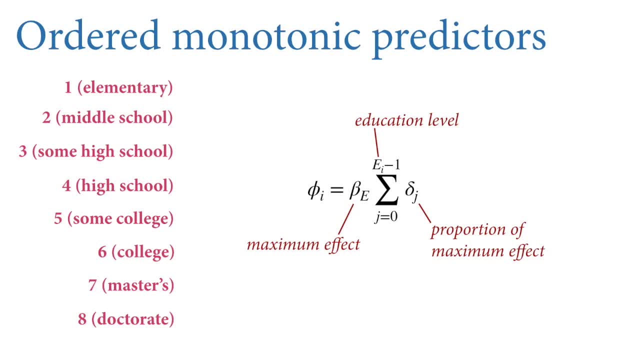 sub i, which is the educational level of the individual, minus one, because remember, the first level, elementary, is kind of taken out of this. it's assigned in an index of zero and so the Delta sub J's only go up to the maximum level of education minus one. so if you have a doctorate you sum up to seven because 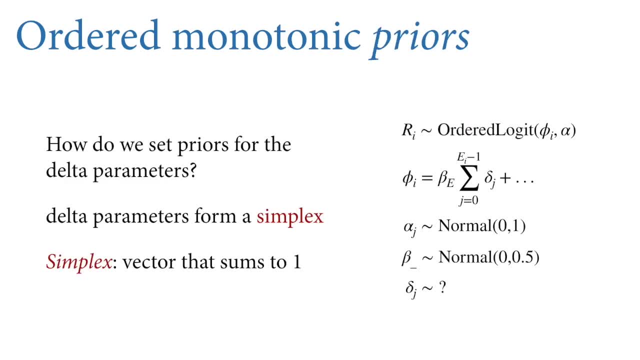 that's the length of the Delta vector. okay, I know that that maybe seems a little weird, but really all it is is a standard additive model where we've just scaled the Delta so they sum to one, because it makes it possible for us to summarize the order of the deltas and the sum of all the deltas and the sum of all the. 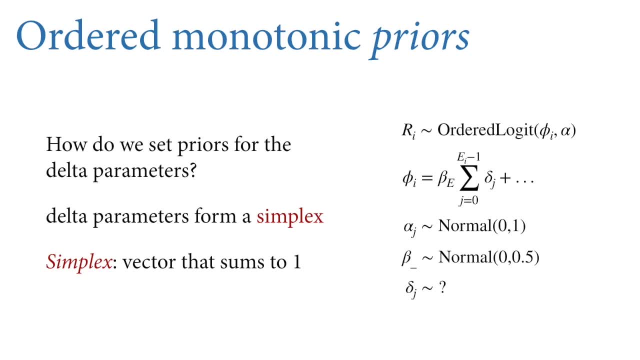 overall effective education by this beta sub e in front. it makes it easier to think about that and it's often much easier to assign priors that way because we can assign a sensibly size prior to beta sub e, because we might have good scientific information about the maximum effect of education on such a thing. but 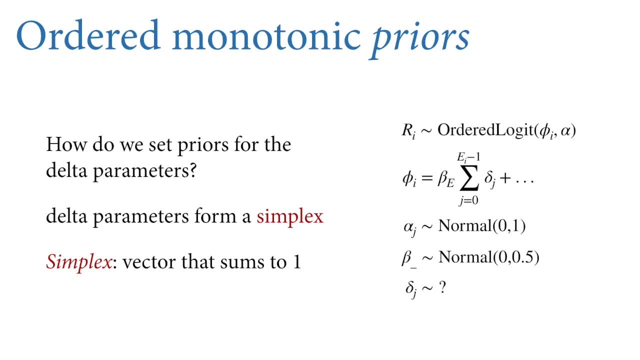 even if we don't, it's much easier to assign, assign sensible priors to the maximum effect than it is to each incremental effect. still, oh, I should say before I explain that, as I said, these Delta parameters now form something called a simplex, because we've made them sum to one, they're constrained. 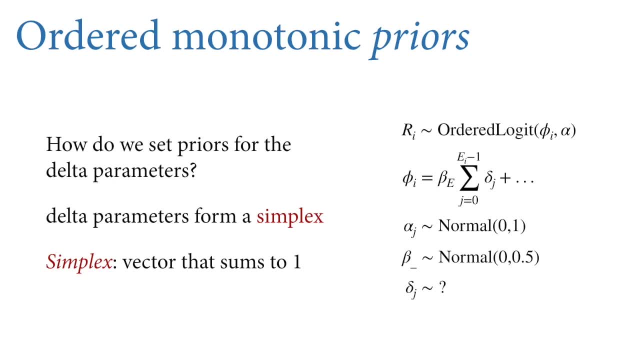 to sum to one. a simplex is just a name for a vector of real numbers that sum to one- which, if you're paying attention, means there are also probabilities- can be interpreted as probabilities and this leads us to finding a prior for them. now we need a prior for each of these Delta sub J's. 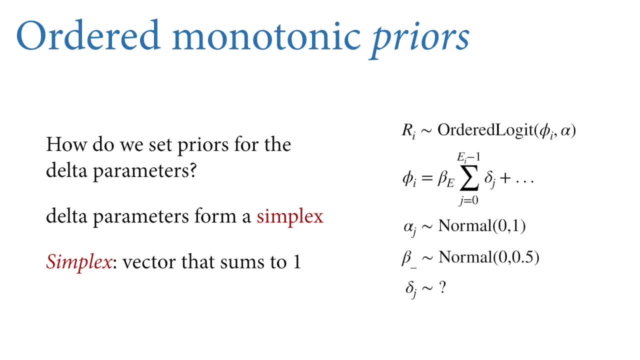 as I show on the right in the mathematical formula of the model at the bottom word. what do we replace that question mark with? well, it turns out there are probability distributions for probability distributions. I'll say that again. it turns out there are probability distributions for probability distributions and the meaning that we draw vectors of numbers that sum to one. 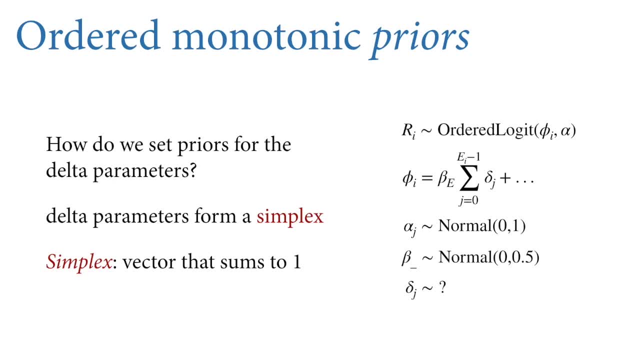 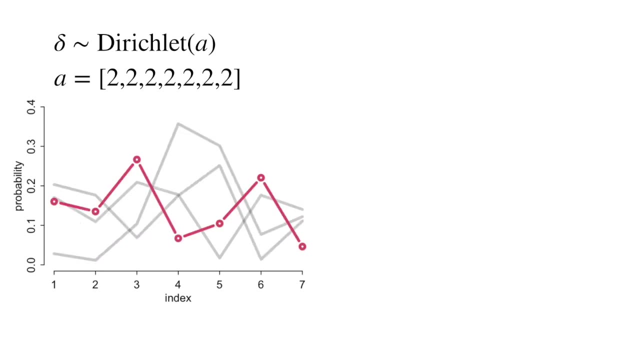 because that's what a probability distribution is and that's what we need as a prior for the vector of delta, sub e deltas, so that they're still constrained. to sum to one, the most famous distribution that meets our criteria is the Dirichlet, and Dirichlet is named after a Belgian. 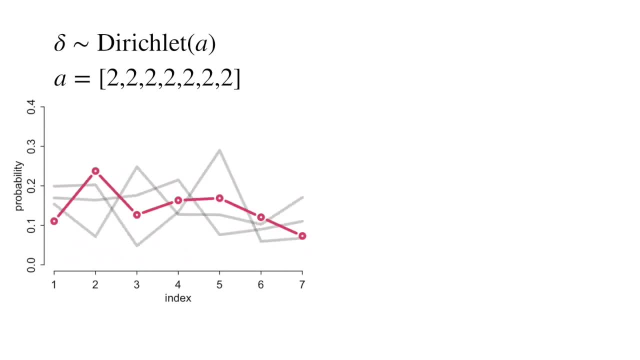 German mathematician who did lots of really important work in in pure and applied mathematics, and this is just one of the things named after him. the Dirichlet distribution um takes as its input- that gives it its shape- a vector of the same length as the number of categories you want. 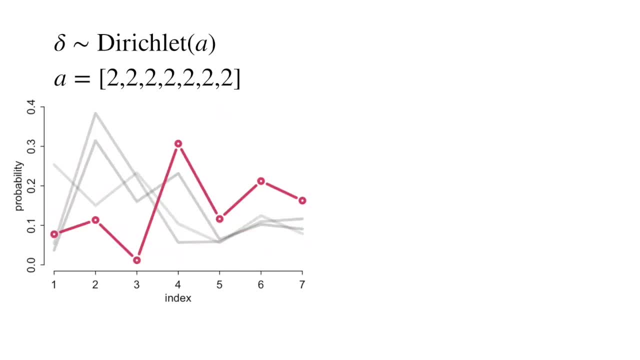 to draw probabilities for. so we want seven, we want a delta of like seven, because there are eight levels of education- remember the first one's free. so we only need seven parameters. and so we want to assign our vector, Delta, which is uplinked seven Dirichlet distribution, and its shape is given by: 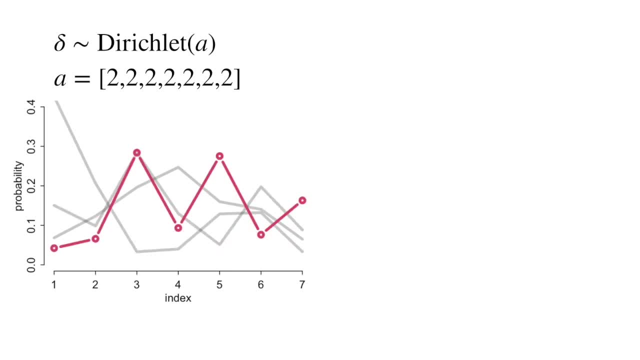 this parameter, a here, and a is just a vector here of seven twos. what do these twos mean? well, you could probably guess, because they're all the same value. that means a priori all of the possible levels of education, or or have the same a priori effect increment, because that's what we're drawing here. 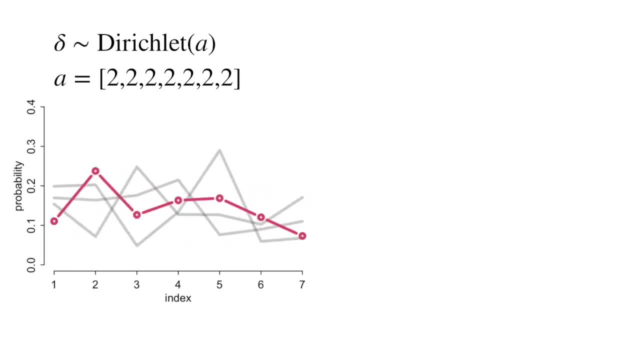 right is proportional incremental effects, a proportion of the maximum Beta sub e. so we assign them all two and that means a priori every level has the same effect. but the size of these numbers in the a vector determine how much variation there is across. so I'm animating here: draws from this. 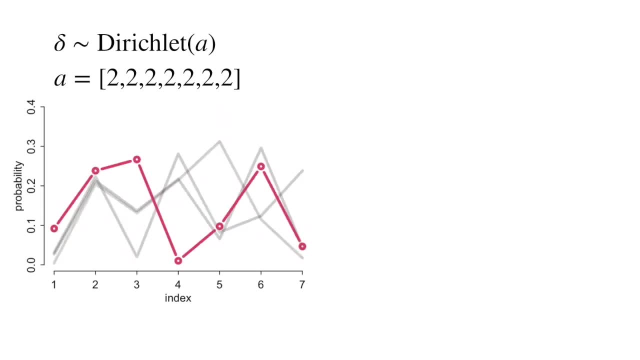 Dirichlet distribution with, where the shape is given by a vector of seven twos, and you'll see that they're hardly ever equal, even though the twos are all the same. the independent draws jumble all over the place, and the smaller the numbers in the a vector, the more variation there will be, the bigger the. 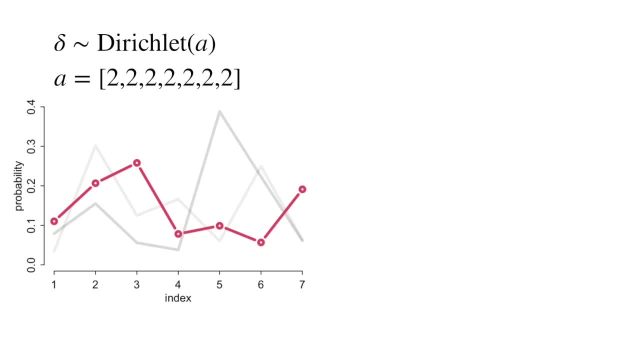 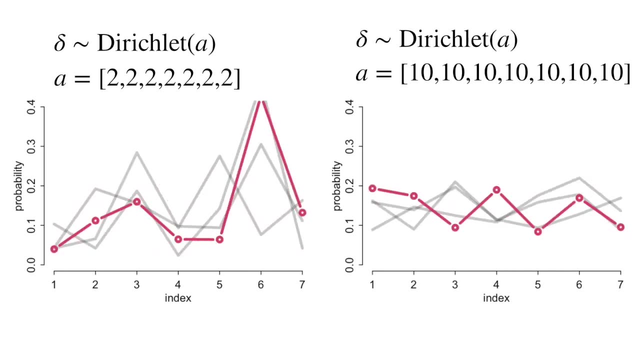 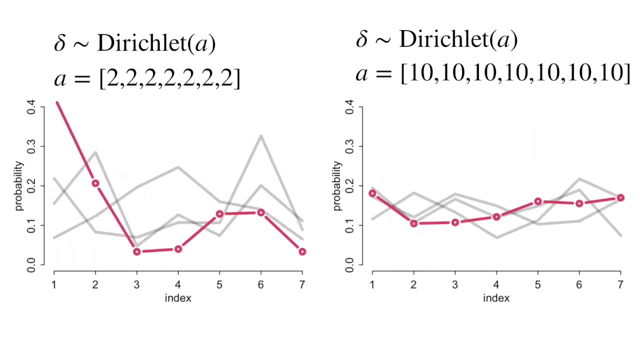 numbers get. the more similar, the flatter the distribution gets. so let me show you: if we make the a vector, seven tens instead. instead, you'll see that now there's much less jostling around and this is like a prior that expects a lot more similarity among them. we don't really expect the increments of every. 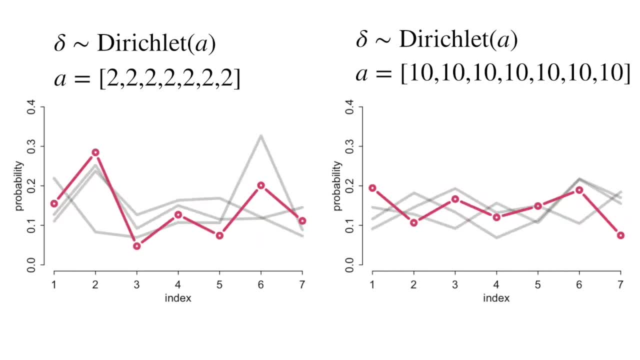 educational level to be the same right. the impact of elementary school and college are probably not the same, so I'm gonna stick with the prior on the left. but before we stick this in the model, I want to show you one other thing: the primary intuition about the Dirichlet. 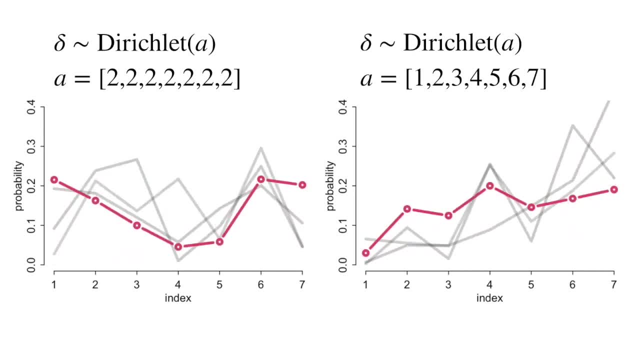 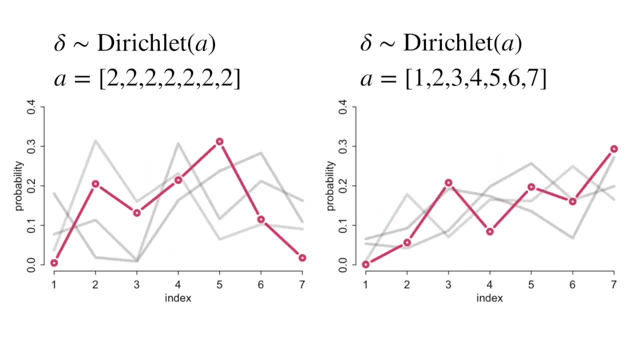 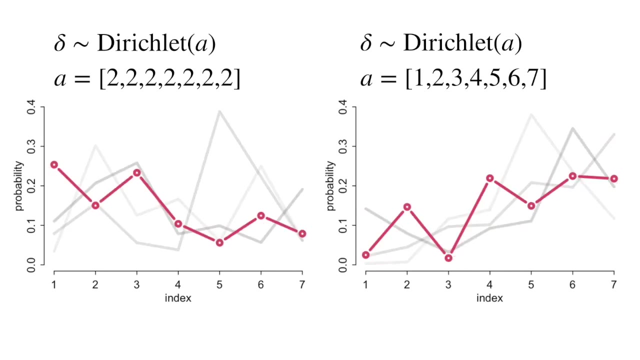 distribution is that the a's don't have to be equal. so here's on the right, drawing vectors from the Dirichlet, where a is set to be the integers one to seven, and now you'll see that this means that the, the higher values, are given higher probability, right, because they have 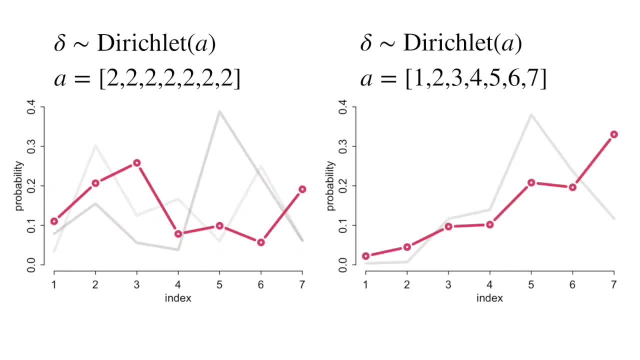 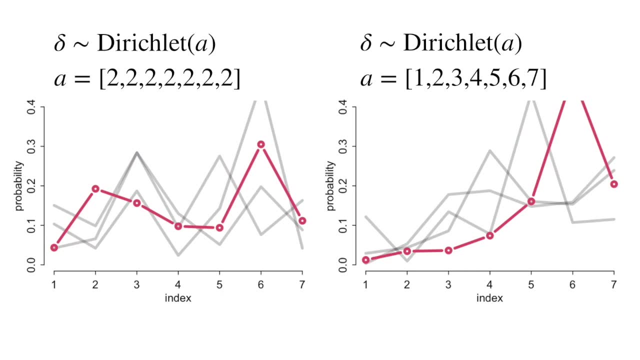 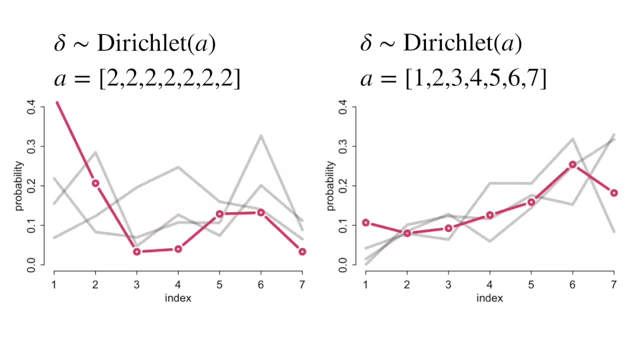 higher numbers and you can do anything in between and you can even have fractions in the a vector as well. those of you who know the beta distribution, the Dirichlet is, is a generalization of the beta distribution. the beta district or you could say the beta distribution is a Dirichlet with only two events: an a. 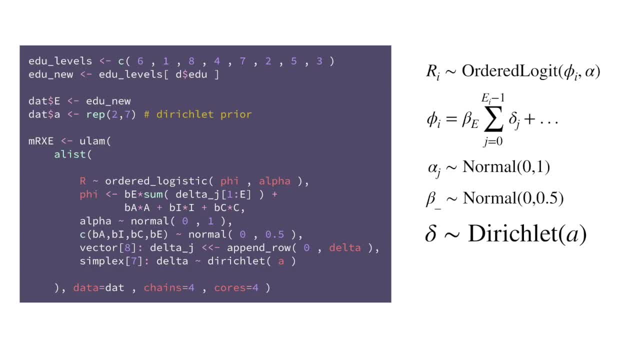 vector of length two. okay, Dirichlet is very useful. it pops up in lots of applied problems and it's going to solve our problem here, putting a sensible prior on the on the vector of deltas so that they still sum to one. here's the ulam code to make this work. 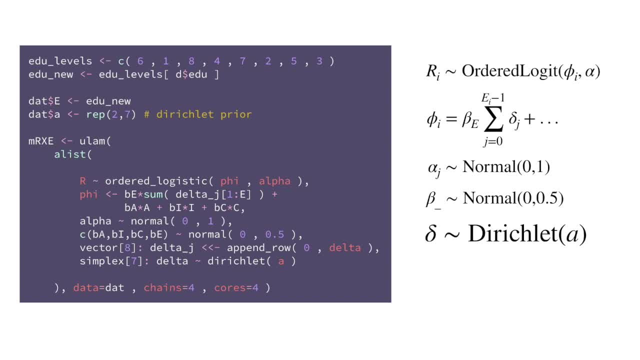 the top of the code box. on this slide I merely extract the educational levels from the raw data. unfortunately, the factor codes in the raw data are not ordered properly as education proceeds, so I have given you the educational levels in their proper reordering and done that for. 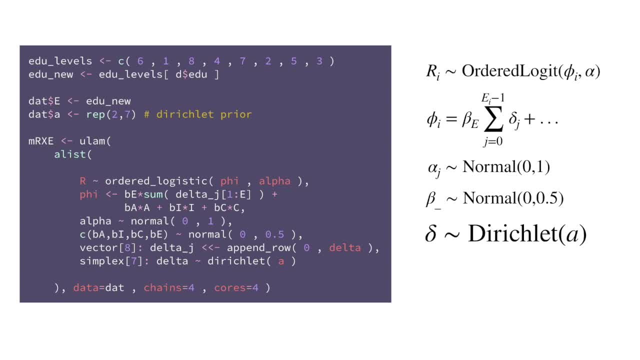 you in the variable called ed- you knew which- which represents education as a proper ordered predictor. and then we're going to feed the Dirichlet- prior that is a vector of seven twos- into the model as data. and then there's the ulam code where you see, in the line for fee, our beta sub e times the sum, literally we use. 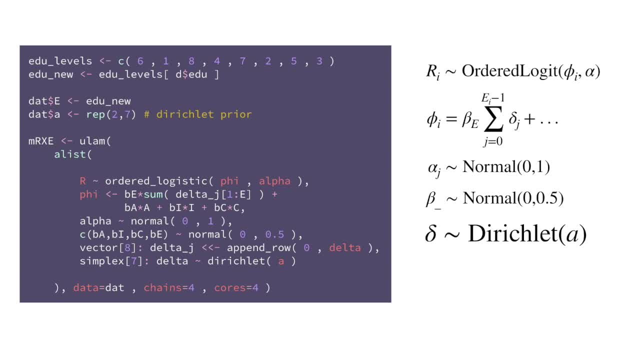 a sum function of the Delta J vector up to the individuals educational level and and then the rest of the linear model, the, the action, intention and contact effects are still there and at the bottom of the ulam code you'll see that there's a little bit of housekeeping to do to build up the Delta J vector. we 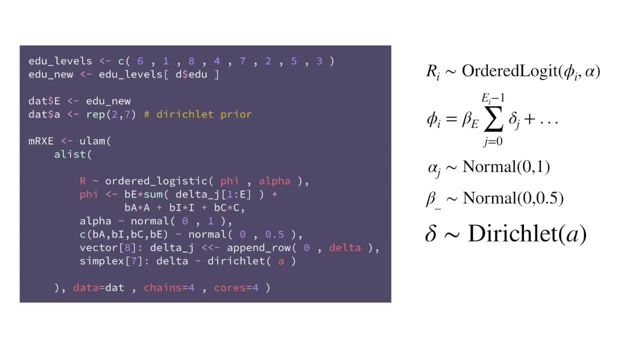 were at first. this append row command is used to put the zero on the front of it. that's for the first level, the, the elementary school level, where the if the increment is zero, always because it's taken care of by the alphas, and and then at the very 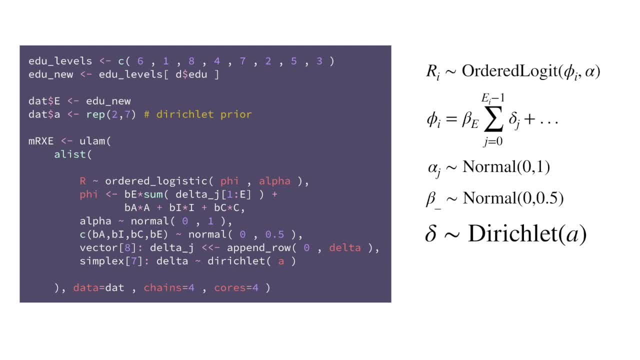 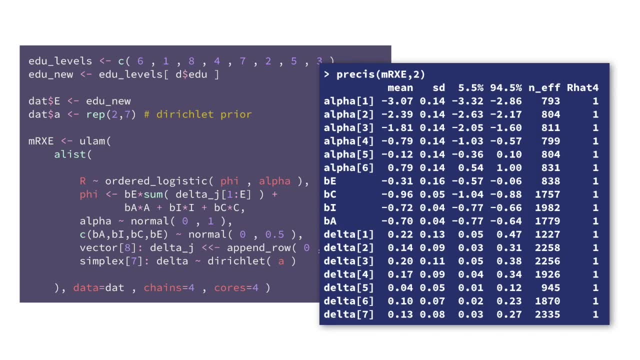 bottom we define a simplex of link 7, which is the deltas, which is given the dirichlet distribution. run this model. it mixes quite well and shouldn't take too long to load, i mean to finish mixing, and again you can look at the, the pricey output, as always, and it's a bit mystical, but and you 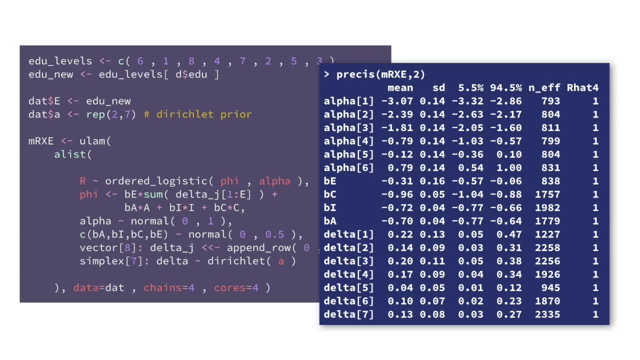 probably shouldn't spend too much time staring at this, because that way lies madness. but you can see the seven delta parameters that have been estimated at the bottom and that they are proportions, because they are proportions of the total effect b, e, which here is negative, which indicates that higher education tends to 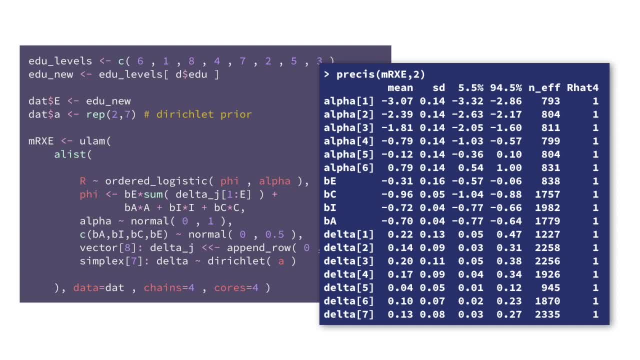 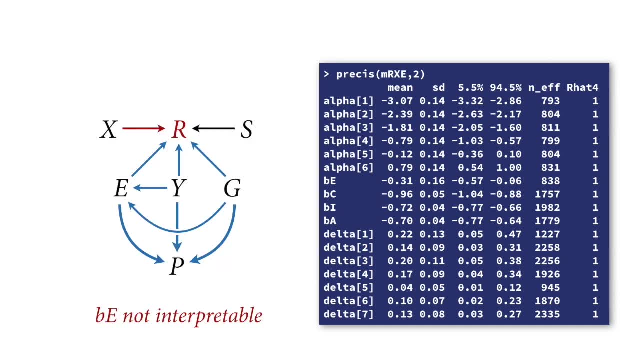 decrease. how, like, how appropriate people think the stories are on average in the total sample: okay, but there's a problem interpreting this because of the fact that the the sample is well selected, probably on the demographics. on education, remember, the college students are vastly overrepresented and probably don't think like most of the population- not my experience. 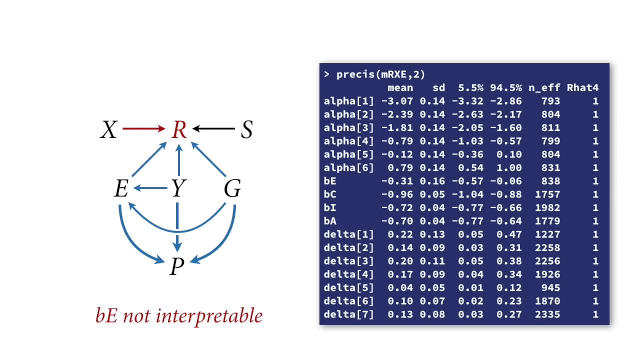 and so we've got this conditioning on a collider on participation which creates these um non-causal associations between education and the response. in other words, there are non-causal paths associating educational levels with responses through age and gender, and so we can't interpret be here as the causal effect of education. that would be unwarranted. 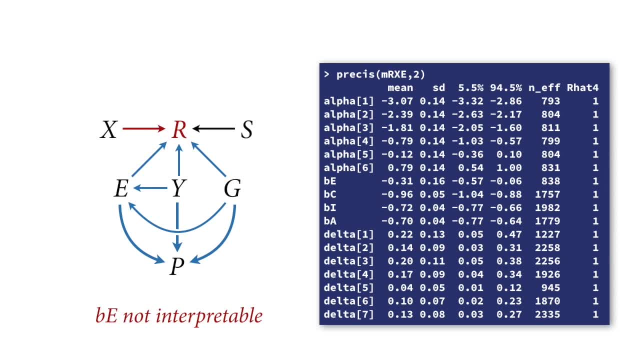 so i hope this this re-emphasizes to you how important it is to think about how the sample is caused. right. it's not just the process by which people make ratings of these stories, it's it's the process by which people ended up in the data set that we're modeling. 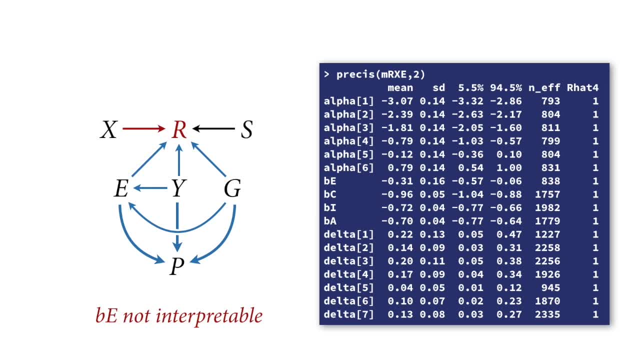 with the dag here and that affects our interpretation and construction of statistical models. so what do we do about this? well, we've got to add the other predictors. if we we we can identify through the backdoor criterion, we can identify the the effect of education if we simultaneously stratify by age and gender, like: take a look at the dag, reassure yourself. 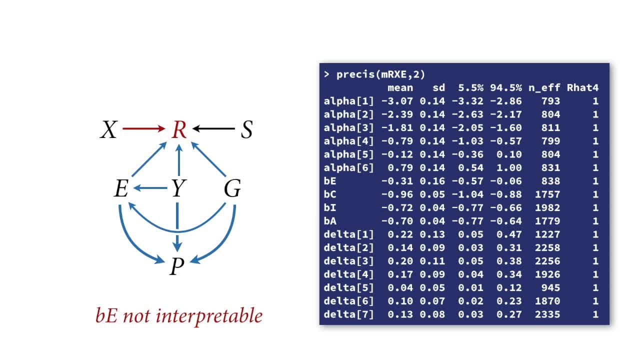 that that's true. and again, as always, if you can't quite figure out why that's true, practice with daggetynet or the daggety package and then look at it yourself again and try to figure out why that's the case. but the intuition is it blocks all the non-causal paths. 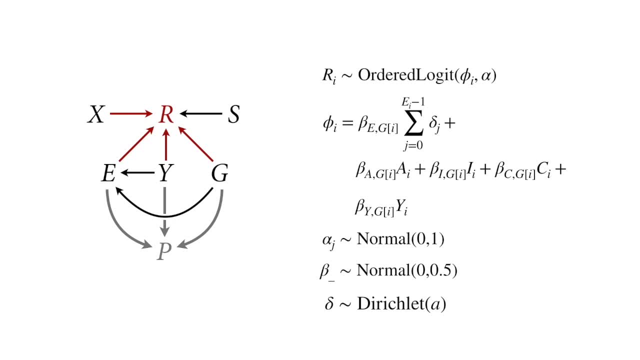 okay. so in order to estimate the direct effect of education, we need to simultaneously stratify the effect of education by age and gender, and here's a model to do it. so on the right, we've got a really big fee linear model component. we'll just take it one step at a time. it'll make sense. 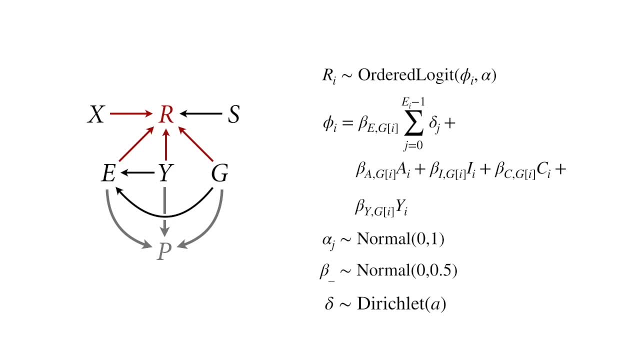 so first we have the ordered monotonic effect of education, but now we're stratifying the maximum effect by gender, so you'll see g of i in the subscript of of beta, sub e, and then we have, as before, the treatments action, intention and condition, and then we have the order monotonic effect of 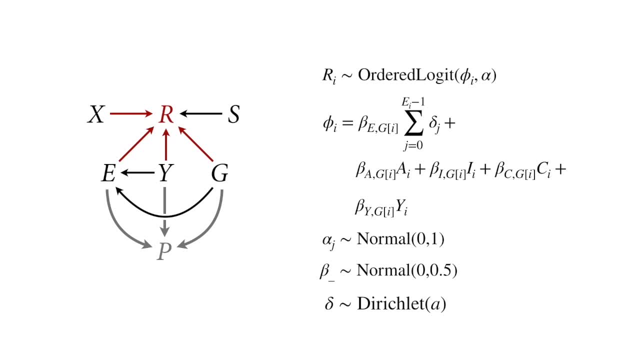 contact, again stratified by gender. we'd already done that and now we've added age and there are lots of things we could do to model age in this model i've just made it a simple linear effect on the log odd scale, on the cumulative log odd scale, although i'm not really satisfied with that. 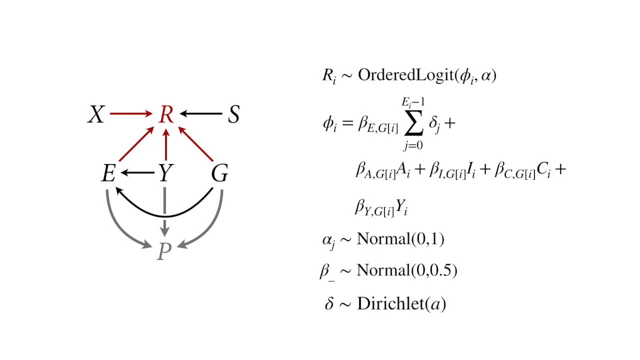 and there are other things that i'd probably try if, if i had a lot more time in this lecture to do it in. we'll talk about modeling things like age more flexibly in a couple of weeks, and then the priors are familiar. these have not changed since the beginning and we still have the 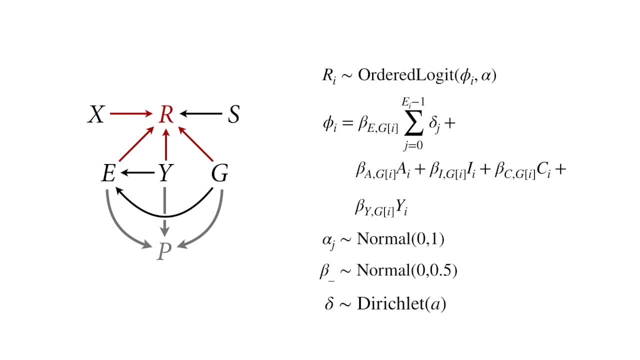 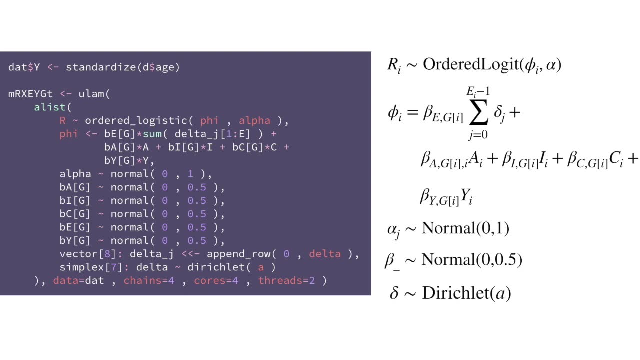 dearie clay prior for the effects of education. setting up the code: you just make a long fee, it's no problem, and you can break it across lines if you need to, so it's easier to read, as i've done here. but otherwise there's no tricks, you've just got a. 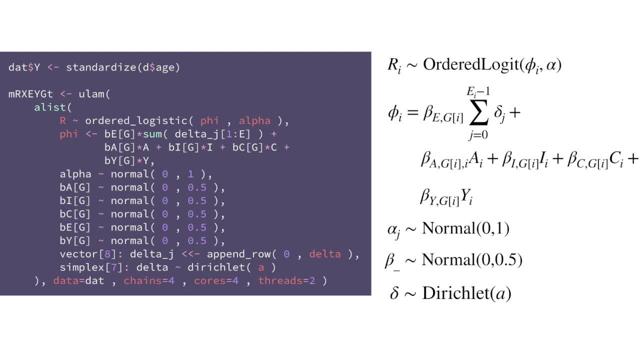 lot of parameters, so you got a lot of priors, but it's it's all the meanings i hope are clear. one thing to note on this is: this is a pretty big model now and one thing you can often do with with ulam models, since they use stan, is you can multi-thread them. so for a lot of models, 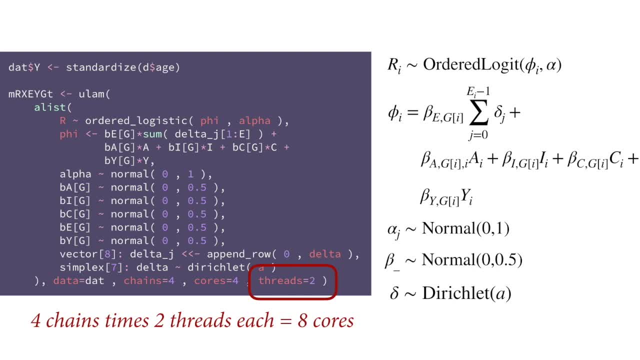 but not all models. if you set threads to a number greater than one- so here i've set the threads argument to two- then each chain will use multiple cores. this is a data set that's really set up to take advantage of this because, as i said, it's almost ten thousand responses, and so if 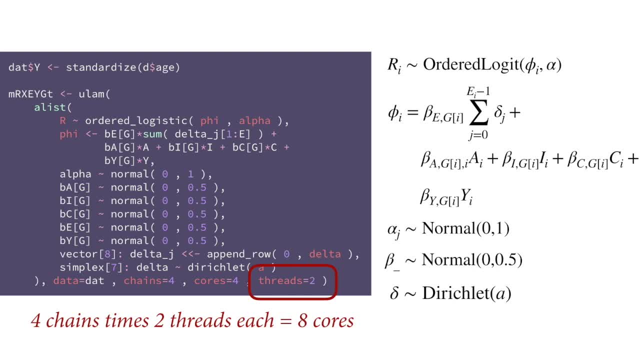 we can take about five thousand of those and send them to one core and the other five thousand to the other core. the cores can take the derivatives, uh some- separately and then put it all back together because it's additive, that is, factor factorizable by each row, not all analysis problems. 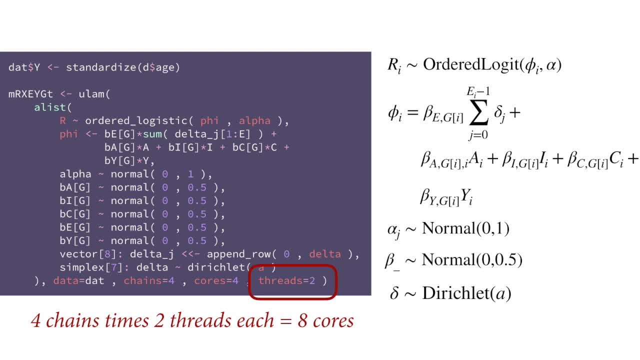 can be factored that way. so you can't always do this, but when you can it can save you a lot of time. so in this case, four chains each uses two threads, that's eight cores total. lots of computers have eight cores these days and my laptop has 12, for some reason. 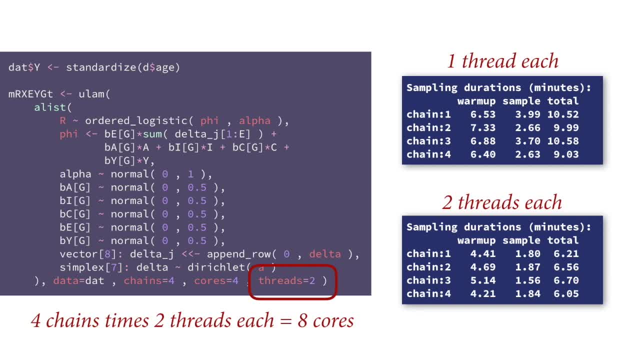 and when you run this. just to give you an idea, this is not that big a model. it doesn't take that long to run, but it's certainly the slowest model so far in this course, and so this model will run with one thread. each chain takes about 10 minutes total. i'll show you in the output in the upper. 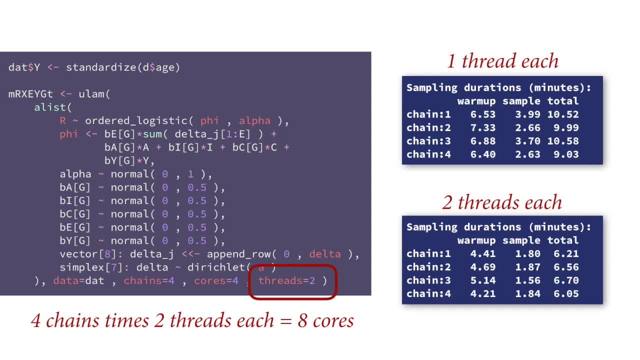 right hand corner of the model. here, with two threads per chain it only takes about between six and seven minutes, less than seven minutes always total. now maybe that's not a big deal- it isn't, but as your models get bigger and bigger that that savings may stay proportionally the same, but in total time it grows real fast and so it can definitely. 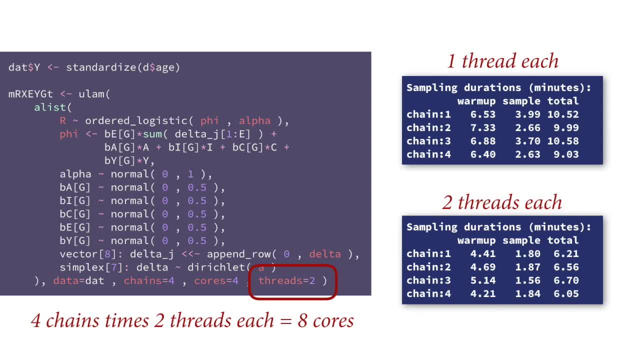 be worth it to use additional threads. many computers these days have lots of separate cores, so you can take advantage of them. i should say that ulam has to make some guesses about how to multi-thread these things, and so this doesn't going to work automatically for any arbitrary. 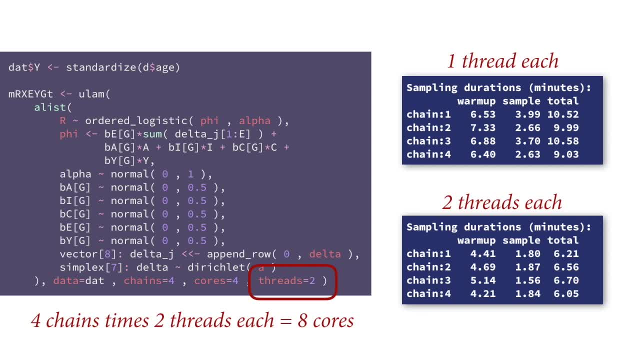 model that you can fit with ulam, but it'll work for lots of glms and that's the way i've written it. if you learn to write stan code directly, you'll have a lot more flexibility and learn a lot more about when you can make this work and optimize it in additional ways. 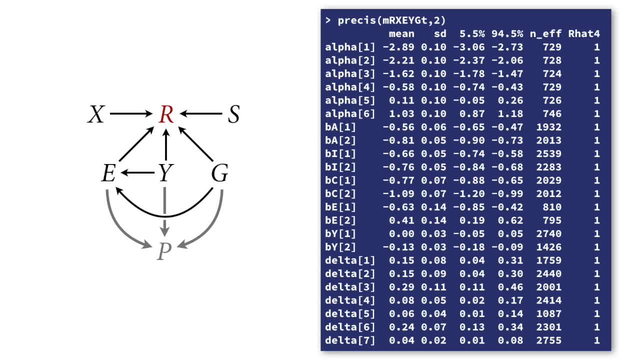 okay, so that model runs six and a half minutes of time well spent. we look at the pricey output here for this model, or poetically called model m, r, x, e, y, g, t, that is. i say it's a model of the response r that includes as predictors x, e, y and g and the little t for threaded. and i'm just showing you all these. 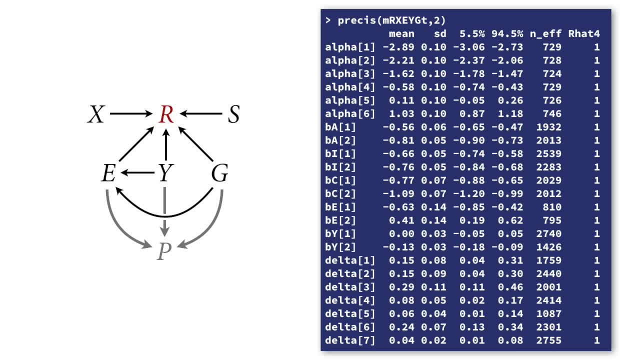 parameters. i don't like to interpret parameters, as i keep saying, but there's some stuff that's useful to point out by taking a tour through this table. so so let me do that. the first is, if we look at the treatment effects stratified by gender, keep in mind that this is only the direct effect of gender. 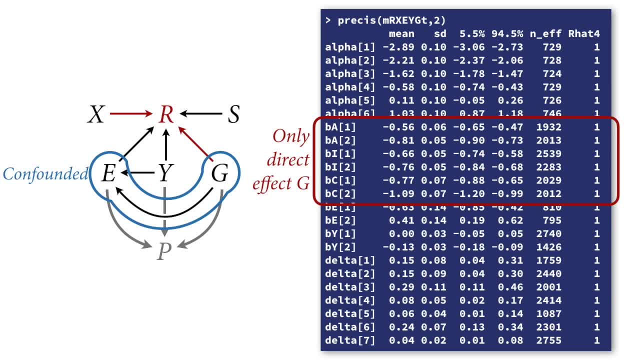 yeah, we haven't estimated the total causal effect of gender and in fact we cannot. i'll say that again: these coefficients are only the direct effect of gender, estimates of because we we stratified by and age, and when we stratify by education, we block the indirect path of gender. and if we 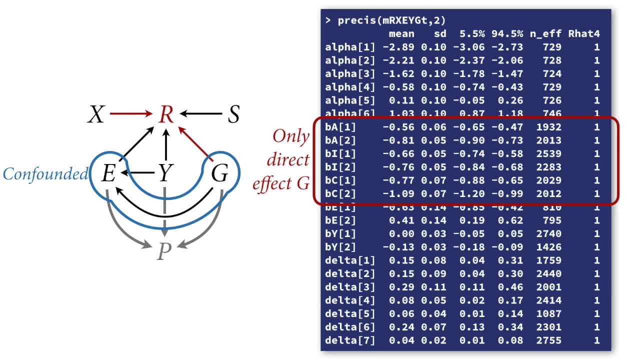 didn't stratify by education, the estimate would be confounded by the sample selection by participation, p, and so in this case we cannot estimate the total causal effect of gender in an unconfounded way, but we can, if this tag is correct, get the direct effect. and that's not nothing, that's something. and 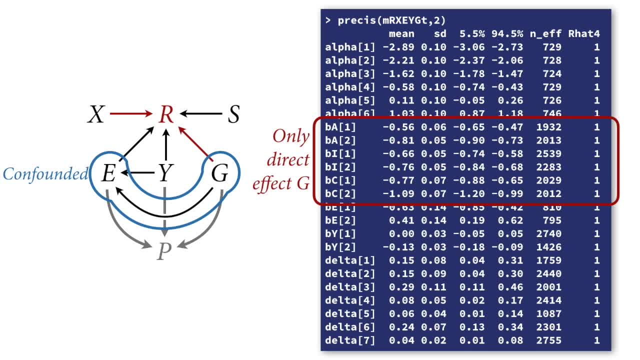 what you see here is that there are- uh, there there do appear to be reliable differences for some of the treatments, but in general, the pattern is very similar. where action and intent are less bothersome to people than contact, then we have education effects, and this is what we were after all along, and this is the 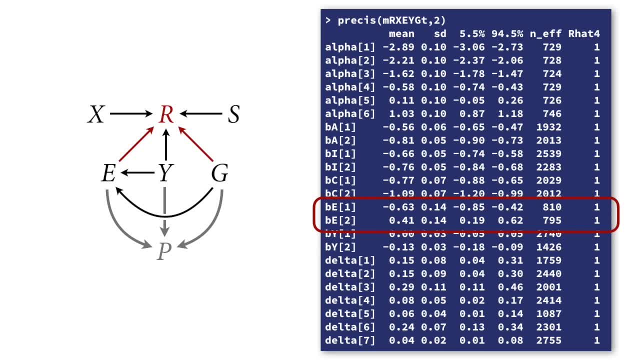 direct, effective education stratified by gender, and what i want you to see now is that it's opposite directions- uh, for women and men in the sample. according to this, this model, so beta e1 is the coefficient for women, and so this says that more educated women in the sample. 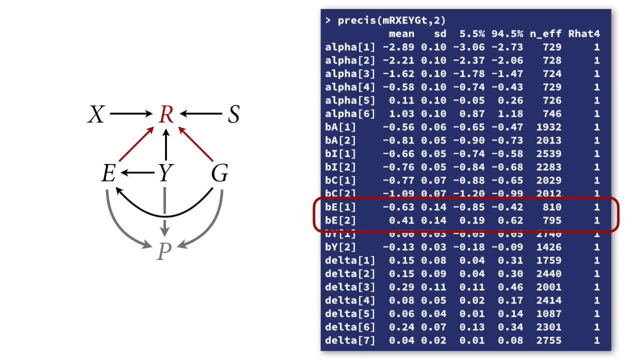 tended to give lower ratings to the same stories that more educated men gave higher ratings to. yeah, you see that in direction of the coefficients. so this is an interesting thing that we didn't see when we only had the average effect that was not stratified by gender. 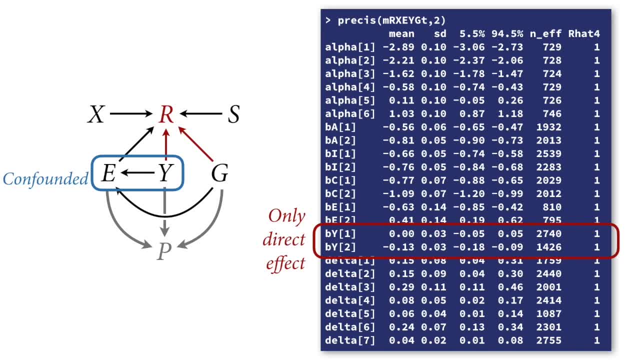 age. age like gender. here we're only getting the direct effect and we cannot estimate the total causal effect of age. part of the causal effect of age, according to this dag, goes through education, as shown in the image, and that is confounded by sample selection by patient p in this. so but we do get the direct effect here because we've stratified by education. 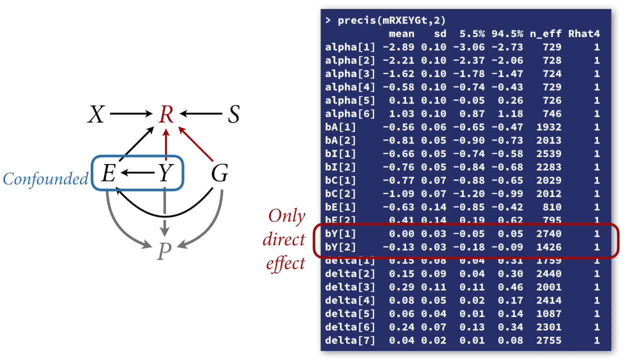 that blocks that indirect path and it also blocks the confounding. and we can get the direct effect, but we cannot get the total effective age. one of the things that this stops us from doing actually with this model, in these data, is that we cannot say what the causal effect of age is in total. 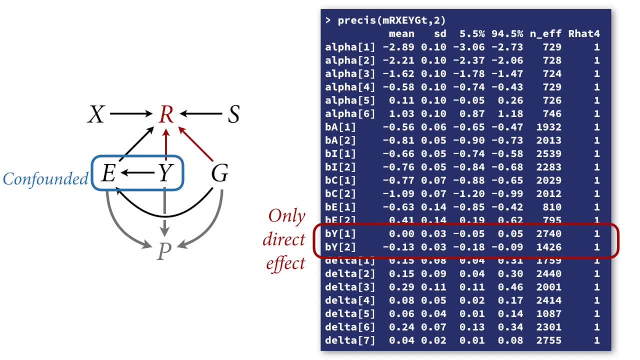 yeah, if you imagine an aging population and how their judgments of these stories might change, that's something we will need additional information on for from outside the sample, in order to estimate the causal effect of. because what do we need? we need the causal effect of age on education, which is always confounded in this data, in these samples. 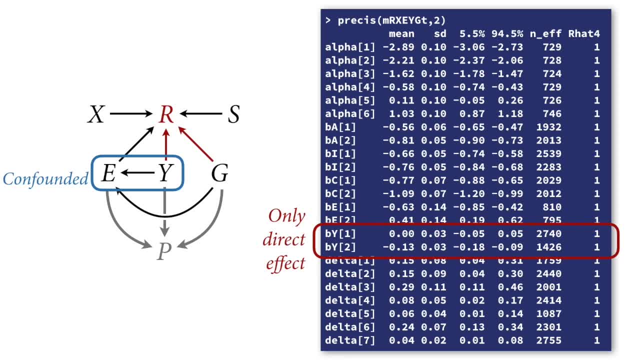 because p effectively effectively acts like a confounder of of the influence of y on e. finally, there are all these deltas. since we found that beta e is in opposite signs for the two genders in the sample, to run a version of this model where there are two delta vectors as well, to see if those are. 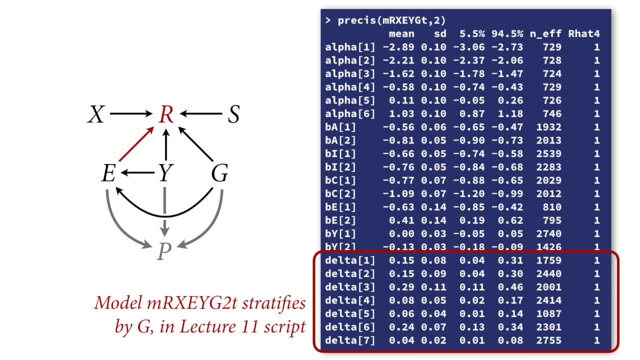 radically different and i'm not going to show you that model in the lecture for the sake of time, but in the script that goes along with this lecture, lecture 11, i'll show you that model so you can see how to specify it and you can pull up the coefficients and look. 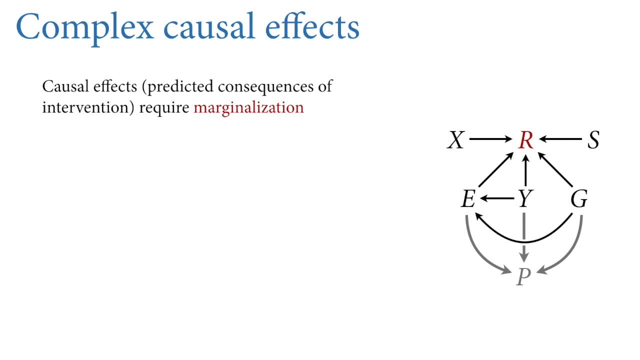 okay, it's often true in realistic data analysis situations that the causal effects of interest are actually very complicated and they're not well summarized by the coefficients that come out of the model. and i know i've said that before, but this is a new level of complexity. 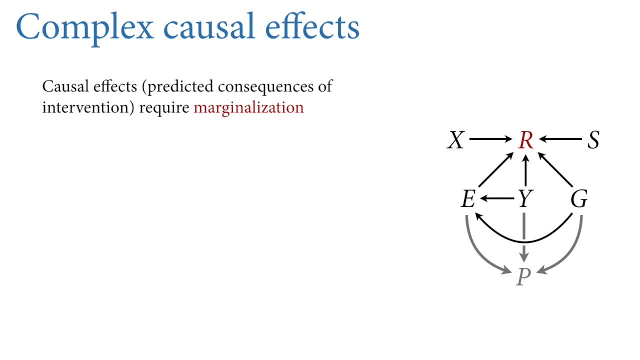 but if the complexity comes from the science and not from the statistics, the statistics are just the coefficients, and the problem is that the coefficients in non-linear models hardly ever tell us about the counterfactuals of interest. so remember usually what we're after as researchers. 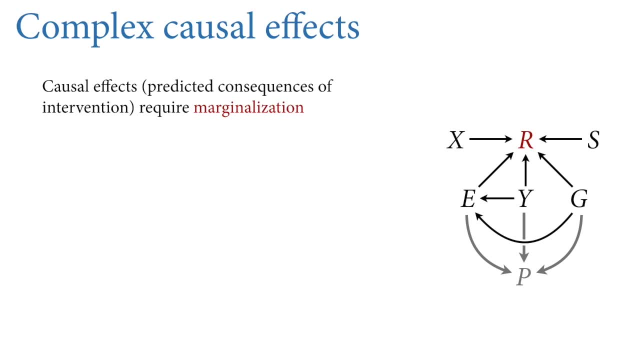 is the ability to predict the consequence of some hypothetical intervention or actual intervention. if you're in the applied sciences, and this requires marginalization, it requires averaging over values of the other predictors, the ones that you're not intervening on. some of those may be influenced by your intervention, but even if the other and you 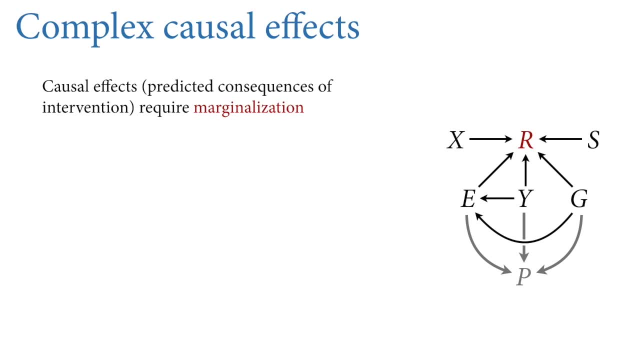 definitely need to average over those, simulate their values as influenced by your intervention, but even the other ones. you have to make some decision about what the target population is and how you're going to do this. let's think of some examples. suppose we want the causal effect of education. well, in order to calculate that for any particular 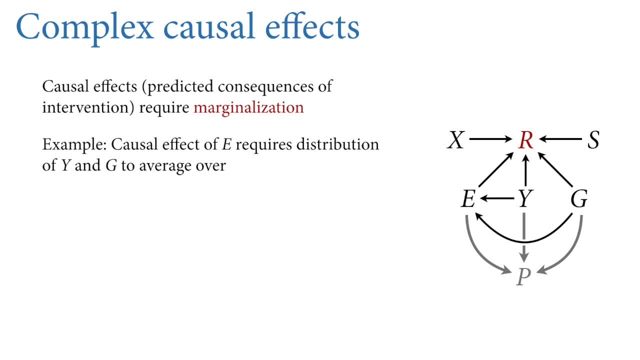 target population. we're going to have to put in some distribution of ages and the genders in the population to average over, because the effective education, the effect of education, will vary on depending on that, even if there's no explicit dependency between those effects in the linear model, because this is a non-linear model, and in a non-linear model- remember if anyone 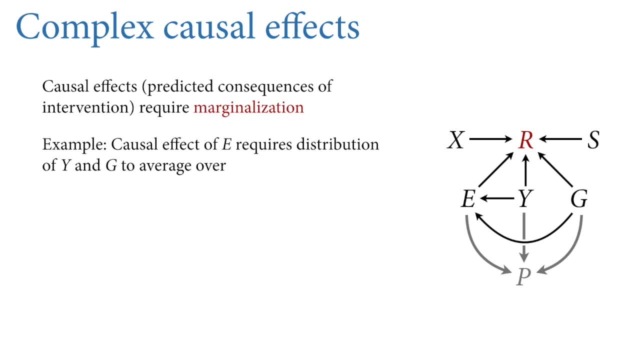 effect pushes the expectation high towards the ceiling or low towards the floor of the outcome space, then necessarily every predictor moderates every other predictor, and so this marginalization step is not optional. you really have to do it to do it right. um so, uh, there's some problems. 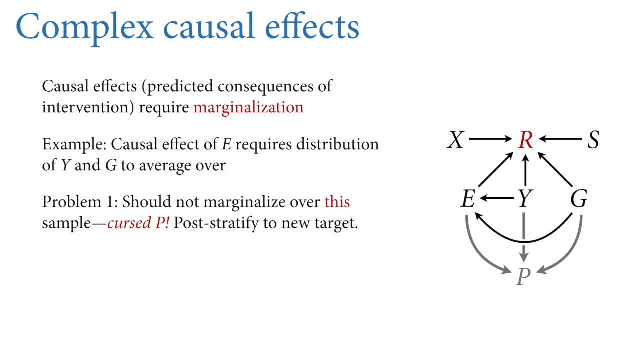 in this particular example. uh, in addition, we can't use the sample distribution of ages and genders for this marginalization if we're going to going to calculate the causal effect of education here, because this sample is in effect cursed by voluntary participation by the p variable, the. 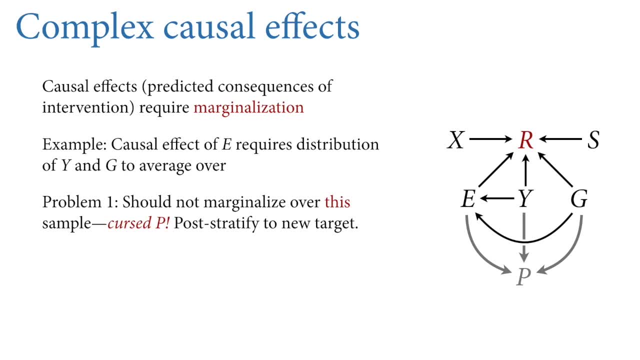 age distribution and the gender distribution are just a feature of this sample. they're not a feature of any population we care about. so we need to use external demographic information to choose a distribution of y and g that we'd like to use to calculate some hypothetical factors in order to calculate the causal effect of education. the other complication with a causal 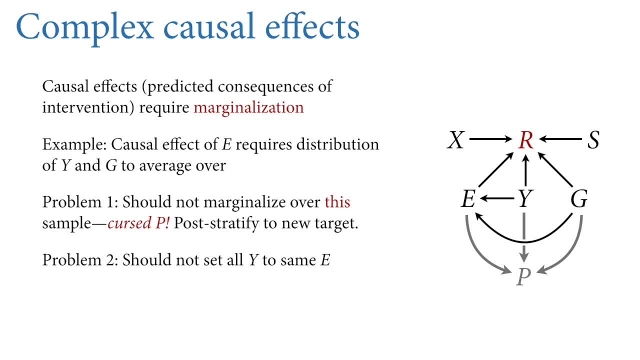 effect of education. this example is: it doesn't make any sense to set everybody's education to the same value, because there is necessarily a very strong causal relationship between age and education. you can't create 10 year olds with phds. that is not a plausible, that's not a possible. 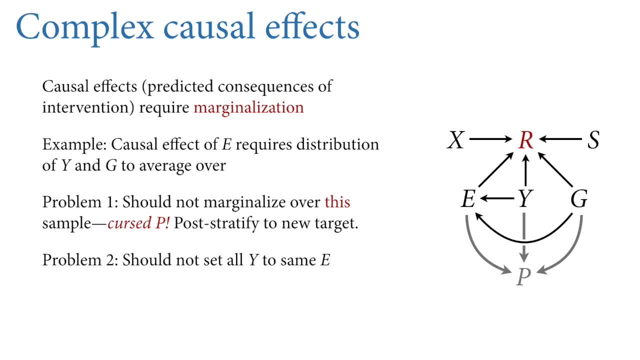 intervention. so you have to think in a much more subtle way about what sorts of interventions are realistic that you'd actually want to calculate some some expected causal effect for and that could be accelerating at a particular grade. it could be accelerating college, and then that will necessarily affect some age groups more than others. 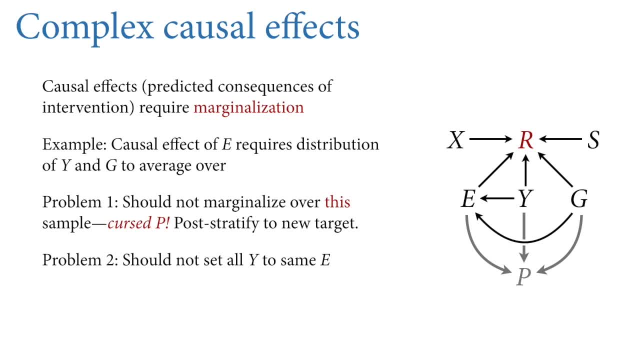 and i know this sounds complicated, but it's just complication that arises because of the causal structure of the scientific problem. it's not inherently a statistical problem, it's a scientific problem and that means you can control it because you have scientific knowledge about your problems. if you don't study moral psychology and trolley problems, 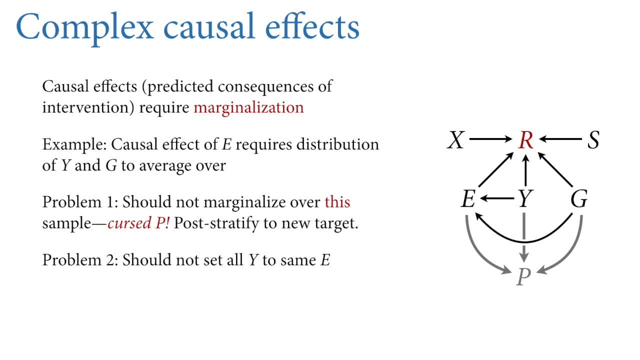 this may seem more confusing than it would actually be if you were working in your own context, where you understand the scientific background and these tasks become much easier in that case, believe me. so another example: say we want the causal effect of age. well, getting the causal effect of age. 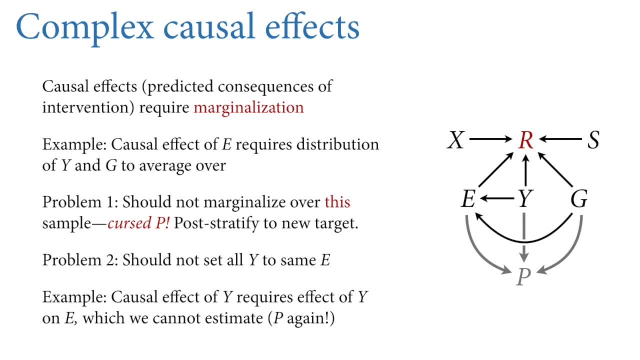 requires knowing the direct effect of age on education. as i just said, there's a strong relationship and it is a strong relationship and it is a strong relationship because it's a strong relationship and it is causal and but we can't estimate that with this sample, and so if we'd like, 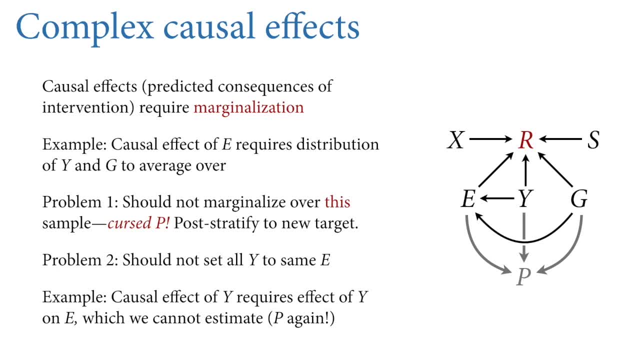 to compute a marginal causal effect of age- how, how, and that would mean how do people's judgments change with age? then we need to get some estimate of the causal effect of age on education from somewhere else outside this sample, and if we could do that, then we can do that, then we can. 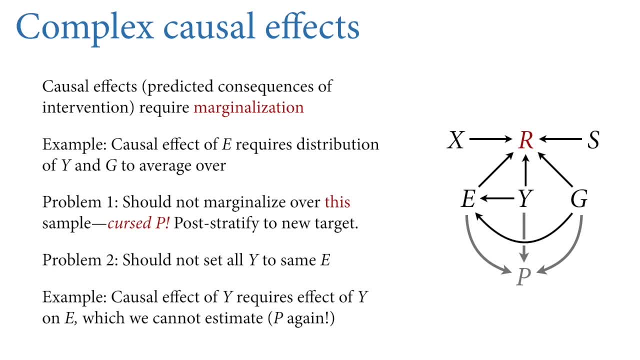 get the causal effect, and that is possible, right, because you can get information from the scientific department about the target population and the rates at which people gain education as they age, and that's all that causal effect means, and then you can complete the calculation. okay, this is. 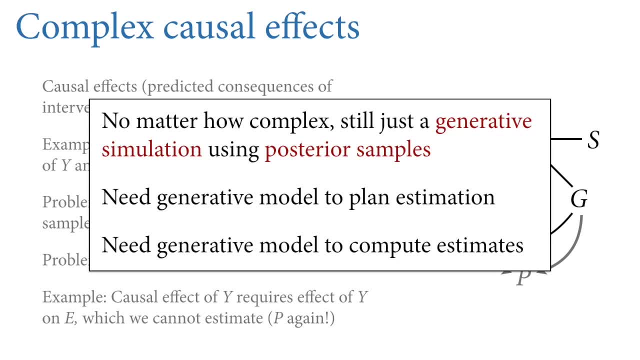 complicated because it's just reality and that's what it is. but the good news is, once you understand the structure of this, the algorithm is always the same. it's just that we're going to use a generative simulation using posterior samples. that's all. these causal counterfactuals are if you've got. 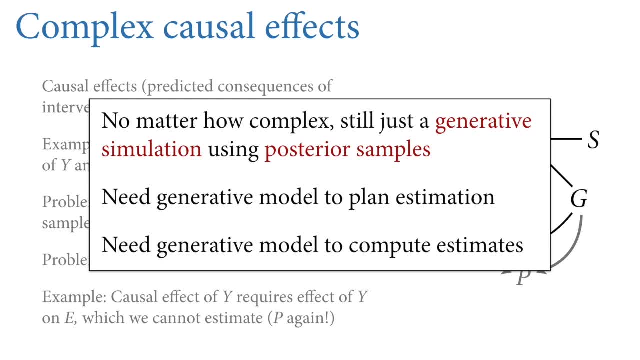 the generative model. You can use the posterior samples to simulate a range of scenarios, each conforming to whichever causal intervention you're interested in. So we need a generative model to plan the estimation. We need the DAG and functions to embed in it just to plan the statistical estimation strategy. 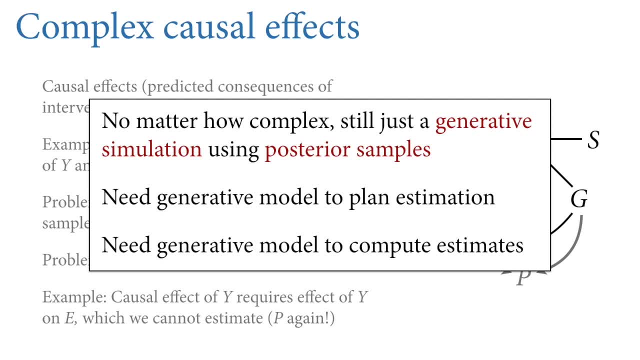 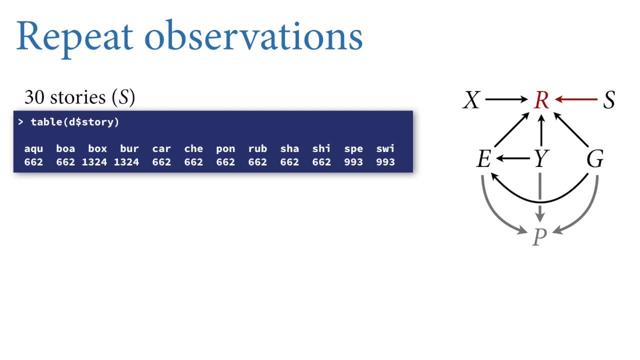 But then we also need the generative model to compute the estimates, that is, the causal estimates. Okay, this has been a long lecture. There's one thing to say that will bridge us to the next. In this dataset, there are some variables we have not dealt with yet and we probably should. 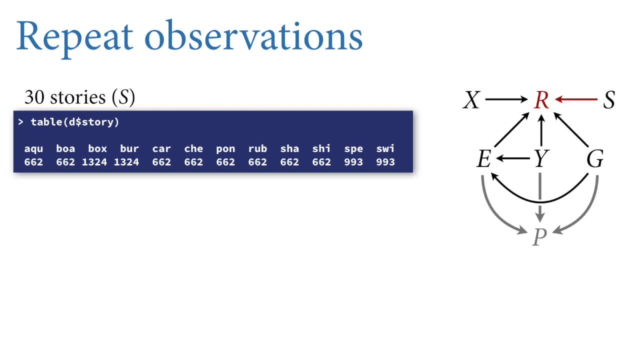 And these are competing causes. So the first are the 30 different stories. These are the trolley stories that the researchers added and subtracted action, intent and contact to. There are 30 of them and they're repeated hundreds of times in the dataset. 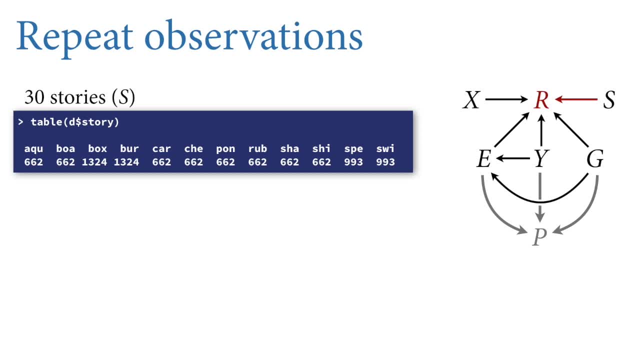 And these stories possibly, quite probably, have been repeated hundreds of times in the dataset. And these stories possibly, quite probably, have been repeated hundreds of times in the dataset And these stories, possibly, quite probably features about them which also affect people's judgments, features other than action intention. 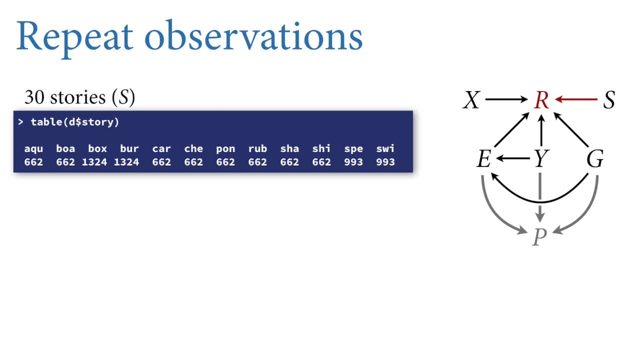 and contact, and we haven't coded those features because we don't know what they are necessarily. but we can statistically estimate if each of these stories induces higher or lower responses, and so we'd want to do that as well. all i'm showing you on the screen here is the frequency. 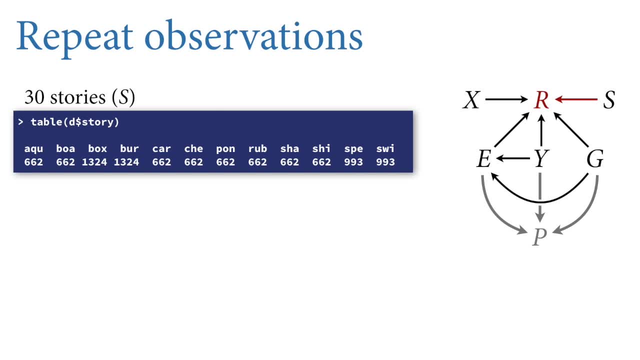 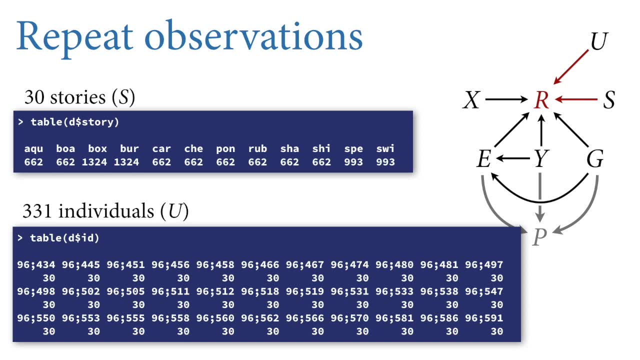 table for the different 30 different stories, and you see that some of them are much more common than others, and then there are also. there's another variable which i'm just going to add to the dag now and i'm going to call it you, and these are features of the individuals which we 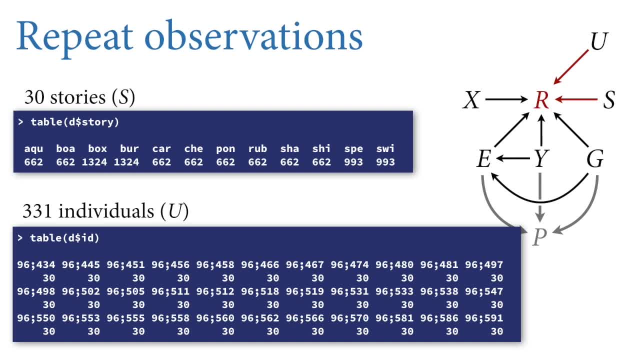 have not observed. there are 331 individuals in the data set and each of them have contributed 30 responses, and we can do the same thing with the individuals. we can do with the stories. individuals may have particular attitudes and experiences and moral theories which influence how they respond to this task. 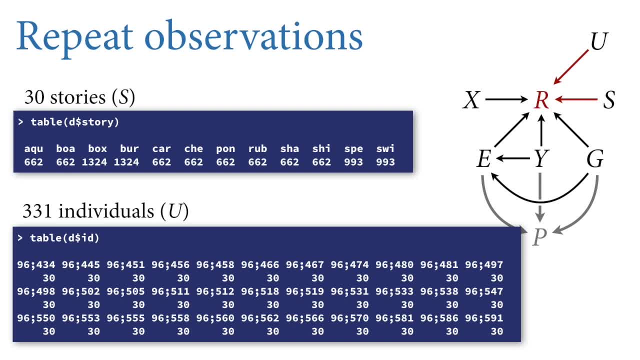 and some individuals are taking it more seriously than others, some less, and we don't have measurements about those things. but we do know the identities of each individual, or rather we can tie each response to a unique individual, and so, statistically, we could try to estimate these? u values as well. however, there are 331 of these parameters to estimate and only 30 data. 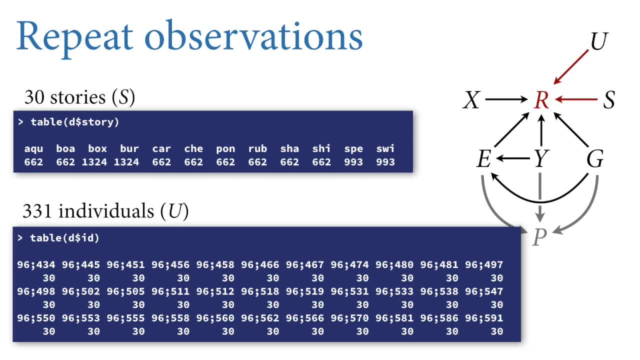 points would to estimate each one, and this opens up a big area in statistics where we can think about the choices we have in trying to efficiently estimate a large number of parameters with a small amount of data for each, and it turns out there's some clever stuff to learn here, and that's what we're. 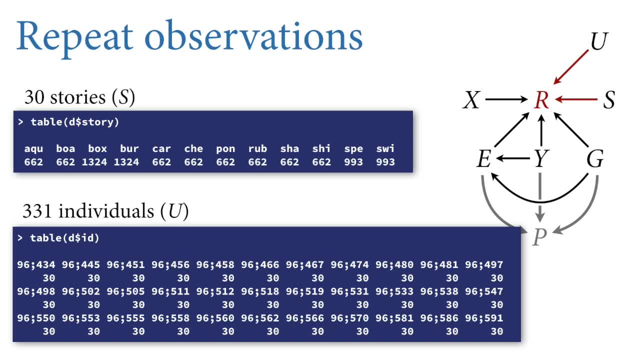 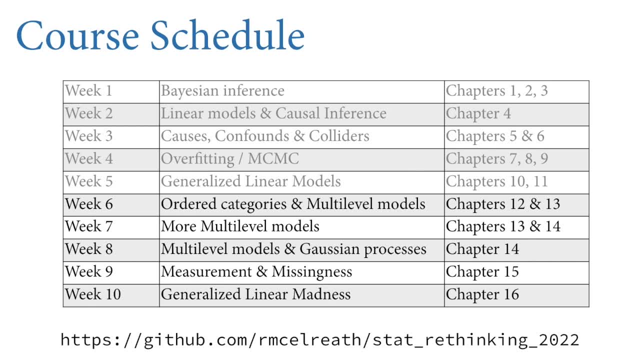 going to start looking at in the next lecture when i introduce you to multi-level models. okay, that has been lecture 11. we're in week six. in the next lecture, we'll introduce you to multi-level models and we'll have a bit of a marathon of multi-level models where all of 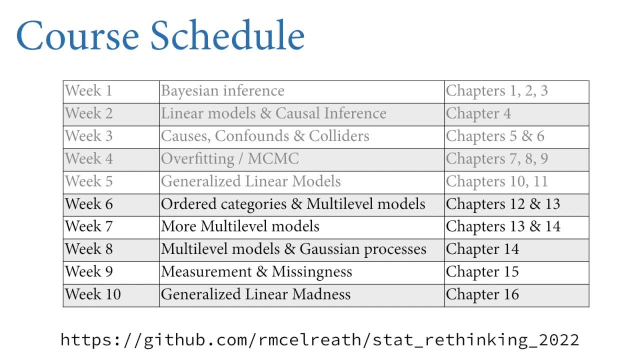 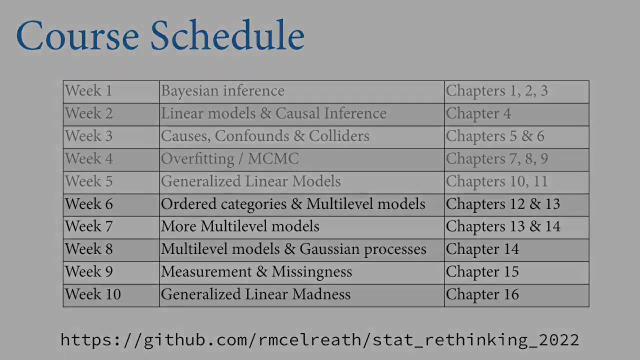 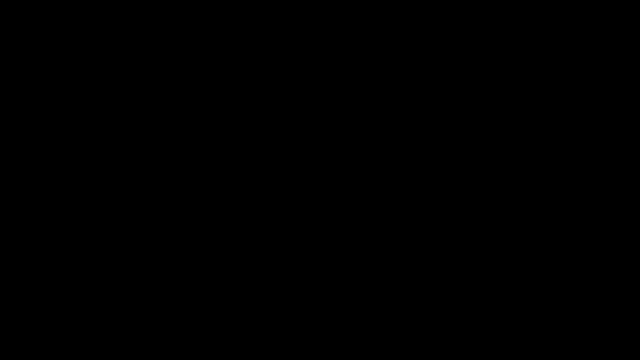 next week will also be multi-level models, and then in the beginning of week eight, and gaussian processes and week eight are also a kind of multi-level model. i've spread the material out so it goes slow, and in the next lecture we'll just do the basics and i'll see you there.